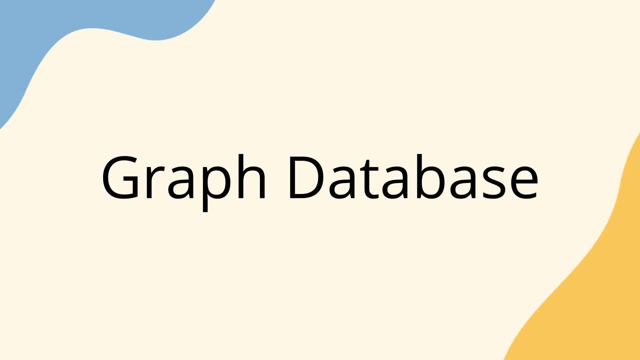 applications data. So, for example, let's say: well, we own Twitter, Twitter is our application. We need a place to store the tweets, We need a place to store the pictures, the accounts, etc. And of course, we're going to do that inside of a database. So, inside of our database, we're going to store our 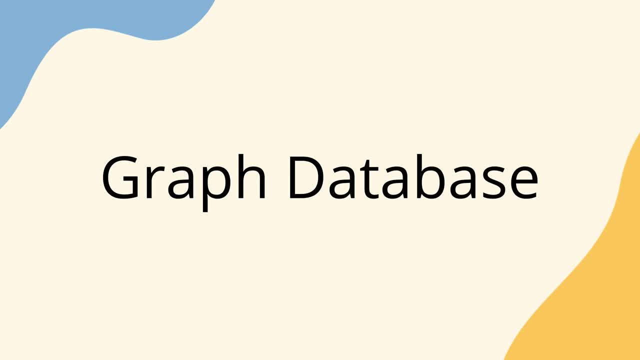 data. We're going to also retrieve data from our database. We're going to update data, We're going to delete data and we're also going to create data inside of our database. Now, what is a graph database? Well, in the database community, we have hundreds, if not thousands, of different databases that we can 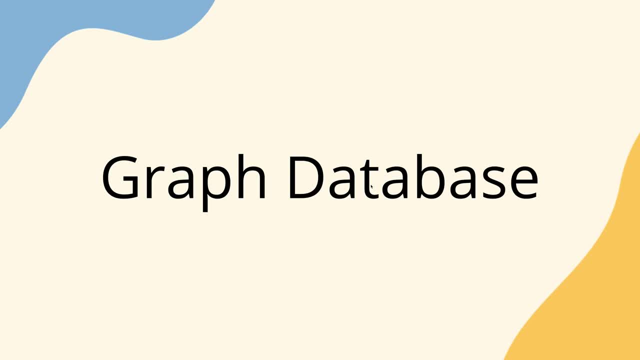 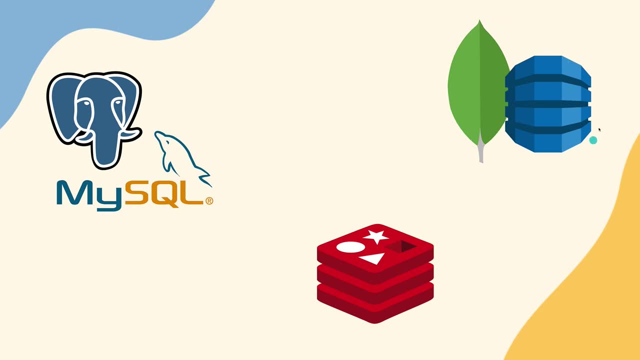 utilize And there's different types of databases. For example, over here for Postgres and SQL, we have SQL databases. Over here we have document databases such as MongoDB and DynamoDB, And here we have key value pair databases like Redis And each database, even though they are storing data, our 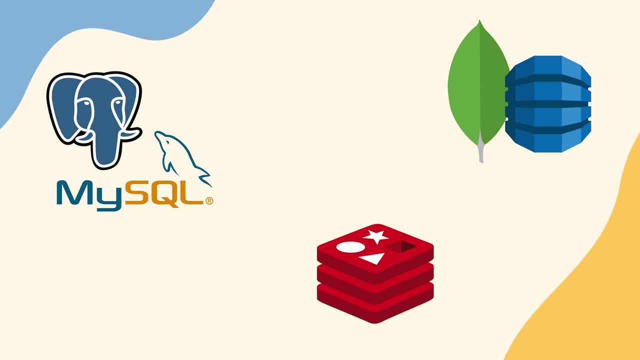 applications data. the way that they store data is by the way that they store data. So we're going to do some more of that in a little bit, But what I'm going to give you today is going to be a little bit more of a general summary for the first two deductions. This is a nice, great statement to 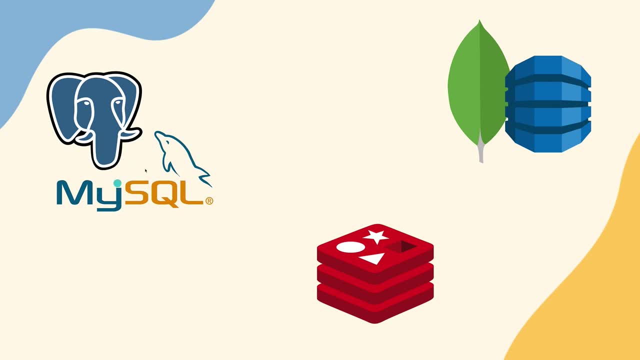 build upon. So let's start off with the first one. The first one is a really useful one that we need to understand. The key value pair database is a database that stores data in a very specific scheme. It's a very complex and very complex schema that allows you to store data: The key value pair. 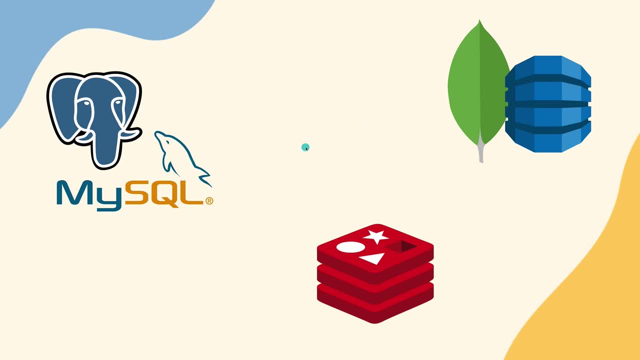 database is a database that stores data in all its different components. So by defining it by each component, you actually store this data in multiple parts of the table. For example, SQL databases store their data in tables even though they are very strict schemas, Whereas document databases 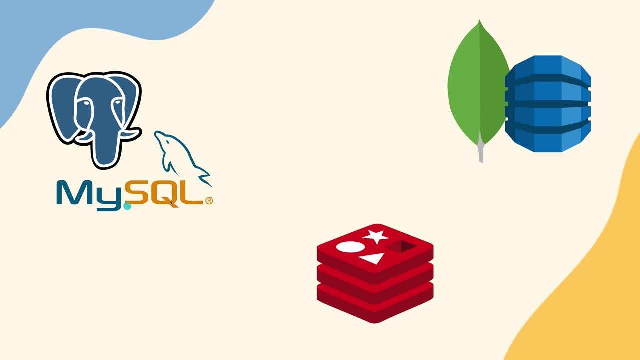 For example, if you want to cache your data somewhere, you're probably not going to use a SQL database to do that. Instead, you're going to use a very quick key value pair database If you want to store very sensitive data and you need to make sure that the scheme is correct. 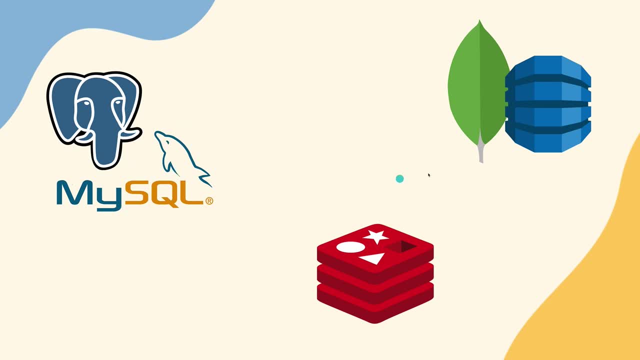 well, you're probably going to want to use a SQL database for this. So what does this have to do with graph databases? Well, graph databases are a different type of databases And they're databases that are used when our application has a lot of relationships. 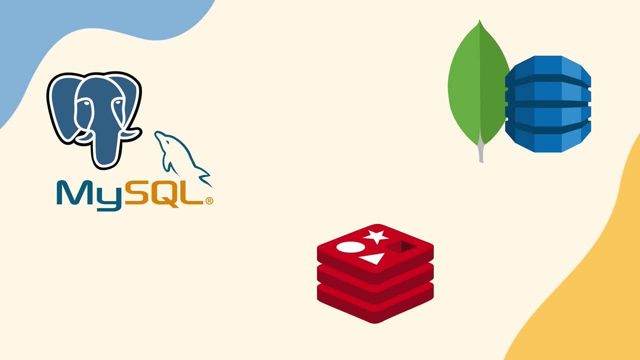 And Twitter is actually a great example of this. So we can have Twitter, we can have a tweet, and then people can actually like that tweet. So we have a relationship between the user that liked that tweet and that tweet, And also that tweet belongs to a specific account, so we have that relationship as well. 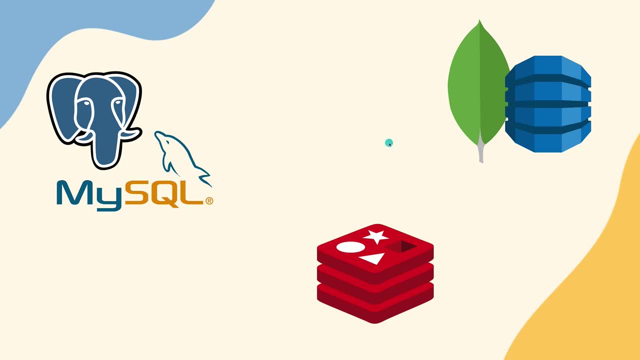 So there's so many different relationships. Now, of course, we can use- We can utilize SQL databases or even NoSQL databases for these types of relationships, But sometimes the relationships are so cumbersome that we might want to use a different database that really focus on storing data as well as their relationships. 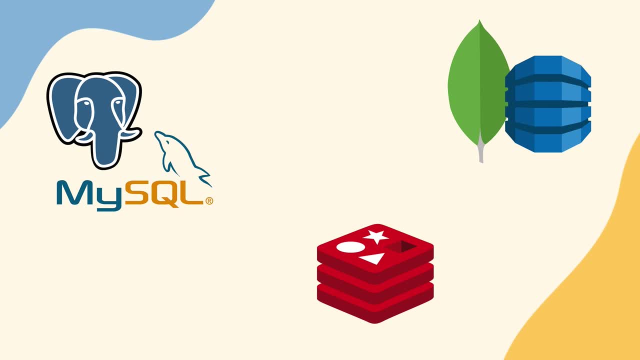 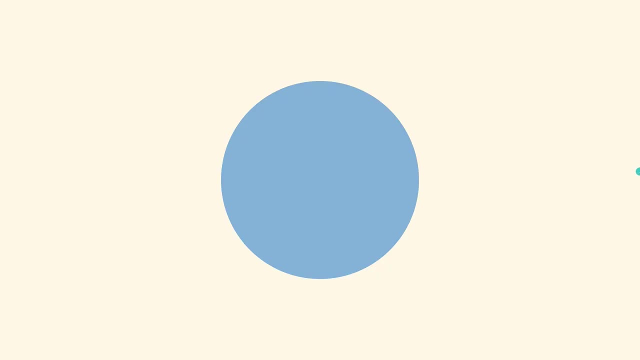 And that is what graph databases are for, And that is exactly what Neo4j is going to do. So now that we understand what a graph database is, let's actually look at how data is stored inside inside of a graph database. Inside of graph databases, things are stored inside of something called nodes. 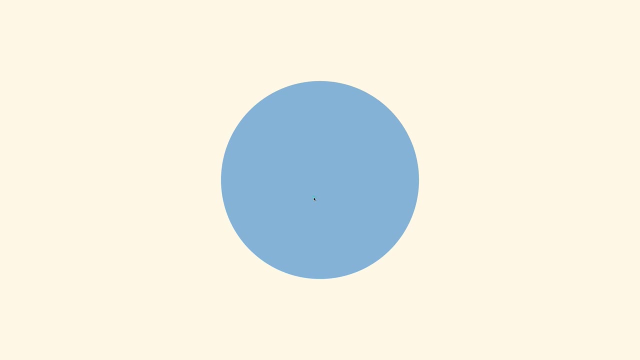 And over here we have this circle that is representative of a node, And inside of that node we can have any one thing. Now you might be thinking: what is this thing? Well, this thing can be anything that we define. This could be a food item. 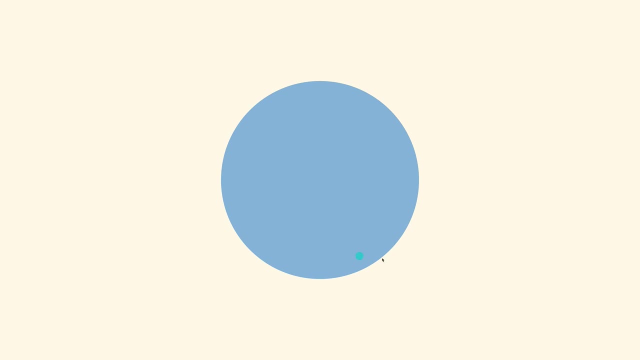 This could be a laptop, This could be a building, This could be a person, But again, we're going to store that thing inside of that node. For example, let's say, that thing is an NBA player, Then what we would do is we would store, well, let's say, LeBron inside of this node. 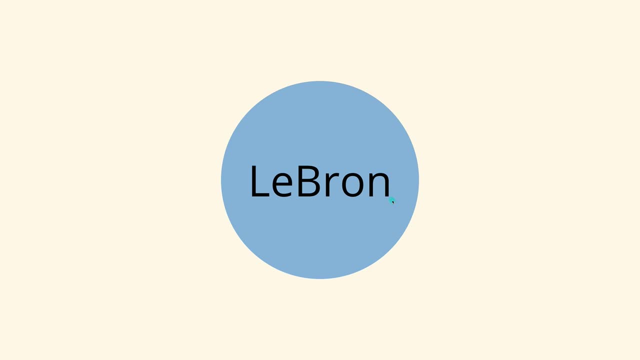 So we would store it inside of this node. And now if we wanted to store multiple NBA players, then what we would do is we would have multiple nodes and we would store those NBA players in those nodes. So over here we have LeBron Anthony Davis, Russell Westbrook, James Harden and Kevin Durant. 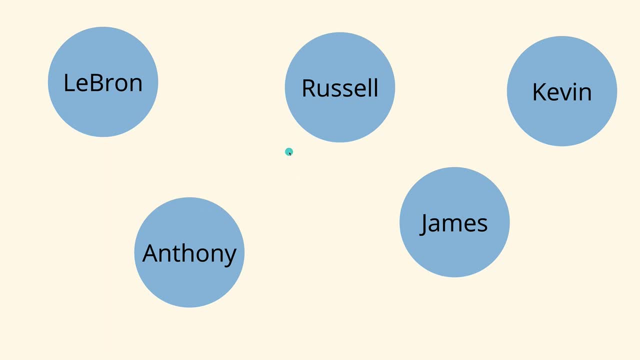 Obviously, you don't have to know them, but if you watch this channel, I always have basketball everywhere. You guys probably know I'm a huge basketball fan. But again, those things which are NBA players are stored inside of nodes. So that is how things are stored inside of graph databases. 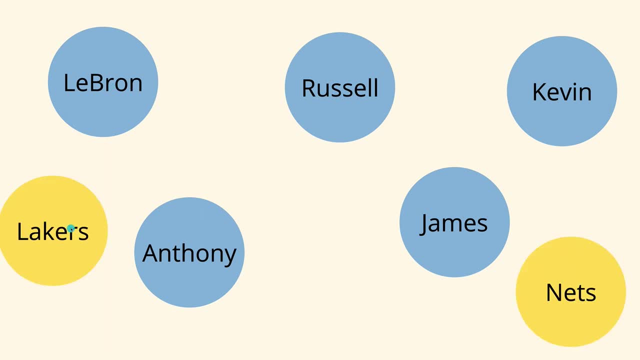 Now, of course, we can also store multiple things. So over here we can have a node that is storing the team, the team Los Angeles Lakers. Over here we can also have another node that is storing the team. Over here we can also have another node that is storing the team Los Angeles Lakers. 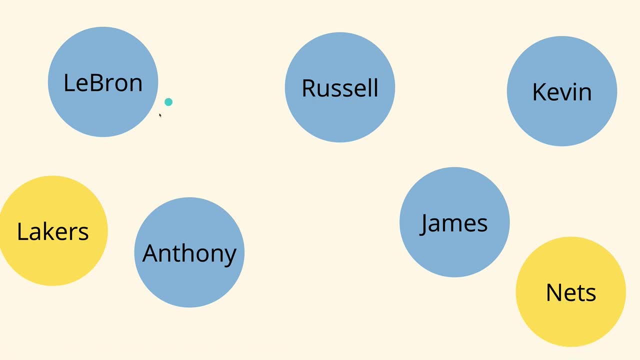 storing the team Brooklyn nets. So we can store multiple things. they don't all have to be, you know, players. we can have players, we can have teams, we can have coaches, etc. we can have a bunch of different things. Now, the special part about graph databases is that we are going to be 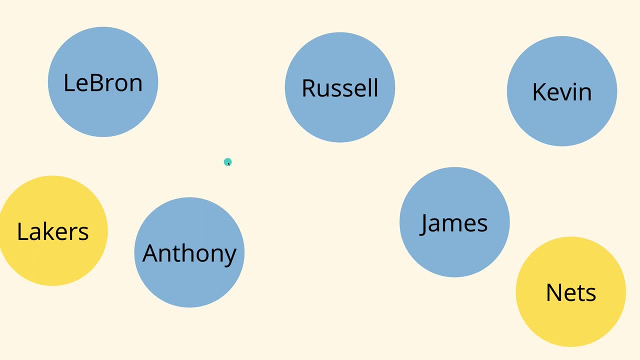 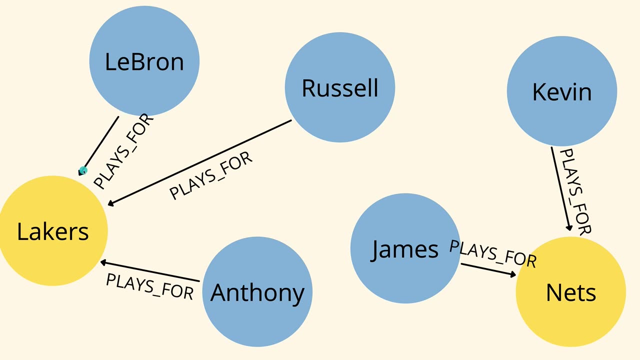 able to relate these nodes together. So, for example, over here we have this node and then we have this relationship. So we have this relationship. So this node, LeBron James has this relationship with this other node, Los Angeles Lakers. And what is this relationship? 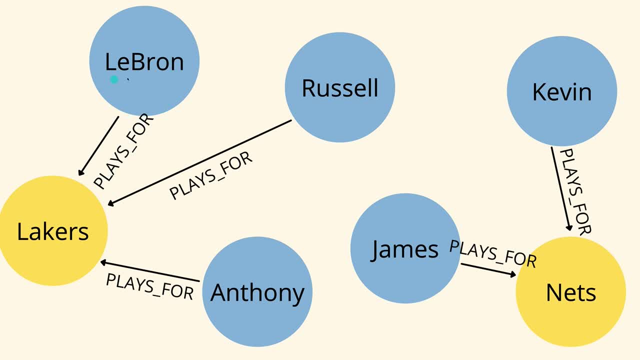 Well, this relationship is plays for. So LeBron plays for the Los Angeles Lakers. And notice that this relationship is directional and it's only one direction. it's only moving in one direction, LeBron. he plays for the Los Angeles Lakers, not the Lakers plays for LeBron James. 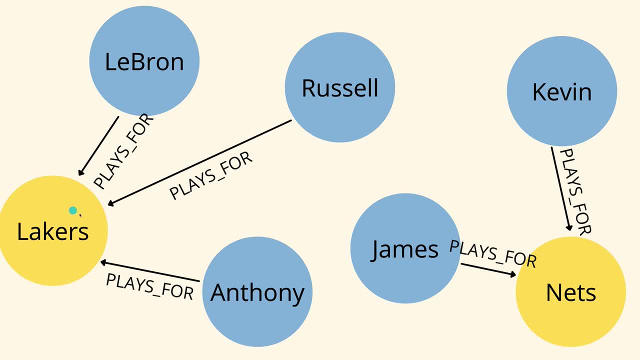 Similarly, over here we have Russell Westbrook: he plays for the Los Angeles Lakers. And over here we also have Anthony Davis: he plays for the Los Angeles Lakers. So over here we can also define these relationships. And over here we have Kevin Durant and James Harden: they play for the Brooklyn. 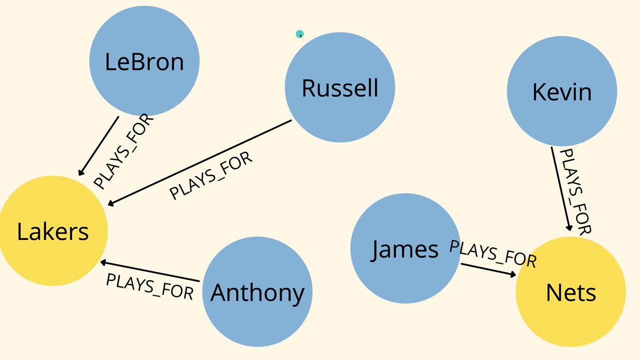 nets And of course, we can have multiple different types of relationships. For example, we can also have: LeBron James is a teammate to Russell Westbrook. Russell Westbrook is also a teammate to LeBron James, So we can also have: LeBron James is a teammate to Russell Westbrook, So we can also. 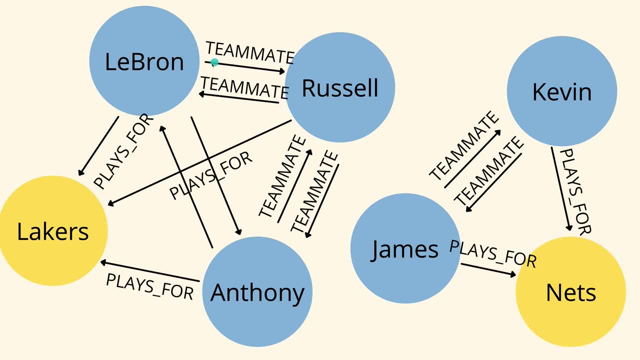 have LeBron James, So we can also have LeBron James. Now notice that this is going two ways, But these are two separate relationships, So this is going one way and then this is going the other way, And then over here we have. you guys probably get the point. Russell Westbrook is a teammate to. 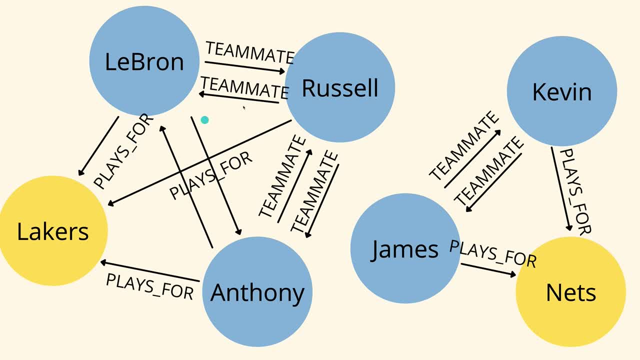 Anthony Davis. Anthony Davis is a teammate to Russell Westbrook. So you can see, here we can actually have a bunch of these relationships across these different nodes And if you're familiar with data structures, this awfully looks like a graph data structure where we have nodes. 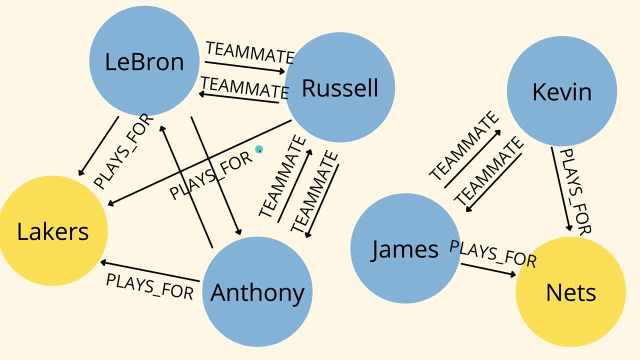 that are attached to a bunch of other nodes, And then over here we have a graph data structure where we have nodes that are attached to a bunch of other nodes, and then over here we have nodes that edges. And that's exactly why it's called a graph database, because it simulates the graph data. 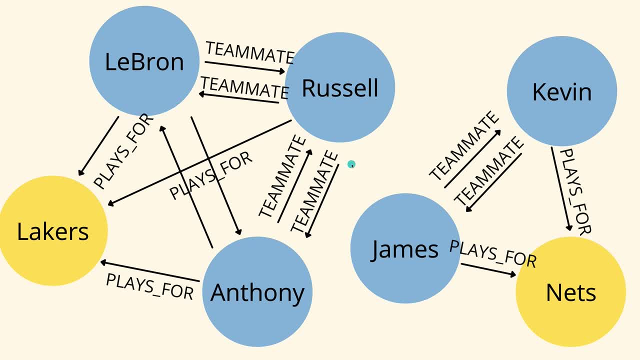 structure And that, again, is how data is stored in Neo4j, which is a graph database, And this is going to make you know when we have applications that are heavily related, there's data that are heavily related. it's going to make querying for that data, adding that data, retrieving that data. 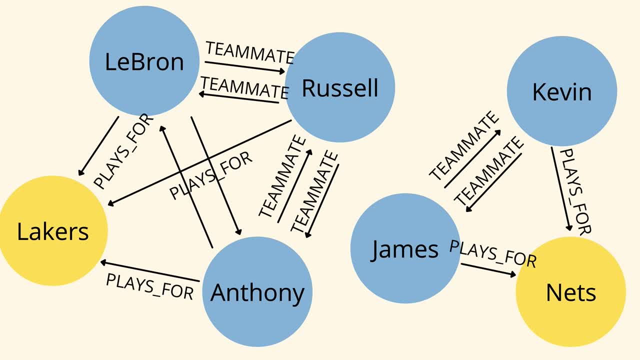 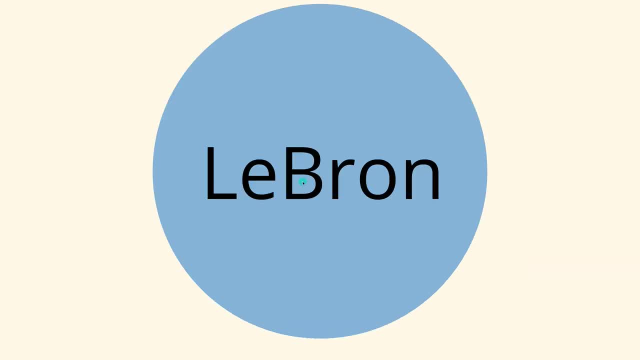 deleting that data a lot simpler than maybe dealing with a traditional SQL database. Okay, cool. So I got one question for myself right now. So over here we have this node. how do we know that this node has you know? how do we know that this node belongs to LeBron James? Well, 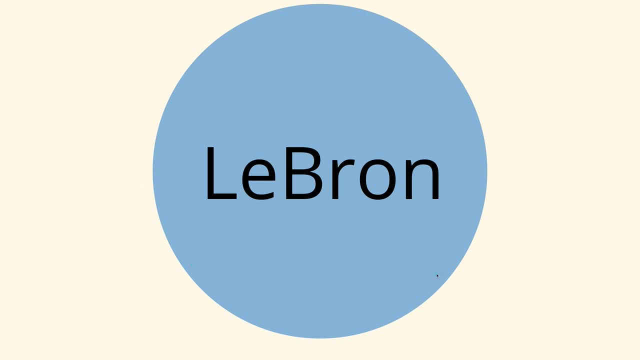 each node, we can actually put different properties inside of it And really it's not going to look like this. it's going to look something like this: So over here we have a node, And then over here we have different properties. 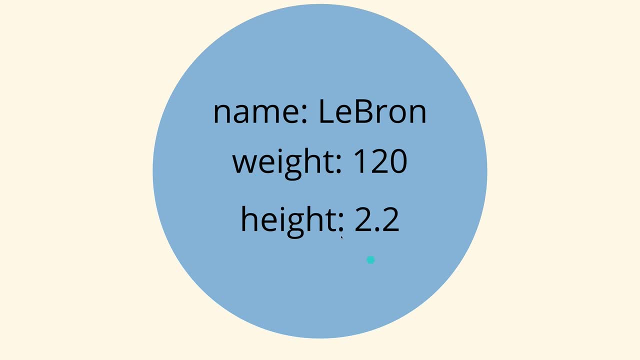 we have the name LeBron And we can also have multiple different properties. it doesn't just have to be the name. we can have the weight, which is, you know, 120 kilograms, the height, which is 2.2 meters. So we can have different types of properties inside of our node, And that's how. 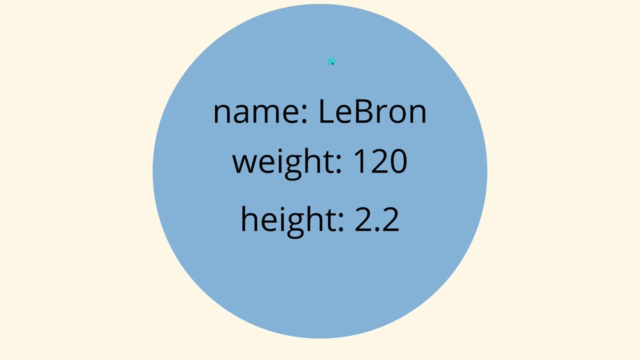 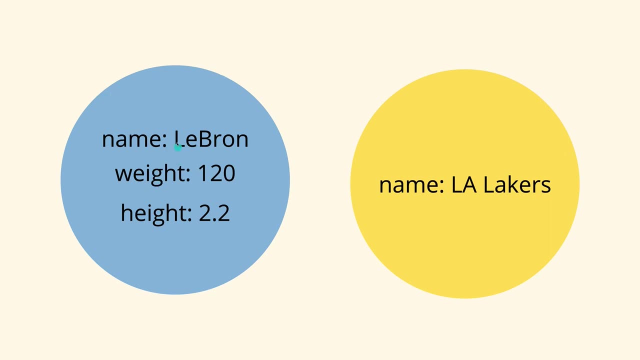 we store data for a specific node. Now let's actually talk about the Los Angeles Lakers. So we understand that now we can have different properties inside of the nodes. So over here we have a name: LeBron, weight 120,, height 2.2.. And then over here we have the Los Angeles Lakers, which is name. 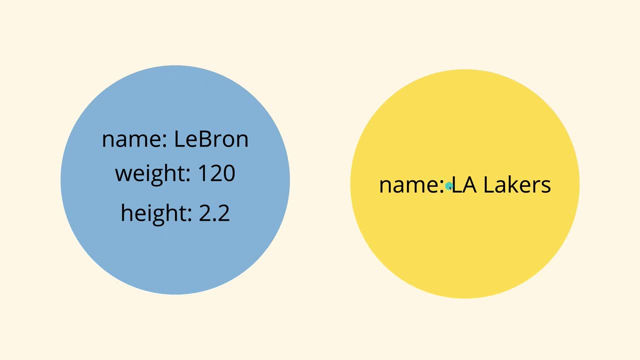 you know Los Angeles Lakers. Now my question is is: how do we know that this node belongs to, well, is a team, whereas this node over here is a player? Well, what we can do actually to kind of distinguish the two is give each node a label. So let's say that this node is a player. So let's. 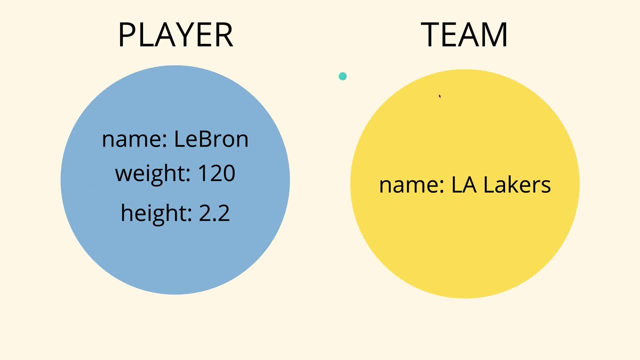 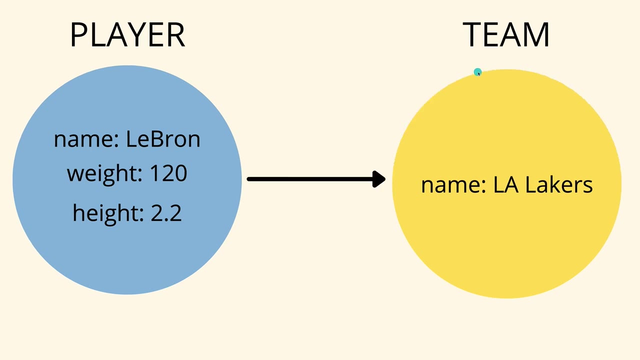 label. So we can give this node the player label, And then over here we can give this node the team label. So in order to separate our nodes, because they might be different entities, we give them labels. So over here, player label, over here we have the team label. Now the last thing I want: 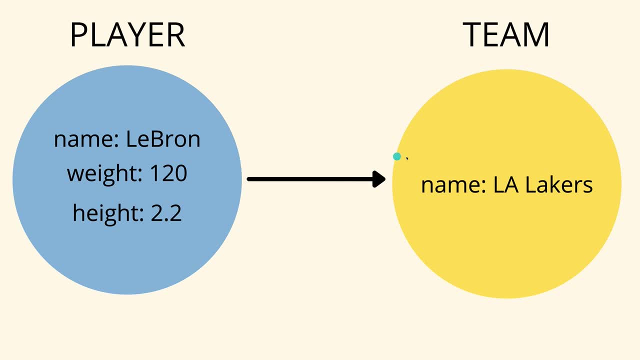 to talk about is the relationship. Remember, relationships are only going to go in one direction, So we have one direction. Now, if you want to have, you know, two directions, we would have to create two different relationships. we have to create a relationship here. 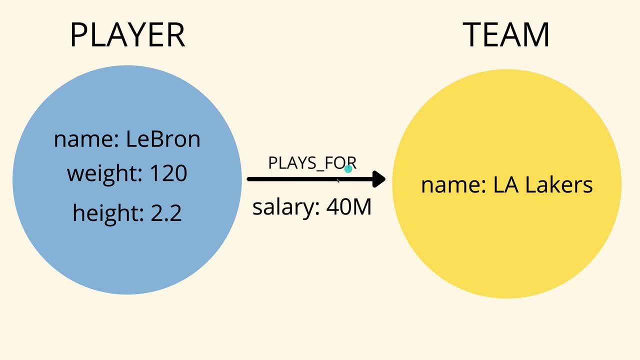 and then a relationship here. But now let's say, though, I want to say that, okay, this guy plays for the Los Angeles Lakers, But what's great about it is I can also add properties inside of the relationship itself. So maybe I can add LeBron's salary inside of this relationship, And 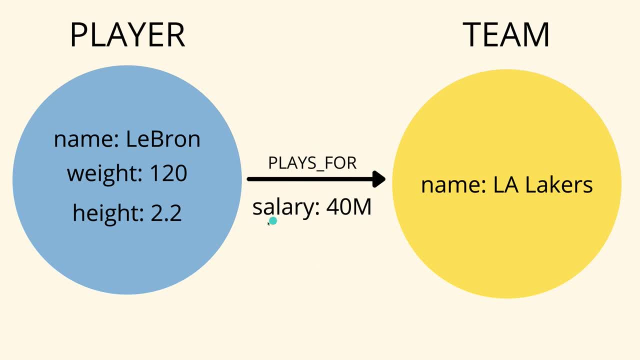 we can add, of course, multiple other ones, But that's what's nice about Neo4j and graph databases: you can actually add properties to the relationship itself. So if I wanted to get LeBron's salary, I can add a property to the relationship, and I can add a property to the relationship itself. So 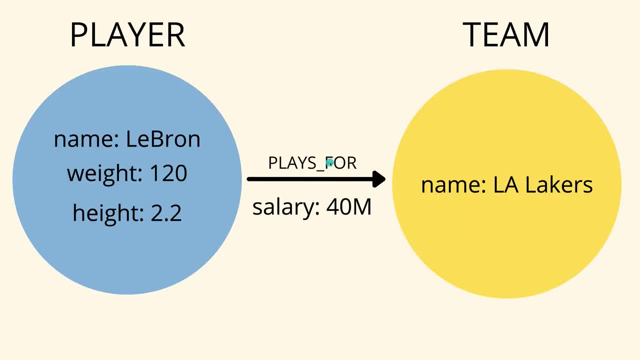 I can add a property to the relationship itself. So I can add a property to the relationship itself. So that is how data is stored inside of graph databases and specifically Neo4j. Now that we have a good understanding of that, let's actually go ahead and get our hands dirty and start coding. 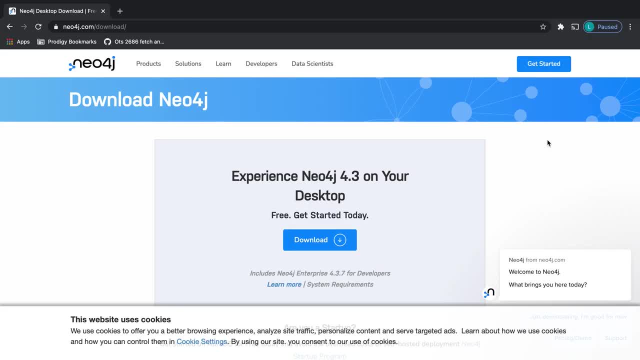 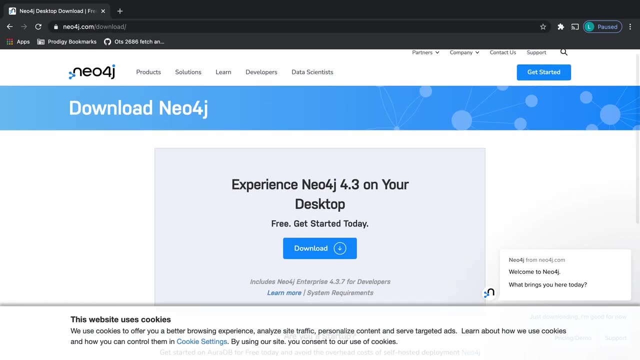 out Neo4j code. In order to get started with Neo4j, we need to install it on our local machine. So to do that, we need to go to neo4jcom slash download, and I'll have this link in the description below. The first thing that we need to do is just accept all cookies. I'm just 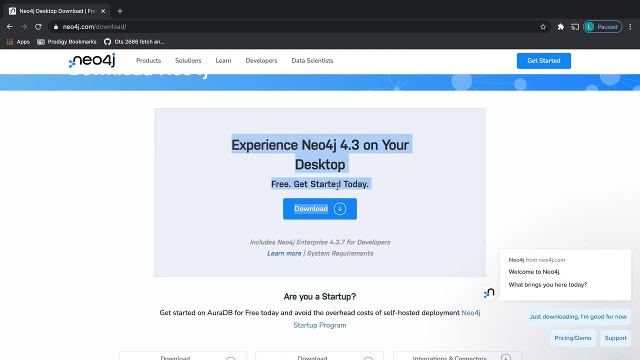 going to go ahead and do that Now over here. it's going to say: well, download Neo4j. and it's going to say version 4.3 or greater for you guys probably. Nonetheless, this is the one that you. 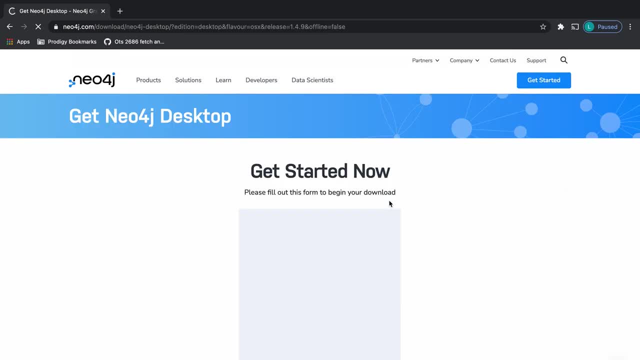 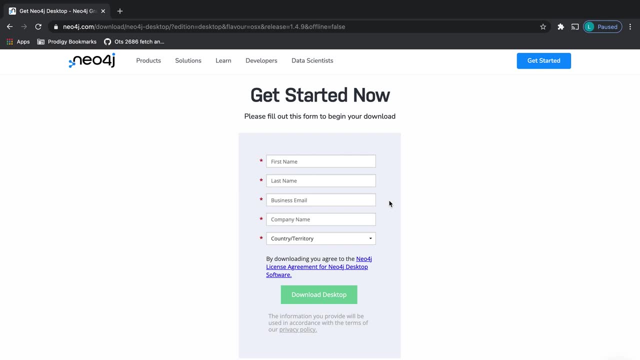 want to download, So you're going to go ahead over here and click download. Now I am on a Mac, but the process for Windows is going to be pretty much the same: 90% the same. There's just going to be a little bit of differences that you guys can probably spot. 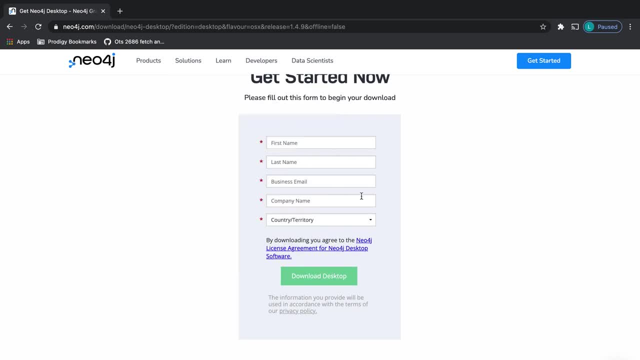 So over here, the first thing it's going to say is: okay, well, I want some of our information. So I'm just going to put in my first name, my last name. Let me just zoom in here for you guys. 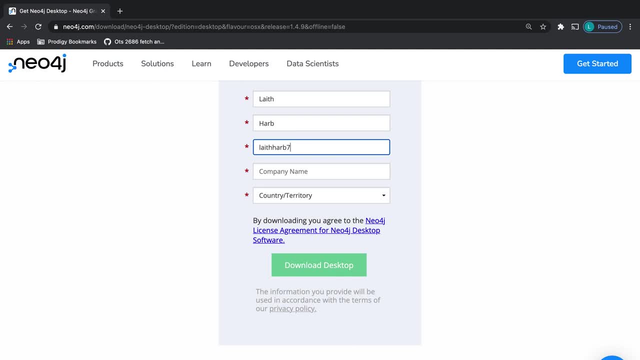 Or maybe I should zoom out, because I don't want you to see any of this stuff. Whatever, It's fine, Gmailcom. And then over here I'm just going to say me and I am in Canada, So I'm going to say 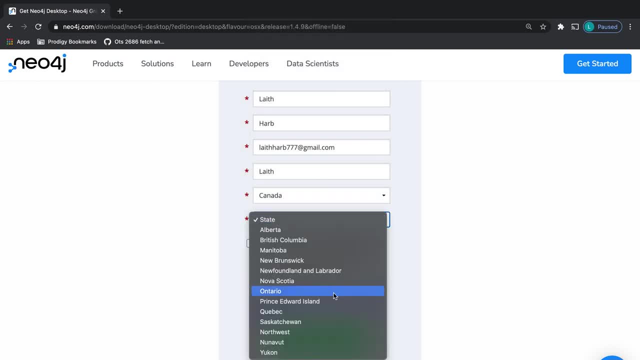 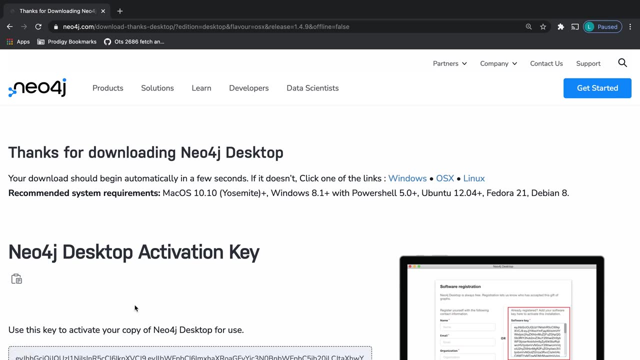 Canada, if I can find it, And I'm in Ontario, All right. So I'm going to go ahead and download this And this should give us a little bit of. so what this should do is redirect us to this page over here, And over here you can see that. 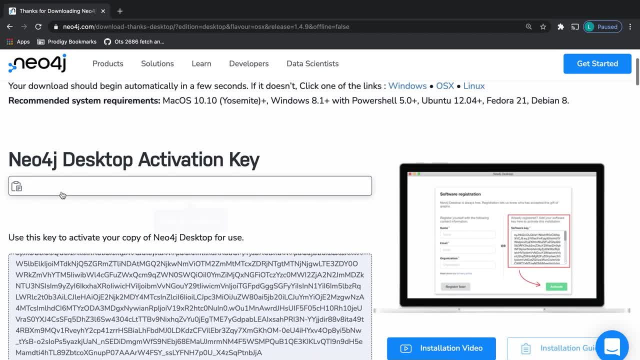 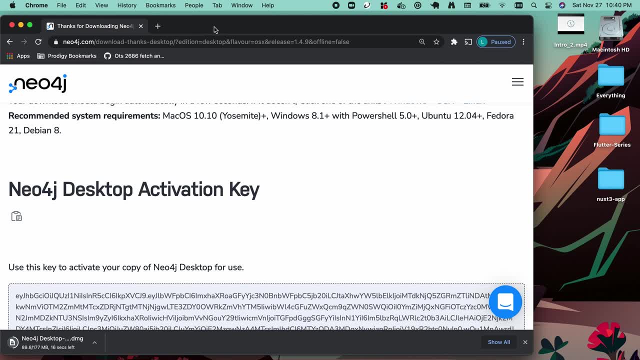 we have this key, And this key is really, really important And we actually need this in order to download Neo4j and activate it to our account. Now the other thing is is if you look over here, you can see that Neo4j desktop is downloading. So let's just wait for that And then we're going. 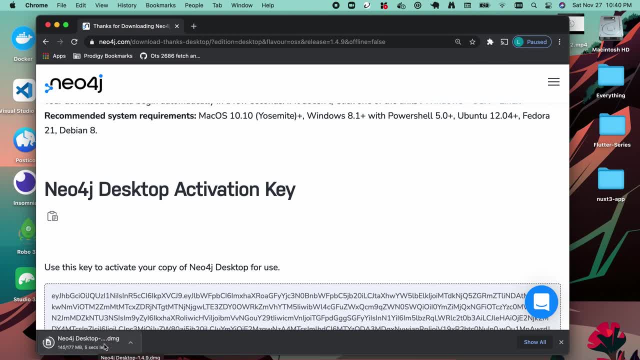 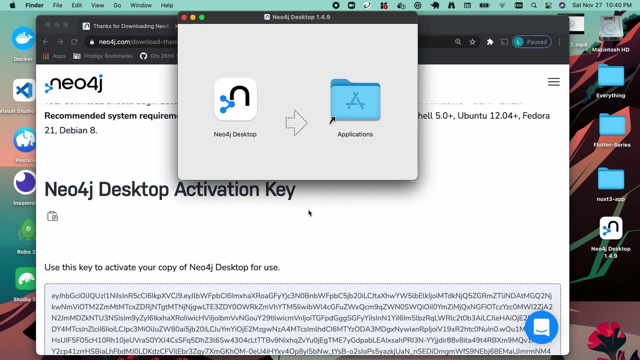 to go ahead and click it once it's done downloading, which should be in like five seconds. So let's give it a quick wait And then we can click on it. All right, So once that is done, we should get this over here, And this is where it's a little bit different, for. 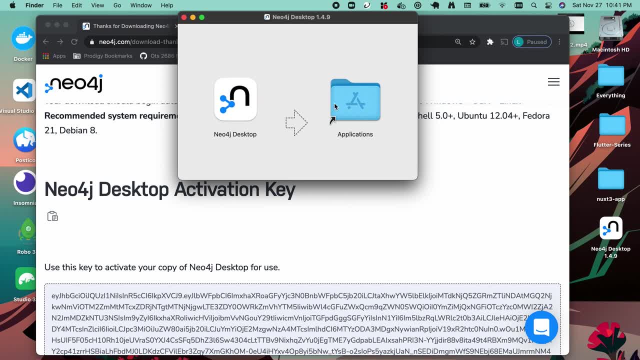 you guys on Windows, The process might be a little bit different. It probably is going to be some sort of wizard. If you're on Mac, all you have to do is just simply move this into your application directory. So we're going to go ahead and we're going to move that in there. 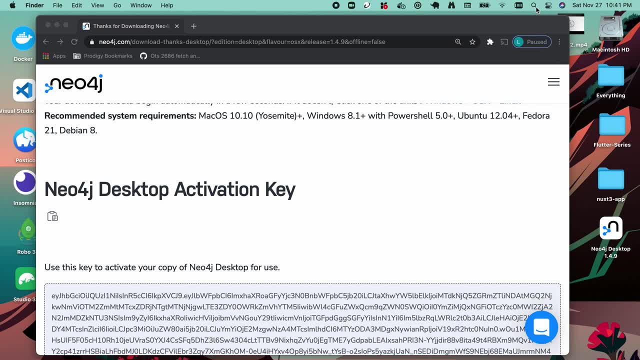 And then, on Windows, it's going to ask you to run it once you're done installing it. On Mac, what you have to do is specifically go and search for Neo4j, click on it and then it's going to go ahead and run. So that's really the only difference between Windows and Mac. Otherwise it's exactly. 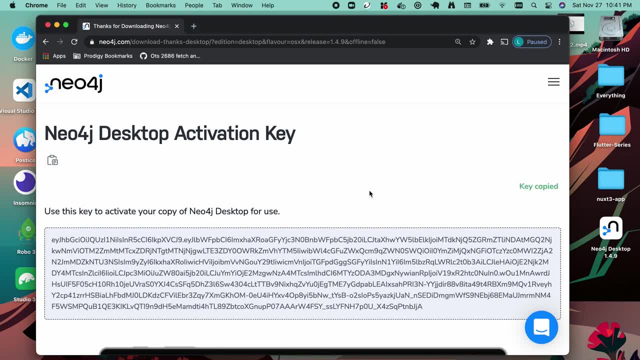 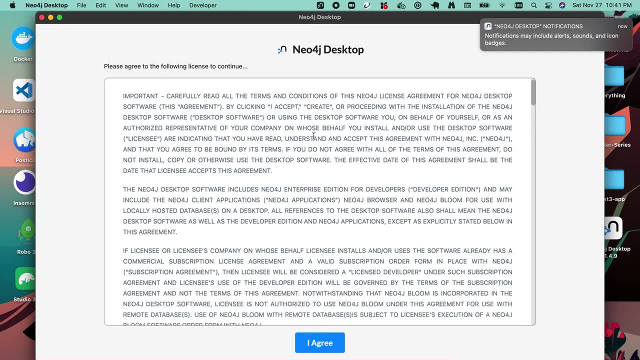 the same, And again we're going to need this key, So let's just go ahead and copy it to our clipboard. So let's just wait. right now, The first thing we have to do is read this licensing agreement, So go ahead and read it. I read the whole thing, So let's just go ahead and copy it to our clipboard. 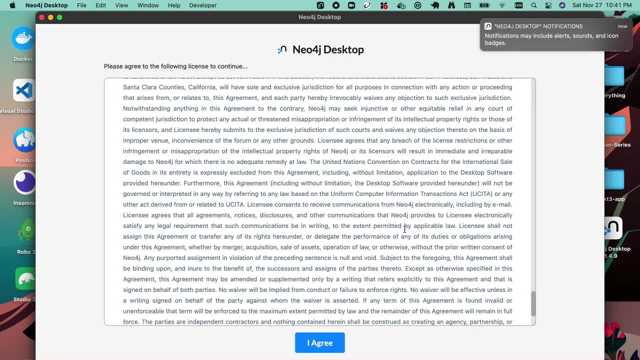 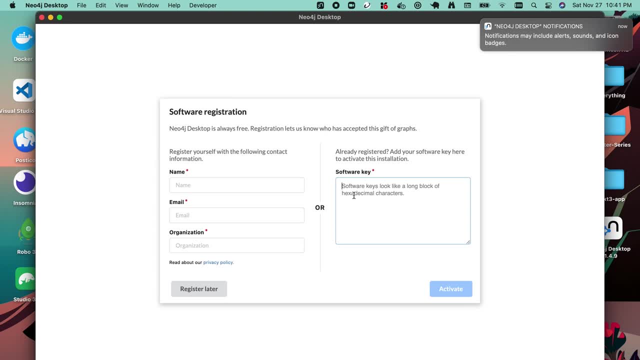 I read the whole thing. I'm joking, I didn't read any of it, I just agreed. And then I'm going to go over here and you can either register with your email or with that key that you were provided. We're going to go ahead and paste in that key and we're going to activate our account. Let's get rid. 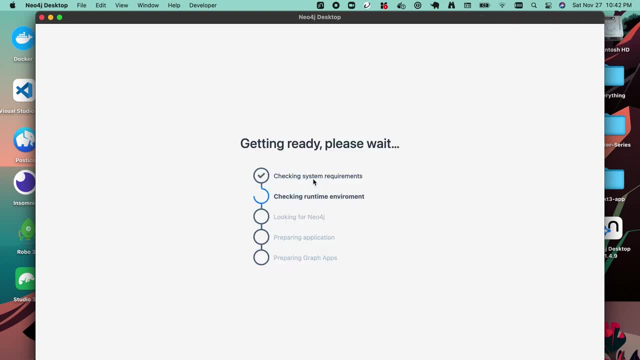 of this, All right. So now it's just going to do a little bit of checking. It's going to check our system requirements. It's going to download the runtime, which I'm not going to pause for because it seems like it's going really fast. I was going to look for Neo4j, et cetera. blah, blah, blah You. 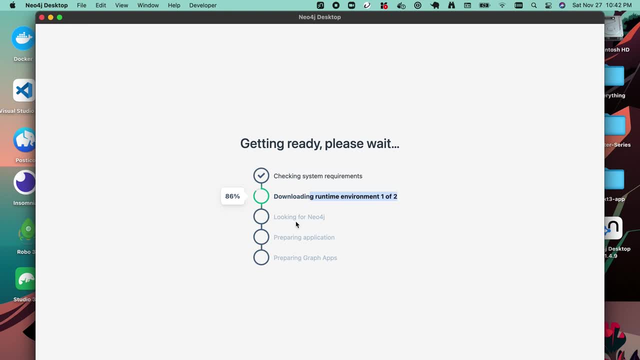 guys kind of get the point. This is just a download process, So let's just wait for this to finish up. All right, So how was your day, guys? I'm trying to stall as much as possible. Okay, It seems like this is going to take a while, So I'm just going to pause the video. 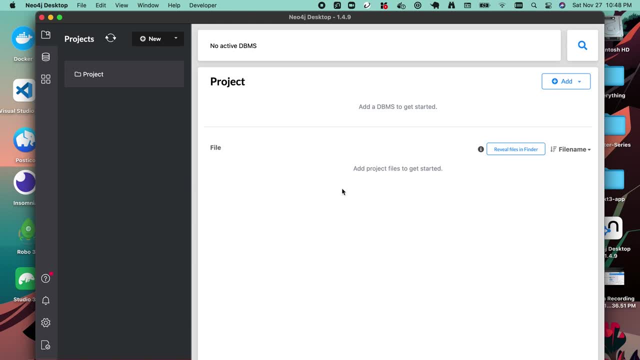 Once the download procedure is done, you should get redirected to a page that looks like this: You'll probably see something regarding the movie databases, And what I want to do is I want to just go ahead and delete that project. So let's just go ahead and delete it and let's create a brand new one, And so this project is. 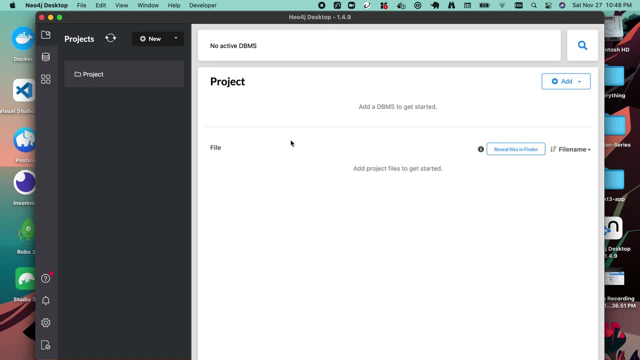 going to be storing a lot of MBA data. That's what we're going to be working with within this crash course to learn Neo4j. So what we're going to do is we're going to change this project name to MBA, And what we want to do is we want to add a Neo4j database management system. So what we're going- 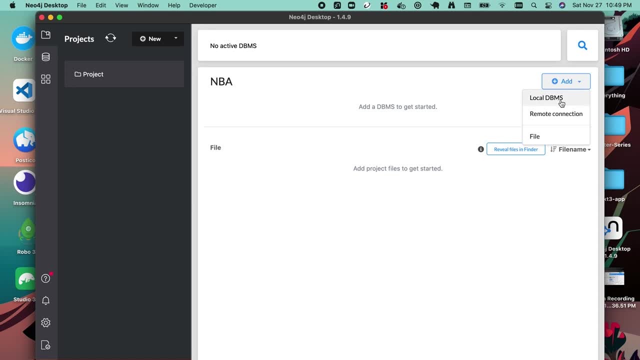 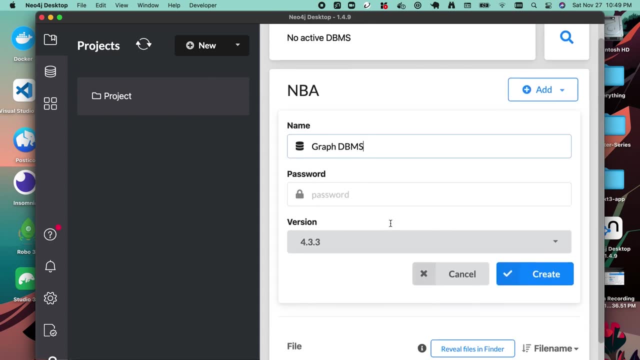 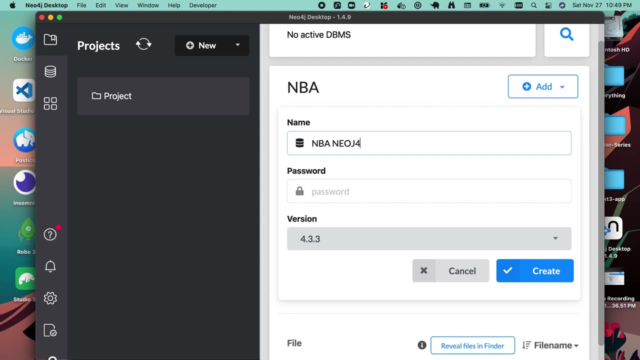 to do is we're going to click add here and we're going to say local DBMS for database management system. Let me just zoom in here: click over here, We're going to do this, And then, over here, what we're going to do is we're going to give our database a name. Let's just call it MBA, Neo4j, And 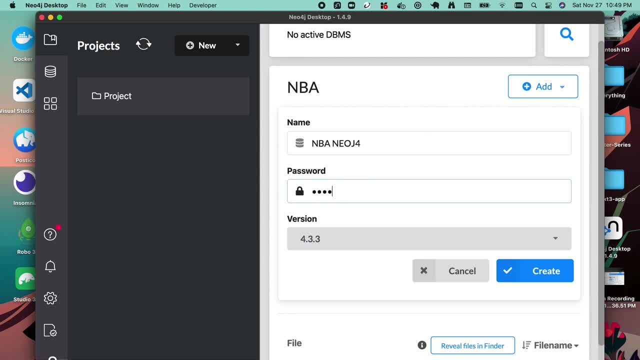 then we're going to give it a password. I'm going to call it well password, And you have to remember this password. Let me just go over here again: password, You have to remember it. Remember, we're going to go ahead. 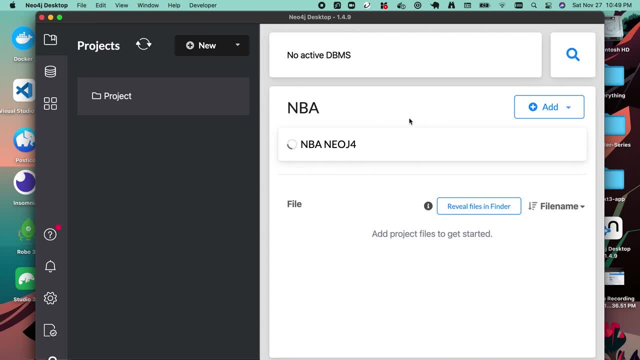 And we're going to create this database management system. So let's just give it a while. This will take maybe a few seconds. I don't suspect that it will take a minute or two, but it should take a few seconds. So TikTok, MBA stands for National Basketball Association, And so now what? 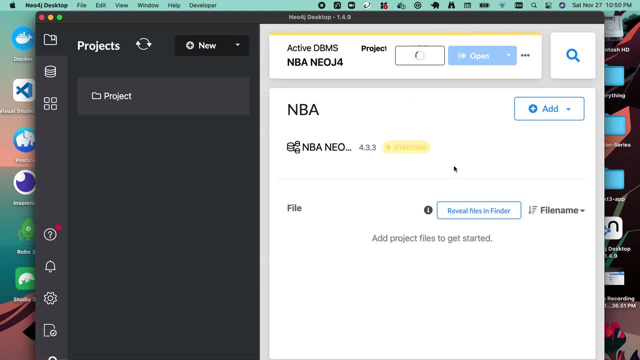 we want to do is: we want to go ahead and start this. So let's go ahead and start it. And again, this should take a few seconds, not a minute or two, but a few seconds. I hope Let's just wait this out. Now that we started our database management system, you can see that. 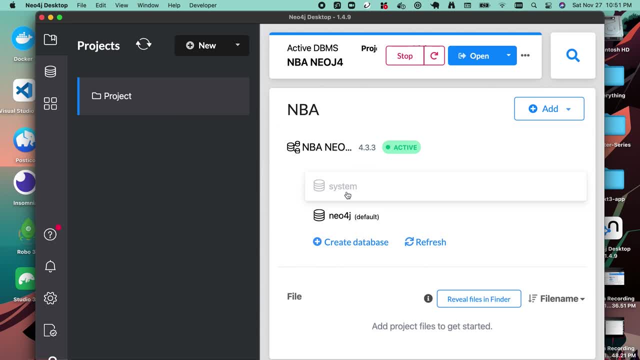 inside of our database management systems. we have two databases: we have the system database and we have this default Neo4j database. Remember, the database is where we are going to store our nodes, as well as our relationships. Okay, so now what I want to do is I want to 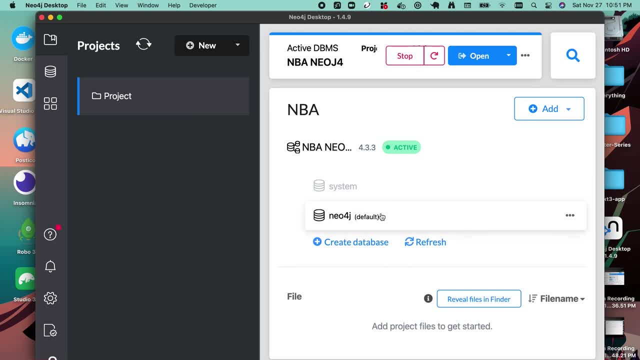 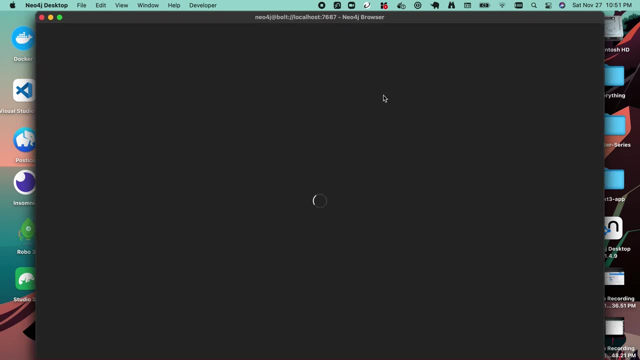 connect to this database and start writing some queries in order to add nodes, as well as retrieve nodes, etc. So, in order to do this, what we're going to do is we're going to go to this over here, graph apps, we're going to click on Neo4j browser And what it should do is redirect us right over. 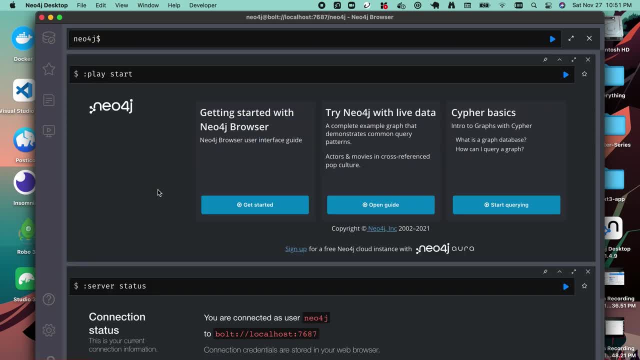 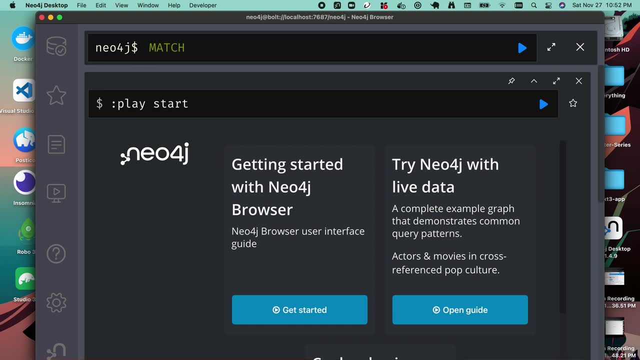 here And now. what we want to do is connect to our database. So what I'm going to do is I'm just going to write a quick query And let me just zoom in here. you don't have to understand this query. I'm just going to go ahead and write this And what we should get. 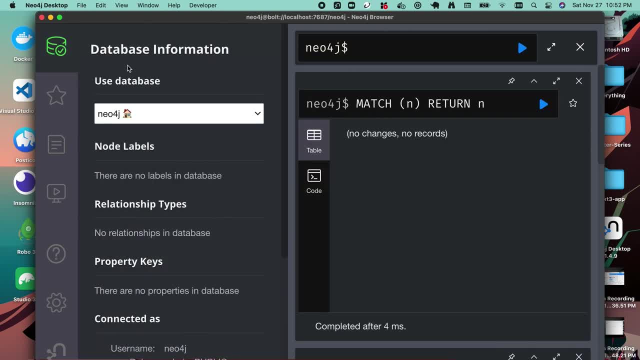 back is nothing, And what's happening is it's actually already pre connected to our query. So you can see here that this is the database information is called Neo4j And it's connected to the MBA app, So it's automatically connected to it. Isn't that amazing? So right in here. 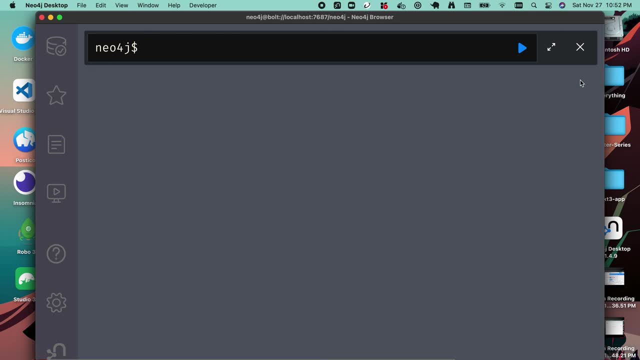 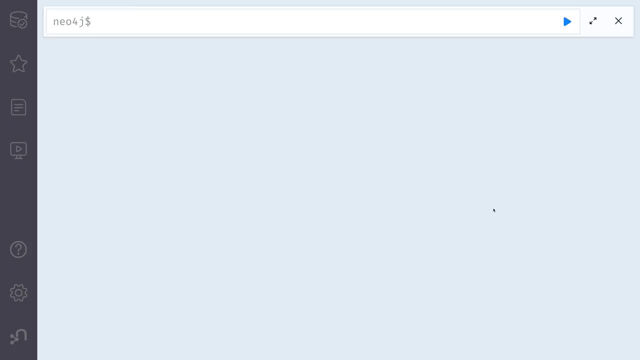 this is where we are going to start executing our Neo4j code. So you know what? let's just get right into it. In this section of the course, what we're going to learn about is querying data, that is, retrieving nodes as well as their relationships. However, in order to do this, we need to have data inside. 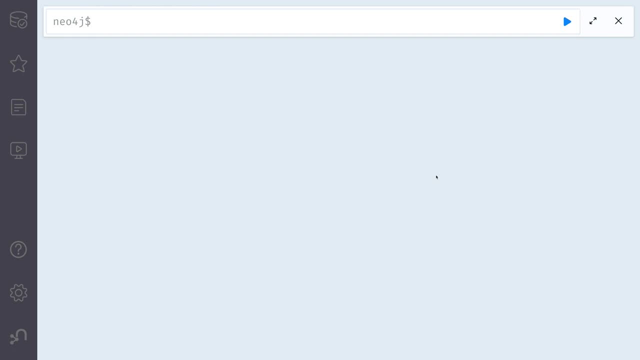 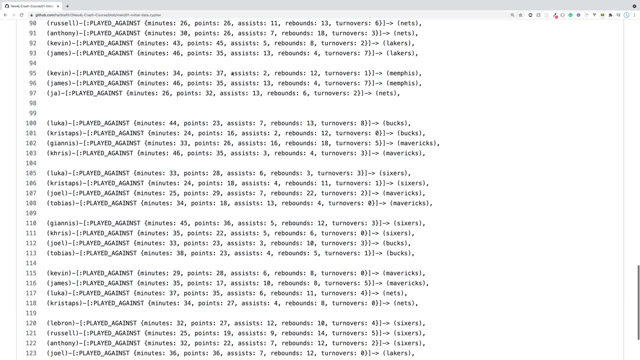 of our database And, as of yet, we have no data. So we're going to learn about how we can add and create data inside of our database, But for now, what I want you to do is I want you to go to my. 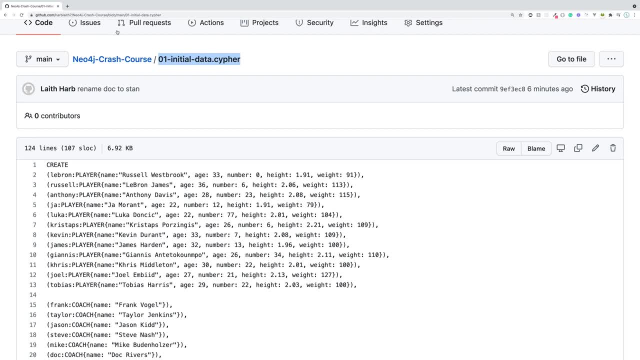 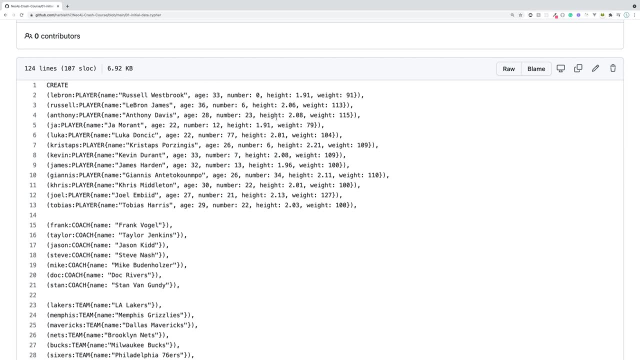 GitHub page and go to Oh one initial data- And I'll have this somewhere linked in the description below- And what this is going to do is run a mutation that is going to create a bunch of nodes as well as their relationships, And all this data pertains to something related to the MBA, So 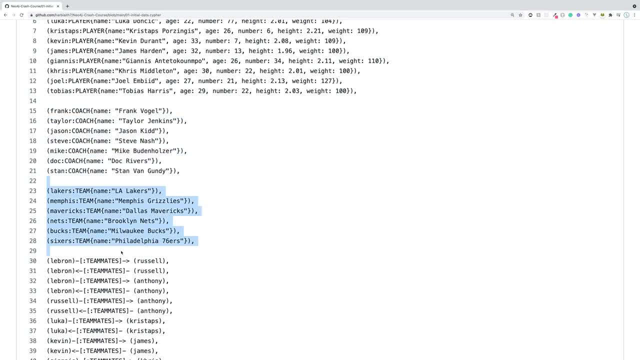 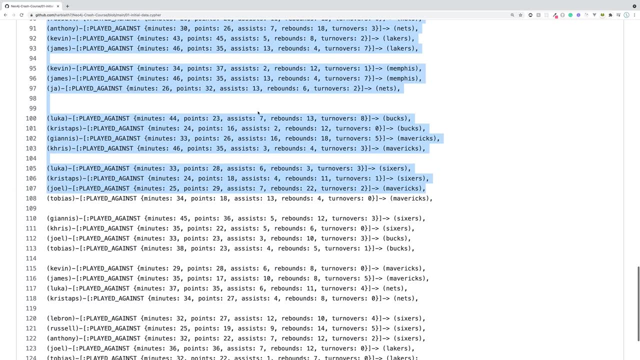 over here we have NBA players, we have coaches, and then over here we also have some teams, And then over here we have a bunch of relationships. So if this code doesn't make any sense to you, that's completely fine. we'll learn about how we can create. 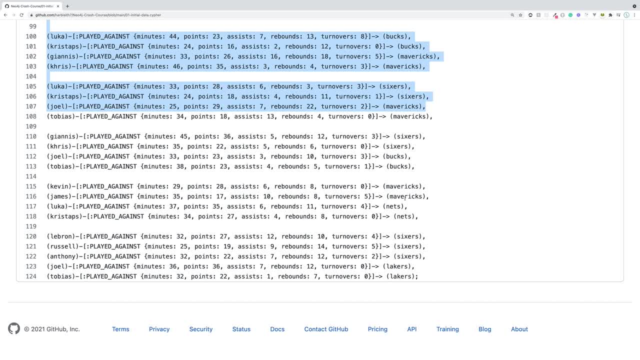 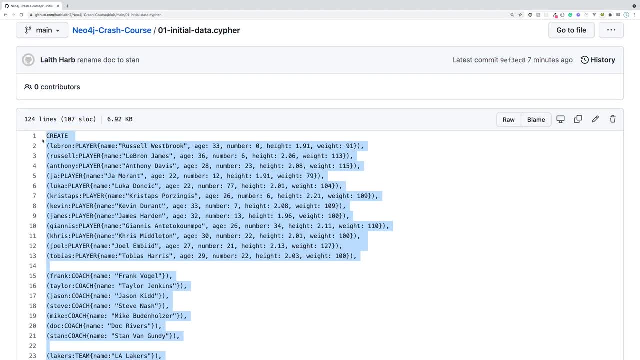 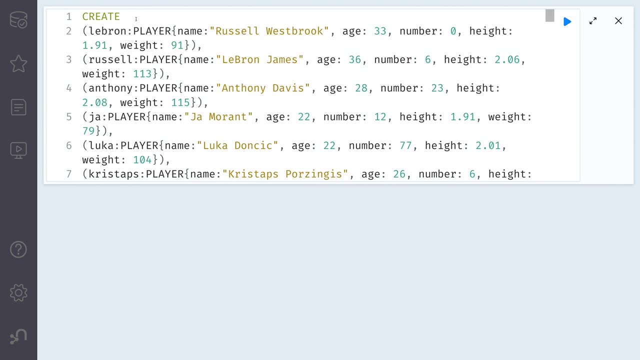 data a little bit later, But for now, I want to focus in on how we can data. so let's just quickly copy all this code. let's copy all this awesome, and what we're going to do is we're going to paste it right in here. now. this right here is actually known as cypher. 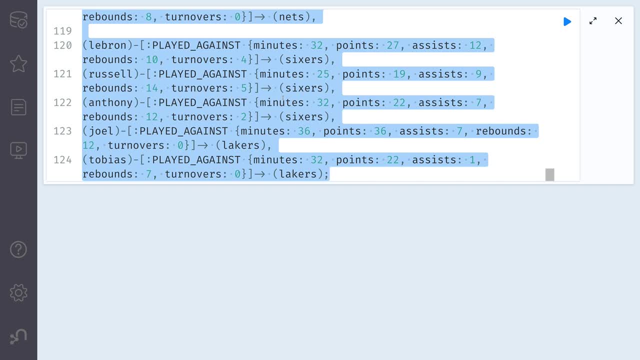 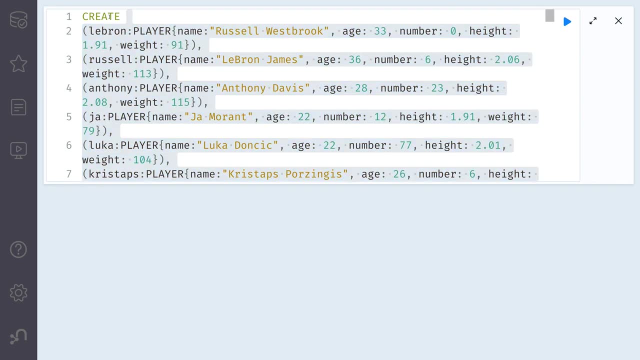 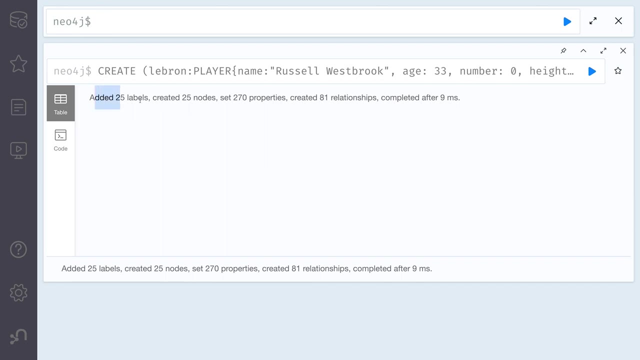 code. so neo4j uses cypher. so, just like postgres uses the sql query language, this is another language called cypher. it's not really important, but just for you guys to know. so we're going to go ahead here and we're going to execute this and we should see this window right over here saying: 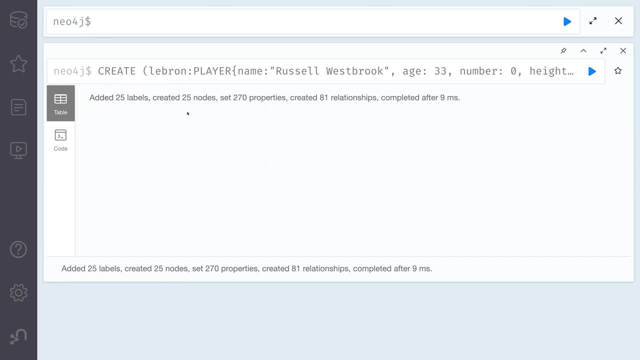 that, hey, we have added 25 labels. we'll talk about what labels are, but you probably know what they are already, because i explained them to you- and then over here we have 25 nodes we're added, we have a bunch of properties and relationships, and so what we can do is we can just get rid of that. 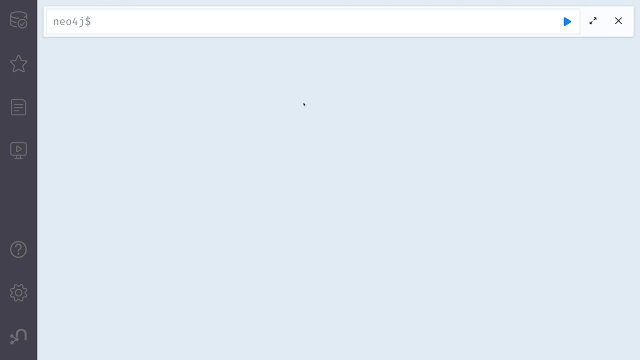 we have data inside of our database, so let's begin with querying data. now. let's remember, inside of neo4j, we have two different types of things that we can store. we can store a node, which you can think of as an entity, a thing, so in this case it's either going to be an nba player, an nba coach or an nba team, and then we 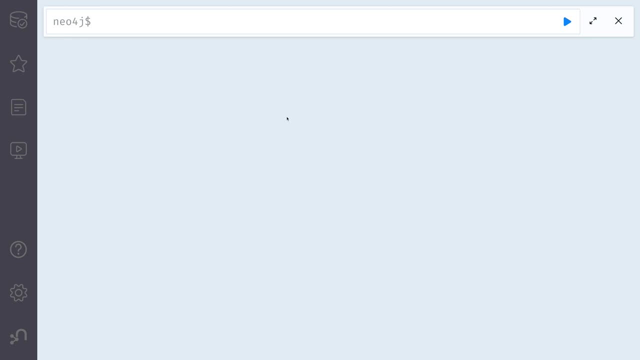 have the relationships between those nodes. so let's forget about the relationships. let's first learn how we can query nodes themselves. now, using the cypher language, what we need to do in order to query for something is state that we need to query for something, and we state that by using the keyword match. so let me just zoom in here for you guys, just so you. 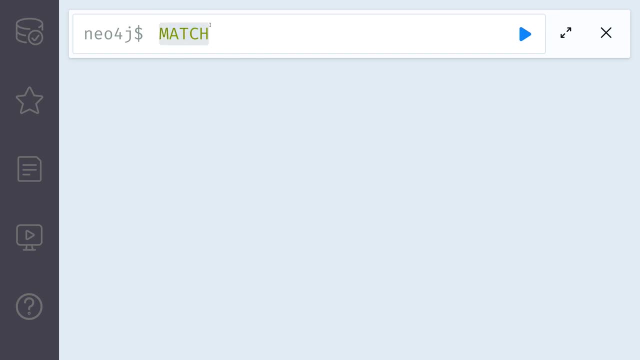 can see, match is the keyword that we utilize in order to query for things, so that's exactly what we're always going to start with when we want to fetch data, and then, well, we want to fetch a node. a node in cypher is always going to be representative as two parentheses, so two. 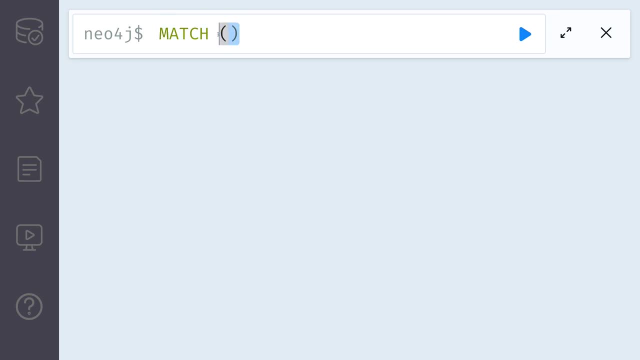 parentheses. so we want. what we want to do is we want to create a node and we want to create a node to match a node and then in here we can give this node a specific variable, so we can just call this node, we can call it whatever it is that we want, but we can call this node and it seems like node. 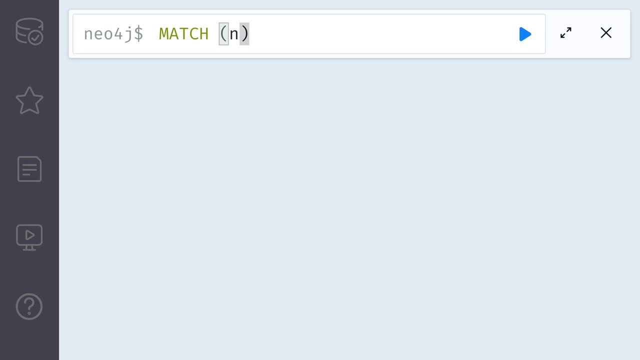 is actually a keyword. let's just- yeah, let's just use n for for for node, and then what we want to do is, well, we want to return those nodes because, okay, this matches the nodes. but now what we want to do is, we want to return that node. we eventually want to get that node back. 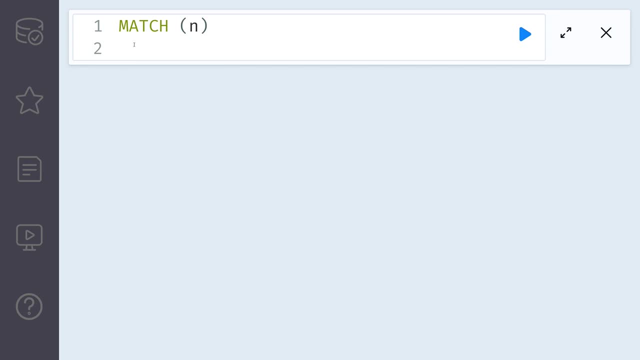 so what we can do is we can do control shift to uh or control enter to go to the other line, and then we can say return and return n. and what this is going to do? what this very simple query is going to do- is it's going to take all of the nodes inside of our application and return it. 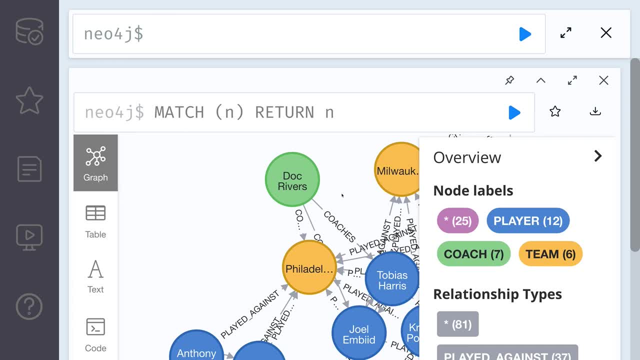 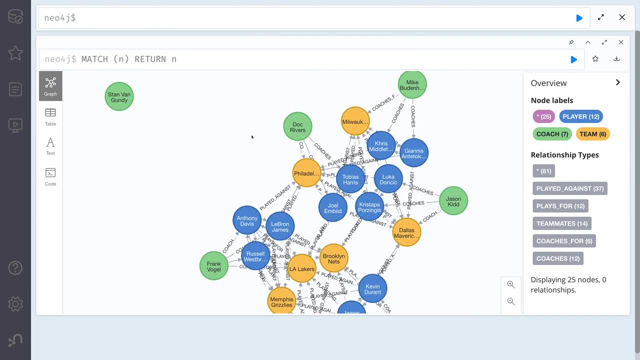 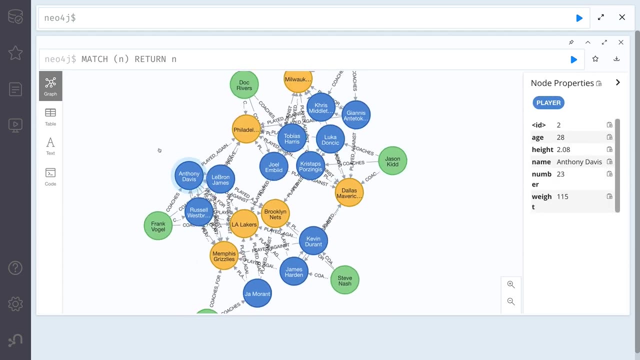 so let's go ahead and execute this, and there we go. let's actually zoom out a little bit. so i'm going to be zooming in and out quite a bit and over here you can see that, well, we have a bunch of different nodes. we got all of our nodes. so you can see, here we have the player. 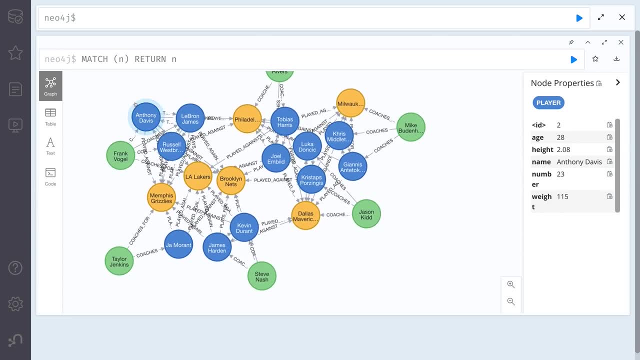 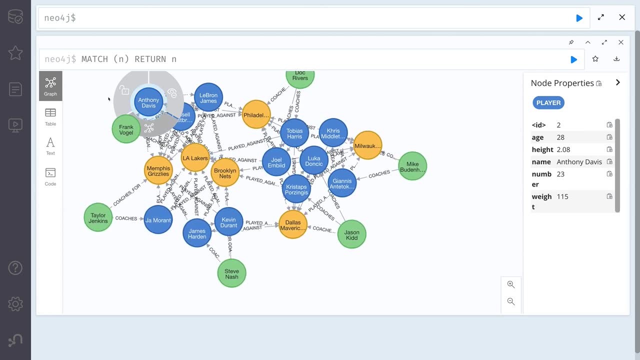 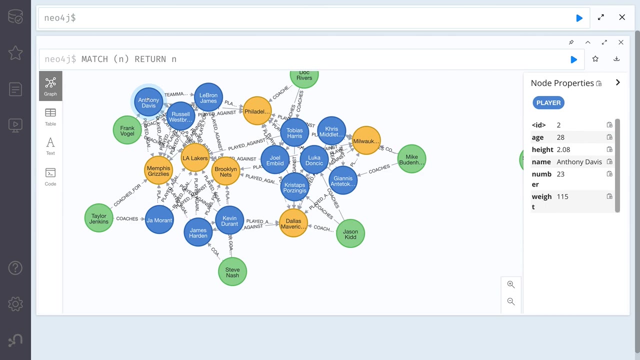 nodes and you can see that they're all organized in different colors. so over here we have the players and also we have these crazy relationships. even though we didn't ask for the relationships from this graph format, we always get the relationships if there are relationships between nodes. so over here you can see that we got anthony davis, we got russell westbrook, we got. 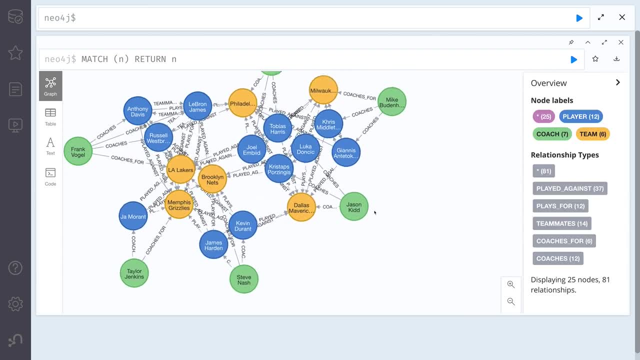 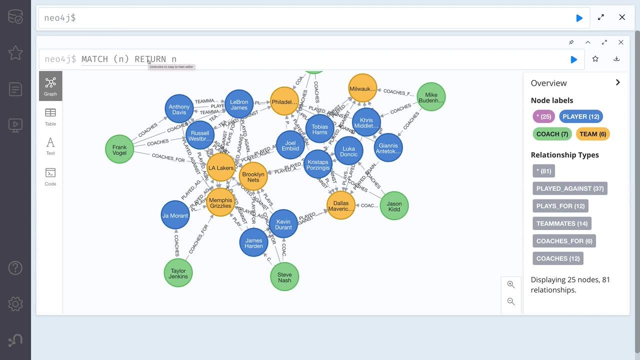 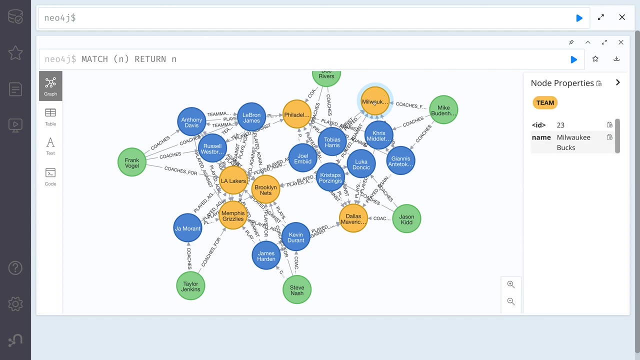 frank vogel, which is the coach. we got the grizzlies, so we got a bunch of different nodes and that was the query to get those nodes. so now let's actually think about how we can maybe filter for specific nodes, for example, maybe i don't care. 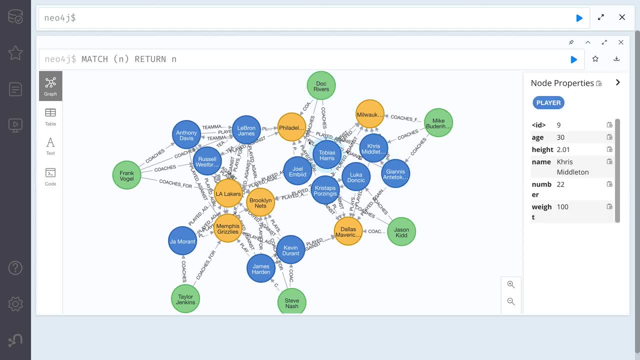 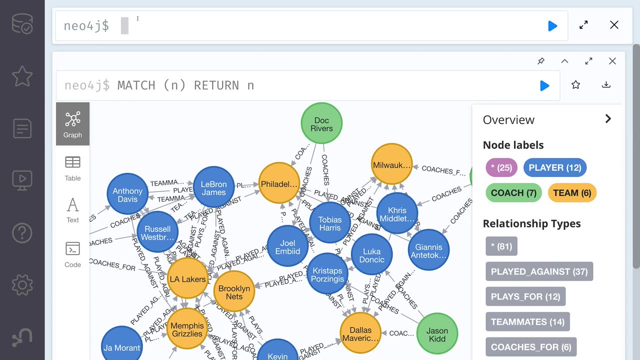 about the coach. maybe. i don't care about the team, i just want to get all of the different players. so let's zoom back in here and let's think about how we can run this query so i can get all of the player nodes rather than, you know, the team nodes and the coach nodes. so the first thing that we're going to do is 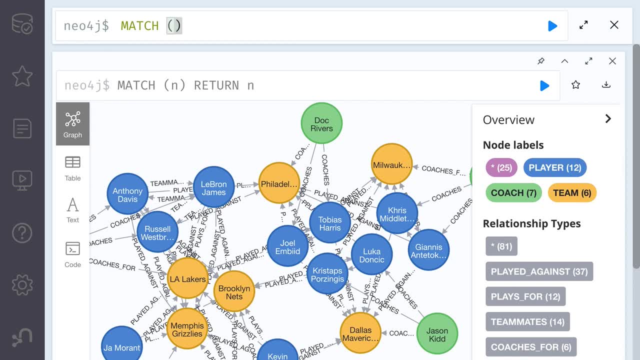 we're going to say match, then we're going to say we want to get a node, so we're going to represent that with these two parentheses, and then we're going to say return, and what we want to do is we want to return, uh, whatever the variable we add in here. so let's just say n- n, so what we want to do, 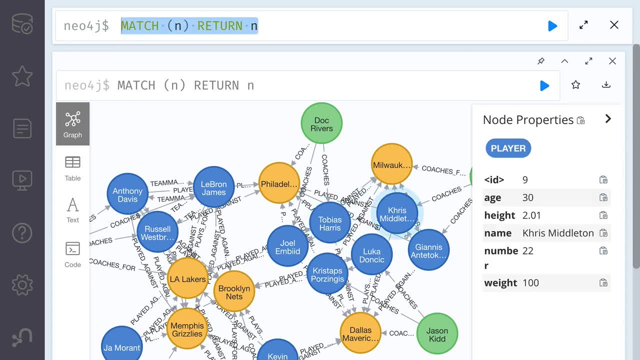 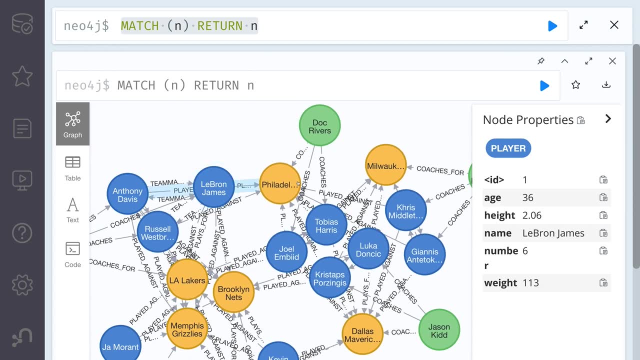 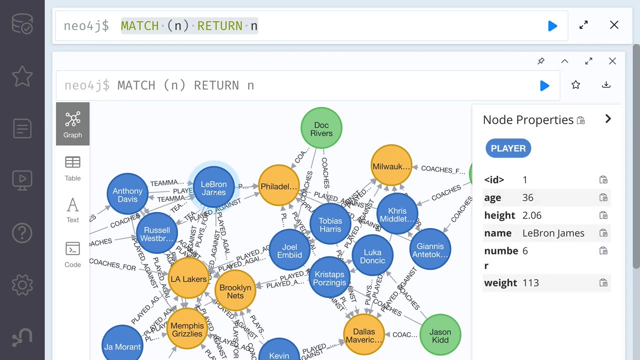 right now is: this is going to match every single node and give it to us now. we want to specify that player nodes- now remember, all nodes- have different labels attached to them, so we can actually attach labels to them. and if actually, if i hover over lebron james, you can see that, uh, to the right, we 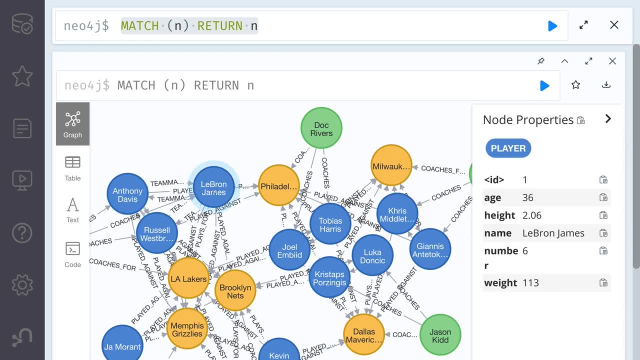 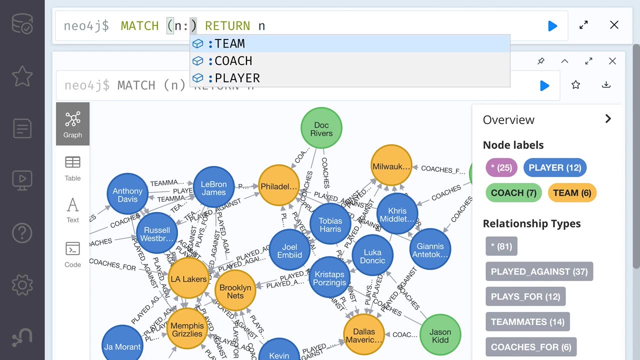 have these node, uh, node properties, and it says player, this one says team, this one over here says coach, and so what we can actually do is, inside of these parentheses that are- that is represented of the node- we can say colon and specify what label we want to get. in this case, we're saying: 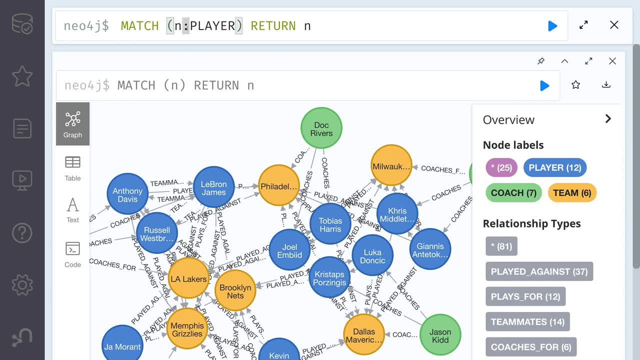 that, hey, we want to get all of the nodes that have the player property and we can actually change this right now. this variable name, this is variable, so we can call it whatever it is that we want. you can change it to player if we want to, because now it's more indicative of being a player. so we 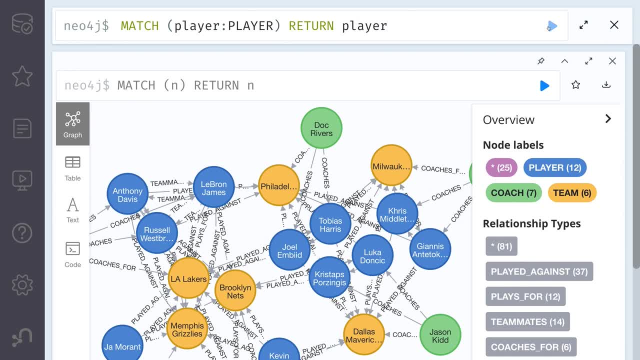 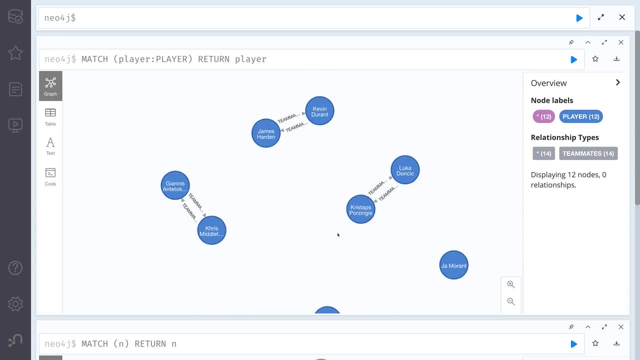 can go over here, say, player, you want to return player. and if i were to execute this and let's zoom out again, you can see now we get all of the players as well as their relationships. so over here you can see, we have kevin durant, we also have james harden. 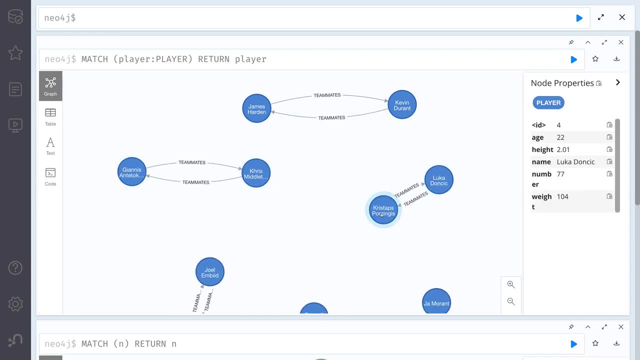 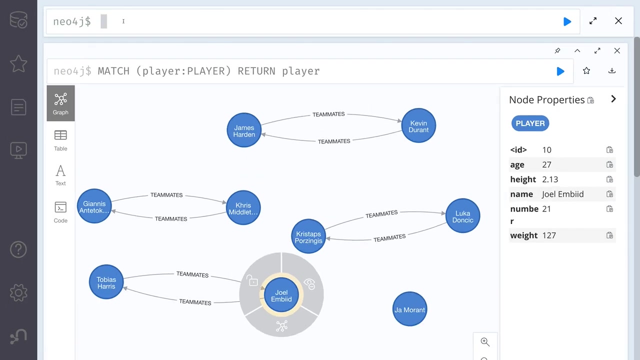 their teammates: yannis and then chris middleton, luka docic, and then we have all of these relationships and of course, we can do this for coach as well as for team. so we can go over here and, if we want, what we can do, and let me zoom- 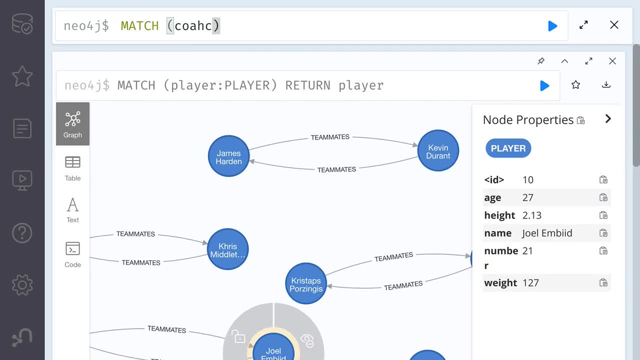 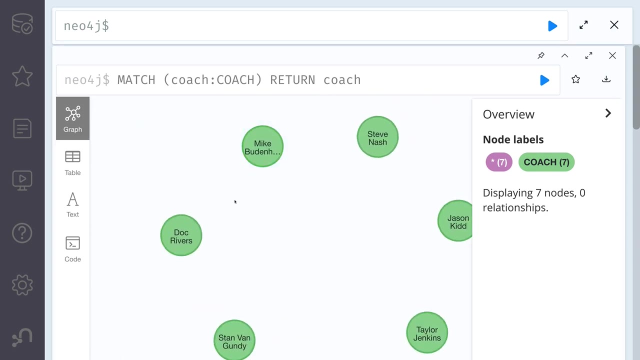 right back in we can say match and we can say coach. and then over here we can say: i want to be coach and i'm going to say return coach, return coach. so let's go ahead and execute this. and you can see, now we get all of our coaches and there's no relationship between coaches. so that's completely. 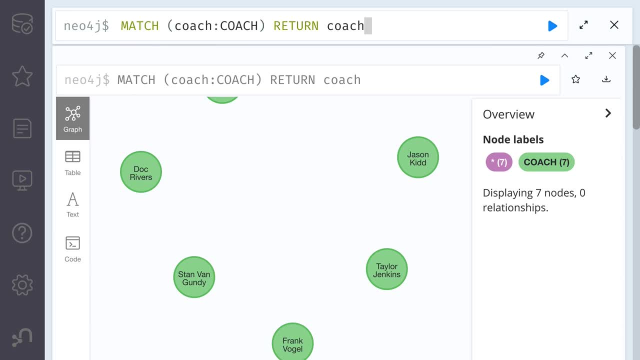 fine now i highly encourage: try this on your own. get all of the team nodes so i'll give you guys five seconds to pause the video and do it on your own. all right, hopefully you guys tried this. this is going to be relatively simple. we're going to say: 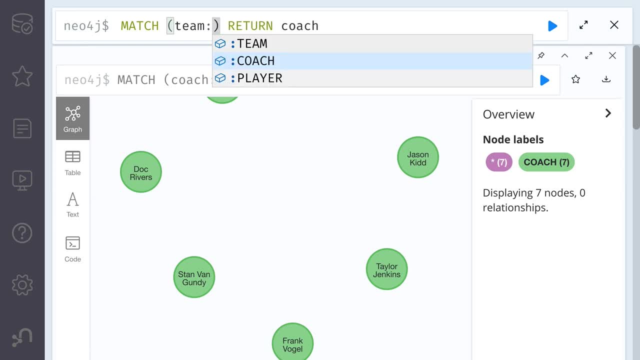 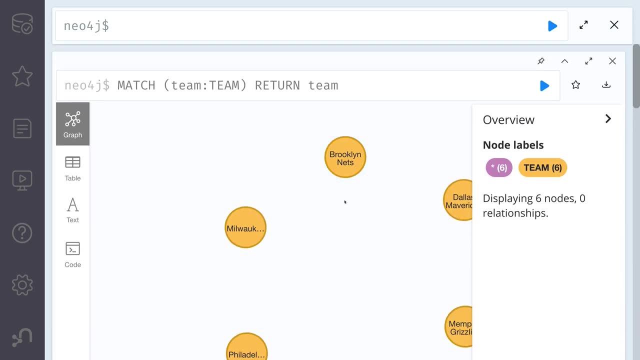 well, we want to get a node. we're going to call this team and then over here we're going to give it the label team, and then we're going to go here and we're going to say return team, and then over here you can see that we get all of our teams. how terrific is that. okay, so let's actually go back a. 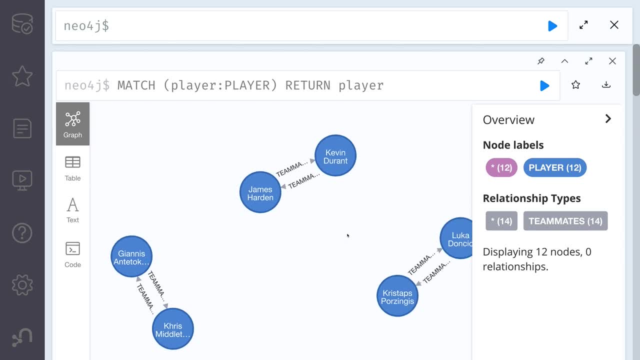 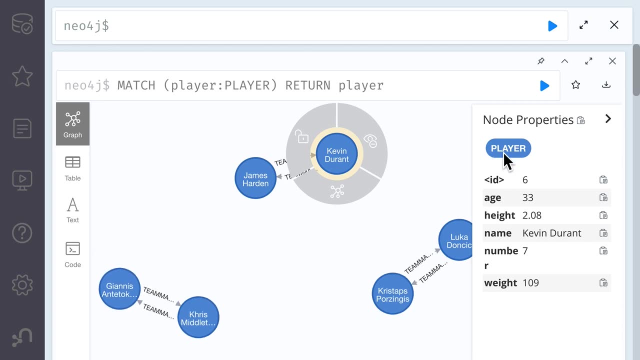 bit and let's go to all of the players. now what i want to do is i want to click on a particular. so when i click on this particular player, you can see that this player has the label ball player. and then over here we have a bunch of different properties. so remember, a node is: 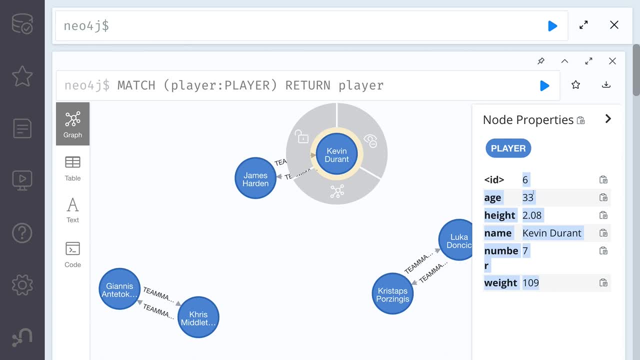 going to have a label as well as a bunch of different properties. it has an id, it has- well, i added- an age, it has a height, it has a name, it has a number and also has a weight. so what we can actually do is we can actually fetch for specific properties. we don't have to fetch for the node. 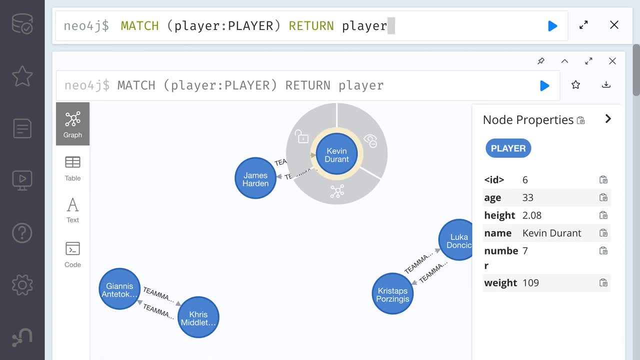 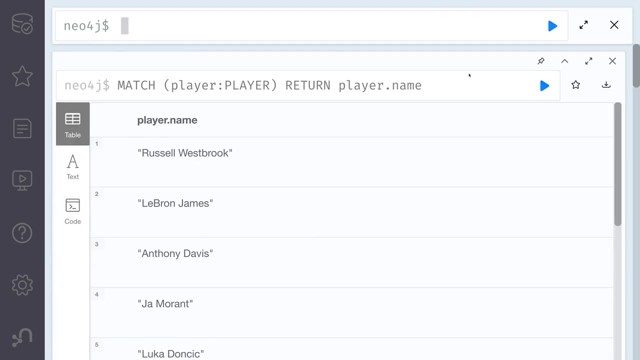 itself. so, in order to do this, what we can do is: well, we can do match, we can do this query, but instead of returning the whole player, node. what we can do is we can return a specific property on that player, so we can return maybe their name. and if we were to execute this, what we get is we. 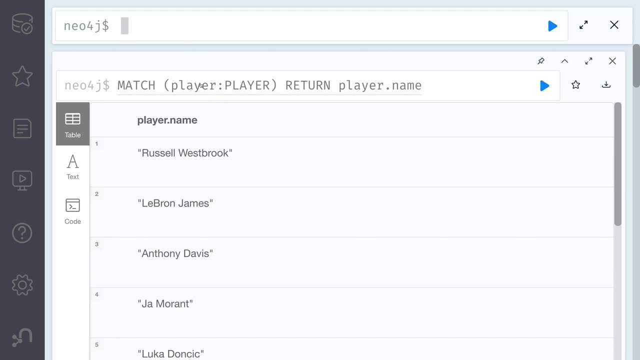 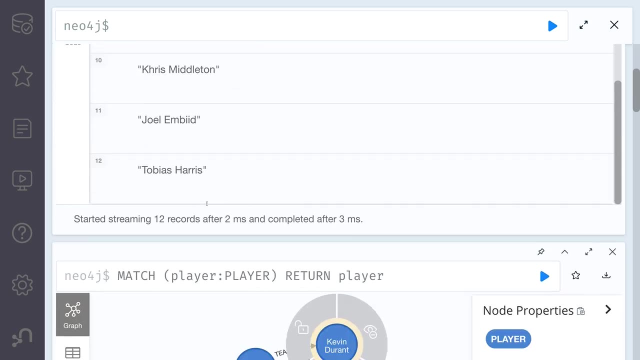 get this table format, because at this point, we're not returning nodes, we're returning properties. but you can see here that, well, we have russell westbrook, lebron, john rand, luca and all these names and that's all we're getting, and we can actually get more. if we want to, we can get more. 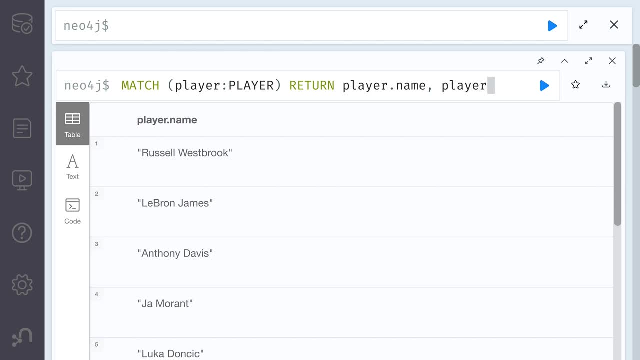 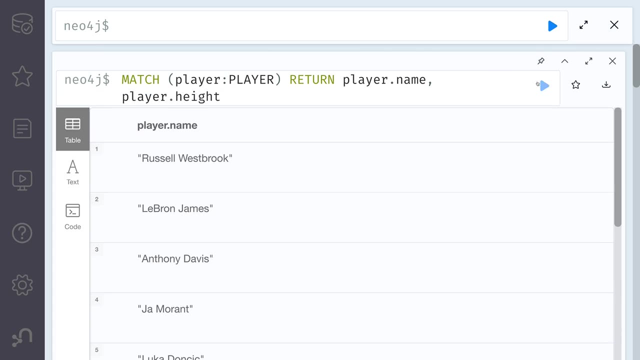 properties. all we have to do is say comma and then player, dot and then whatever property we want. so, for example, we can also get their height. so if you were to execute this, you can see here we get their name as well as their height. now over here you can see at the table it's called the player. 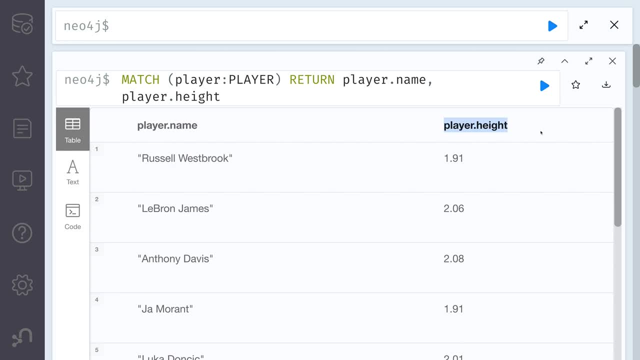 dot name over here also, this is called the player dot height. we might not like to use the player dot name, but we can actually use the player dot height like this name at all. so what we can do is we can actually change this name by using an alias. 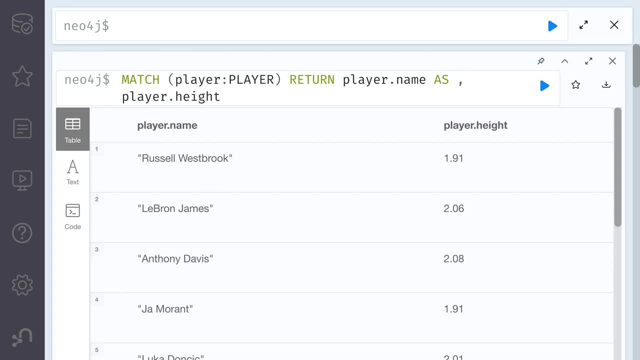 so, in order to use that, we say as, and then we can say: i don't know mba, player name, or we can call this whatever it is that we want. you can just call it name if we want to, and then over here we can say as and we can say as height. so if you were to execute this, let's just execute it here, you can. 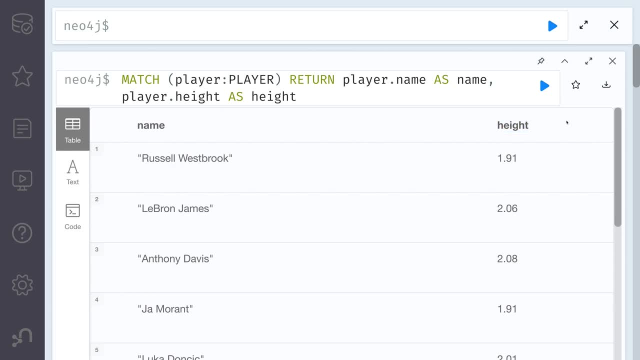 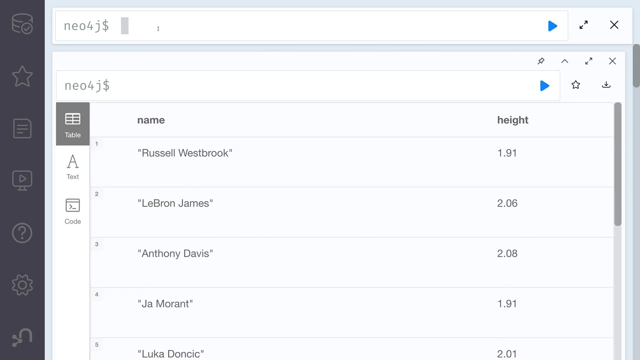 see that the names are now different. rather than player dot name, they're called name and height. all right, cool. so i hope this makes sense and that's really how we can query for specific uh, specific, uh notes. now, one thing that i want to note is that, of course, you can filter your notes, so we actually 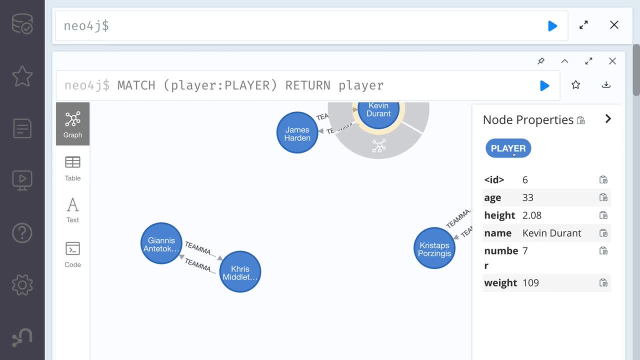 started filtering our nodes by utilizing the label, and maybe that's not enough for us. maybe we want to filter- for you know- nodes within the player label. so let's start talking about the how we can filter our notes. so, for example, let's begin with a very, very simple thing. let's say we 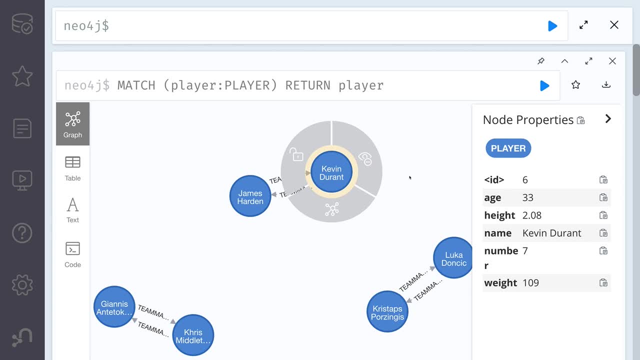 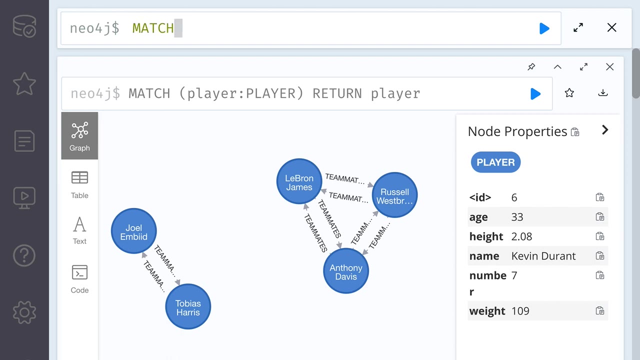 want to query for lebron james's node. we just want to get this node right over here. we don't want to get any of the other ones, we just want to get this node. how do we go about doing that? well, let's zoom in here. in order to do this, what we're going to say is very simply: match and then. 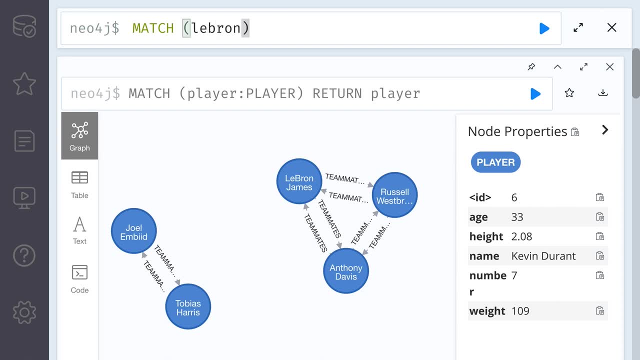 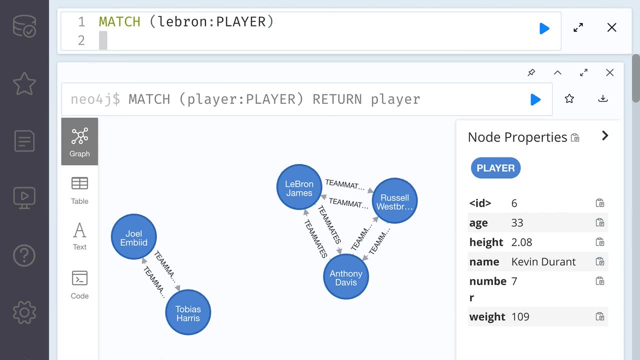 of course we want to match a node. now this node, we can actually just call it a node, and we can call lebron, and we can specify that this is going to be a player node. and now what we're going to do is: let's do shift, enter, let's just say we want to return lebron, so return lebron. so here what we're. 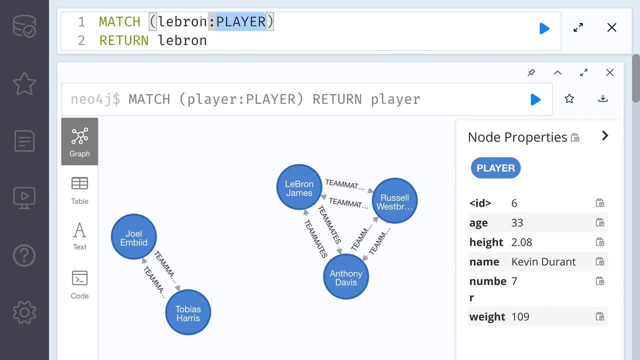 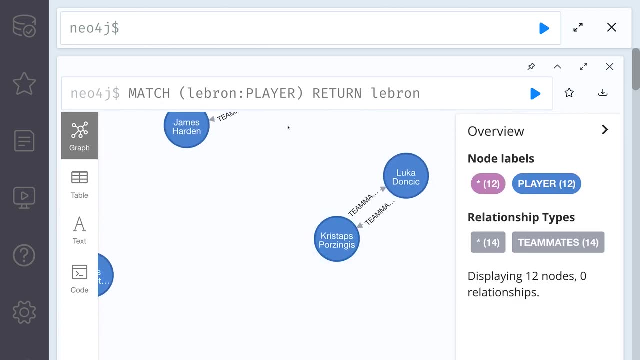 saying is: we want to get all of the nodes that have a player and we want to return it now, at this. at the end of the day, what this is going to do is just return us every single node that has the player label. of course, this is not what we want. so what we want to do is we want to get. 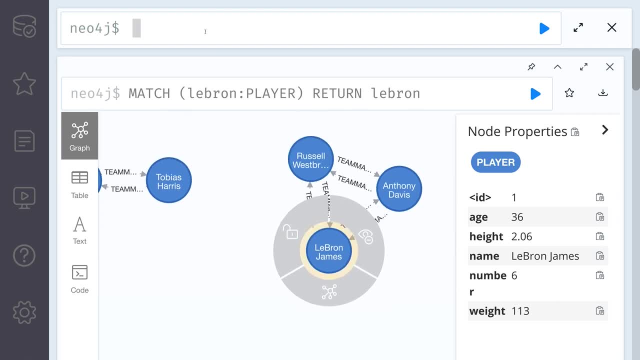 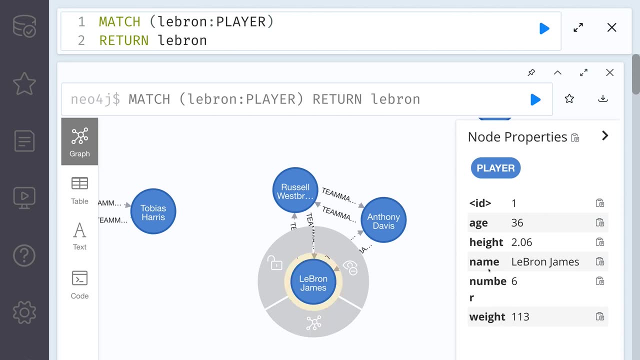 just a lebron node. so, in order to do this, what we need to do is start filtering out for this node based on some of its properties. so the best property that i think of utilizing is the name, because it's going to be unique across every single individual. now, if we have a large database, 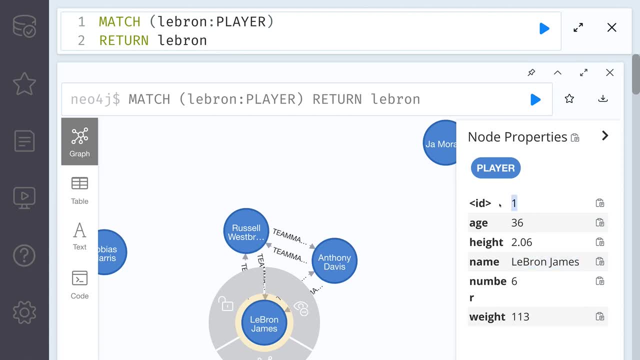 maybe there might be two lebron jameses, so maybe in that case we could use the id, but i'm going to use the name. so how do i filter for all of the nodes where the name is lebron james? well, it's actually pretty easy. so in between the 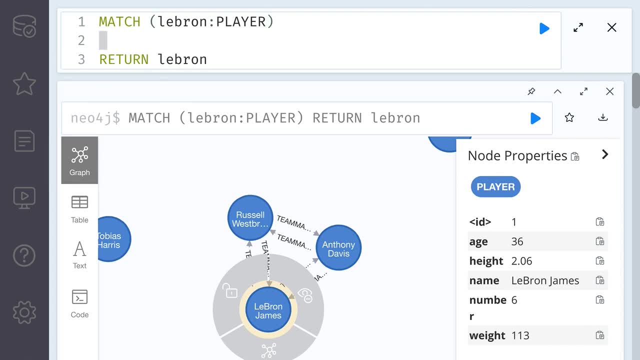 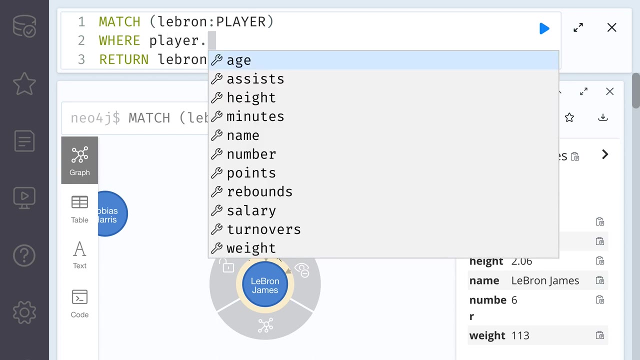 match and the return. what we're going to do is we're going to do another shift, enter, and then here we're going to say the keyword where. so we're going to utilize this in order to filter for specific nodes. so we're going to say where, and then we're going to say where the player, or sorry. 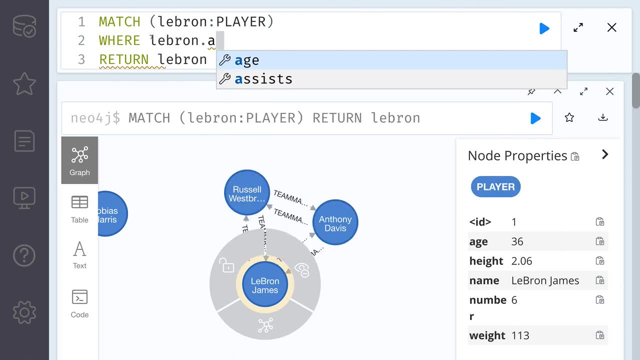 where the lebron dot name, and maybe over here what we can do is we can change this to player, just so it makes a little bit more sense. so we're going to say player and then over here we're going to say where the player dot name and we're going to say where the playername is equal. 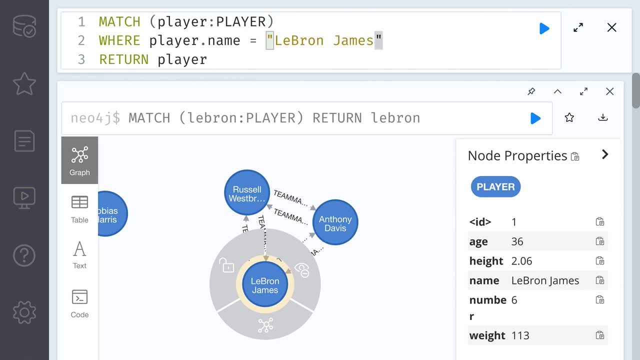 to lebron james, and the capital case is really important. we can't just have something like lebron james or whatever. make sure that that the capitalization is correct, because cypher detects this. so, because there is a difference between this and this, just to let you know. so now what we can do is we can execute this query and now all we get is 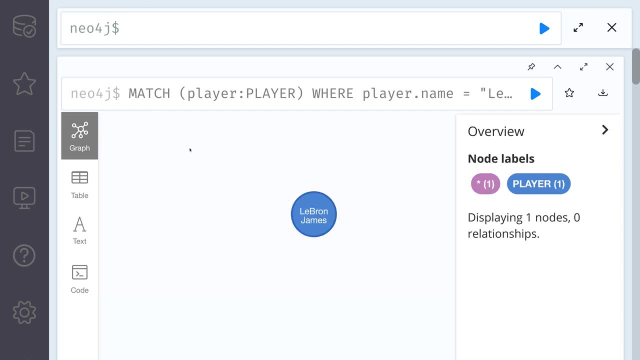 lebron james. how awesome is that. and, of course, now we can click on it and see all the properties. one thing is: right now we're getting the graph aspect of it and this is the visualization, but when we actually get our data back inside of our application, it's going to look a little. 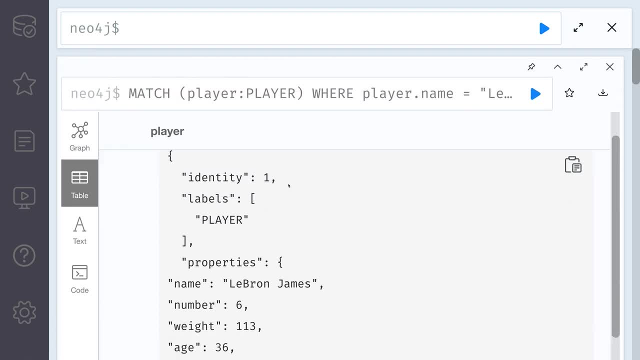 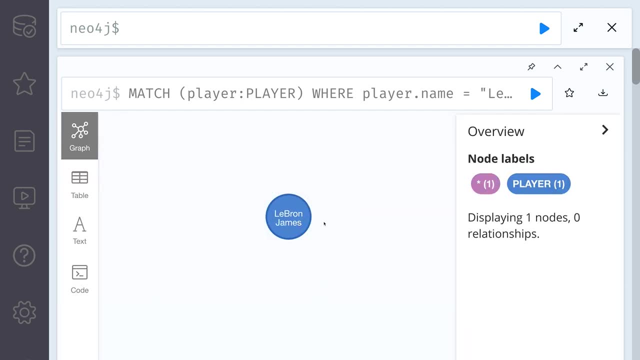 something like this. so it's going to look something like this, but this is again representative of a node. all right, cool. so that is how we can do the first filtration. now there's actually another way we can do the exact same thing. so, instead of doing the where clause just like we did here, what we can do is we can. 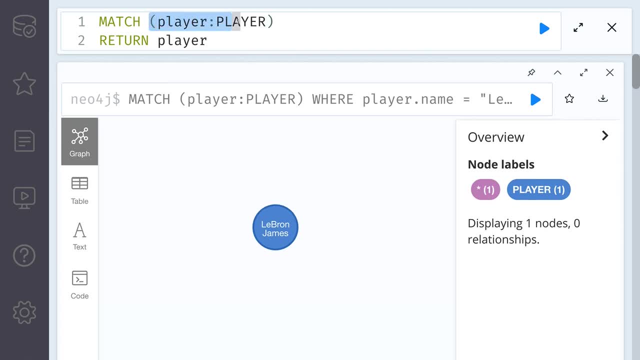 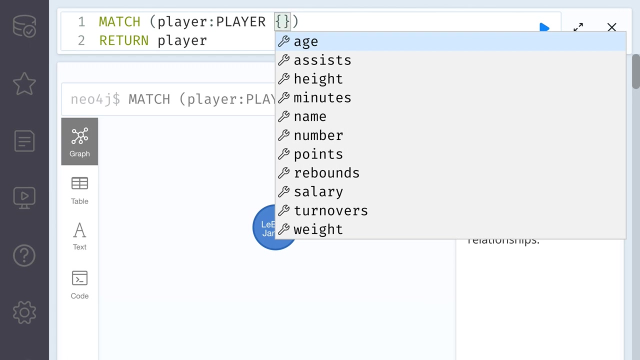 get rid of this and then, inside of this node, what we can do is. what we can do is we can say space, space, oh my goodness, space. and then we can add these curly braces and then, in here, what we're going to do is we can have a key value pair system, so we can say here name, and then here: 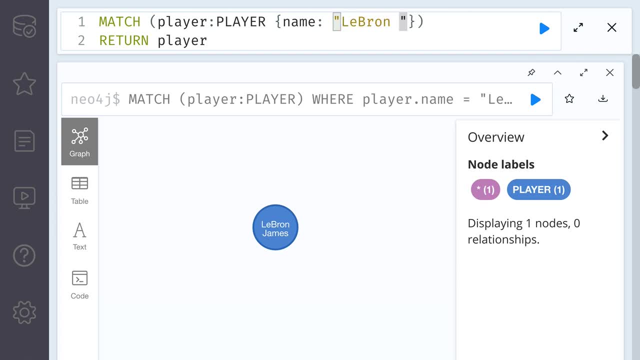 we can say lebron james, and this is going to do the exact same thing. what this is going to do is is going to filter for the player where the name is lebron james, so we can go ahead over here and we can execute this and, of course, for both commands we can have multiple, multiple, different. 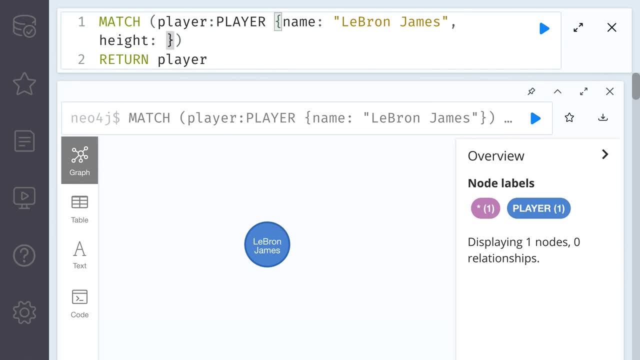 things over. here we can say lebron james, and we can say here, height is two point, zero, zero point. the response option nice and simple. there are four command options according to this, which is called give, h and f, if and g, if This Lemon Raises the' 위에, you see the mirror. so that means we are going to. 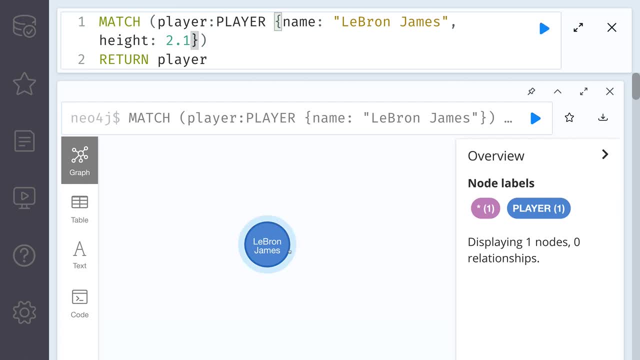 give h for h and f these commands. that makes it much easier when we're doing these commands. so that's point. I don't know one At this point. if I were to click on this, his height is 2.06.. So we should. 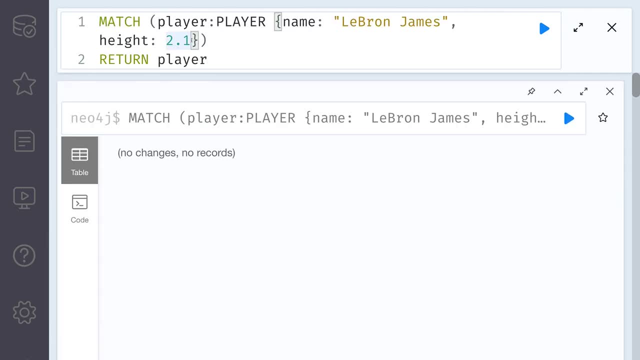 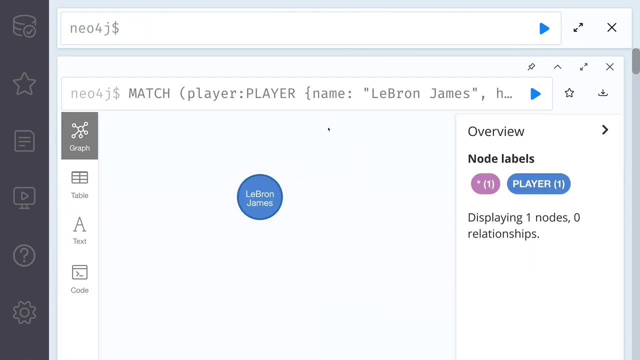 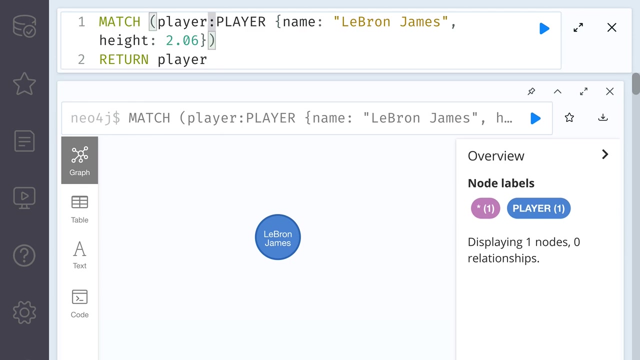 get nothing And we get nothing. However, if I were to change this to this, we should get LeBron back. Let me do. All right, cool. So that is how we can filter for specific things, But well, maybe this is not enough. Maybe we want to get all of the players that are not named LeBron James. 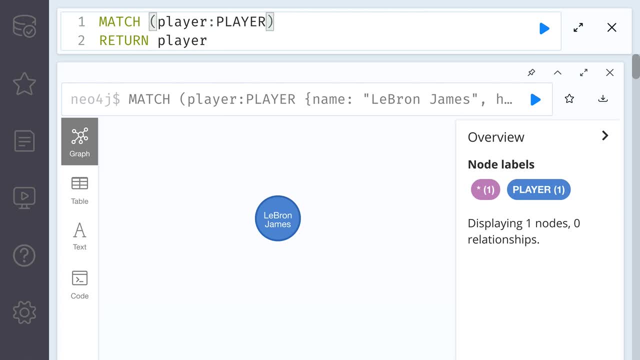 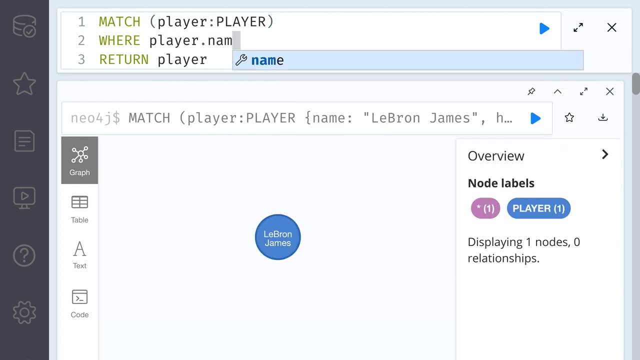 So let's actually go back to the where. So we can say here, where we can say: player dot name is equal to LeBron James. So that's what we had before, And now what we want to do is we want to query for the players that are not named LeBron James. In order to do this, what we can say is: 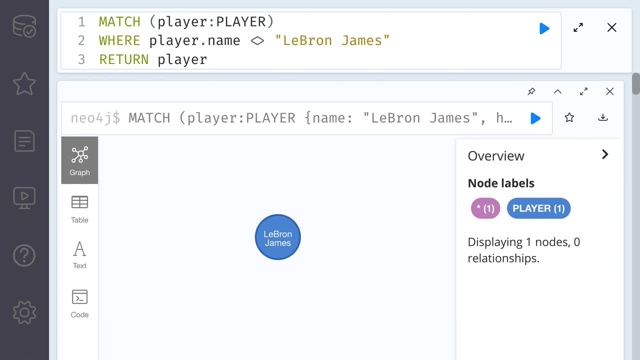 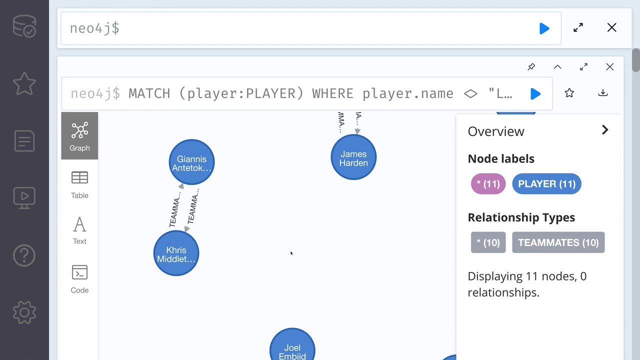 instead of having equal, we can have two square or two triangle brackets over here. This is just simply saying that I want all of the players where the name is not equal to LeBron James, And so if you were to execute this, you can see: here we got Kevin Durant, James Harden, Giannis. We get absolutely no LeBron. 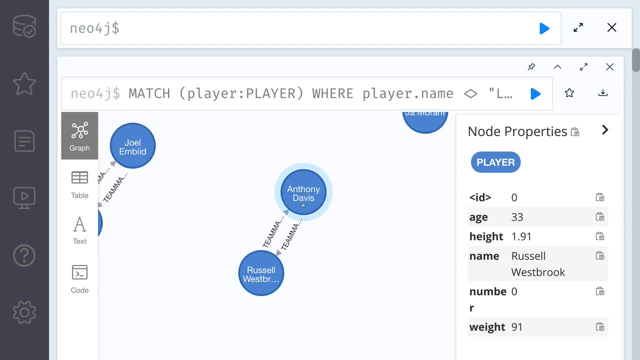 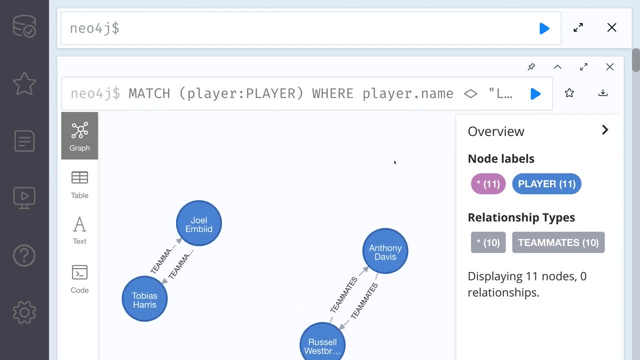 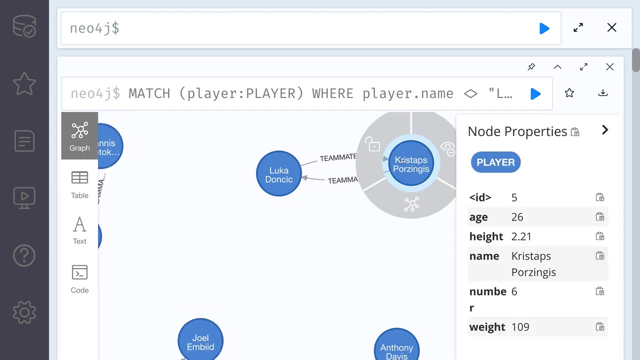 James. So, over here, LeBron should be here because he's teammates with these people. Okay, cool. So the next thing that I want to teach you is some other conditions. So maybe now we want something more reasonable. Maybe we want to query for NBA players based on their height And we want 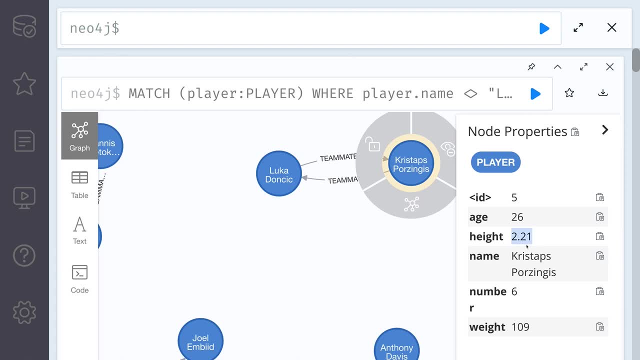 to see all of the players that are not named LeBron James. So let's say, we want to query for the players that are taller than two feet, So sorry, not two feet. Well, I hope that every NBA player is taller than two feet, but taller than two meters- And, honestly, I'm in Canada. I use feet in inches. 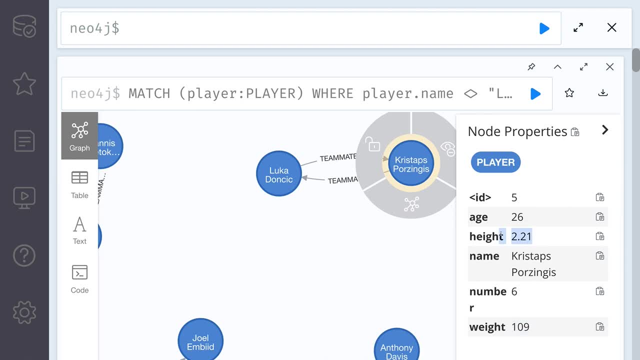 And then I also use pounds instead of kilograms, But when I search for these players on Google, it just shows me them in meters and kilograms, So that's what I'm utilizing. All right, so we want to get the players that are taller than two meters. So, in order to do this, 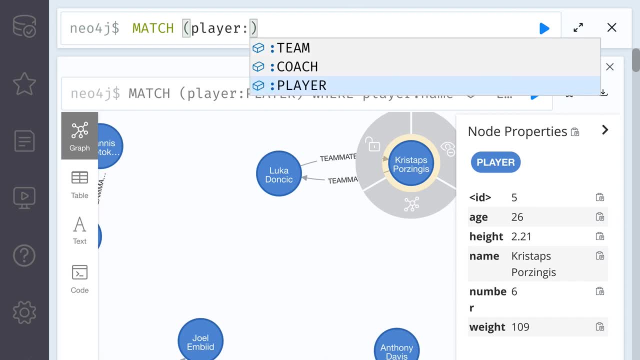 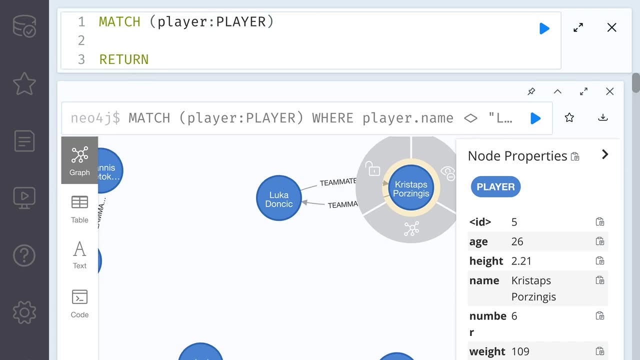 we're going to say match, we're going to say player, we're also going to say that we want to get the, the player label, And then let's go over here And let's just say return player. And then in here we're going to have a where clause. So in here we're going to have a where clause. 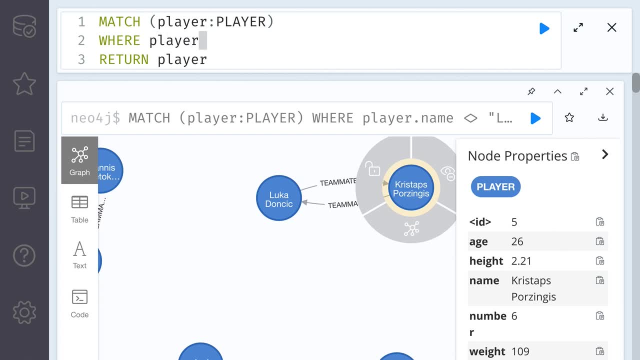 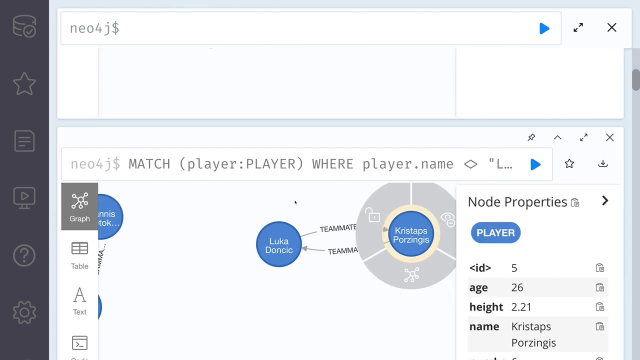 And then inside of this where clause, we're going to simply say where player dot height is greater than or equal to two. So if we were to execute this, we're going to say where player dot height this: you can see that now we don't have john morant. i think john morant was the only player. 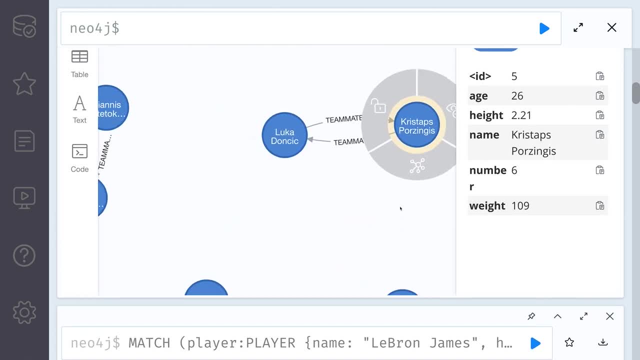 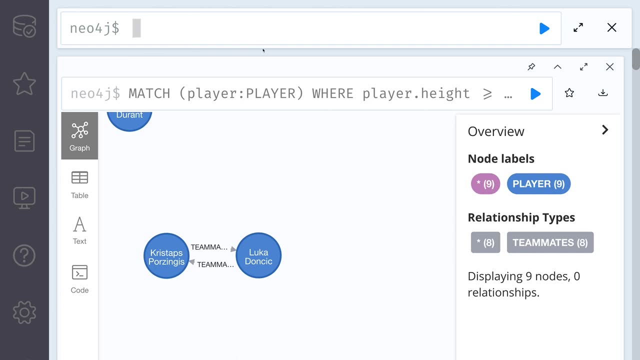 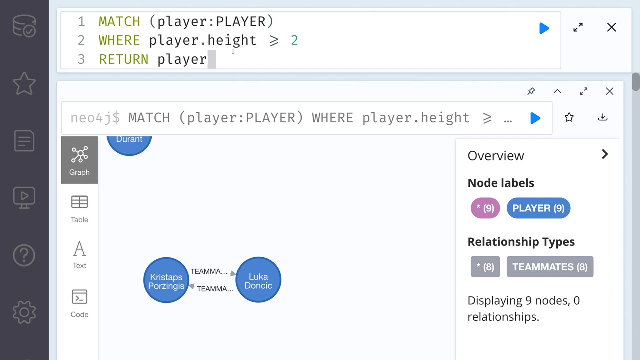 that was under two feet, and i think we don't have him at this point. okay, yeah, okay, cool. now we can, of course, do the same thing for any players that are less than two feet, so we can run this exact same query. and, by the way, what i'm doing to get this query back is i'm 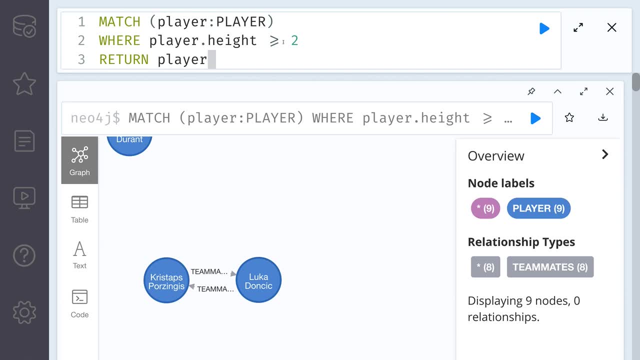 just clicking on this and then clicking the up keyword, and this gets me my query back. so now, what we can say here: we can get rid of that, get rid of this. we can say it's less than two feet, and if you were to execute this, oh, we get james harden, we get, we get a bunch of players. 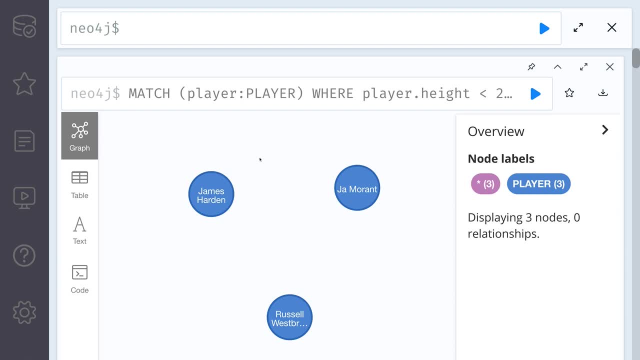 actually not just john morant. all right, awesome, and what we can actually do in here is do some arithmetic. so, for example, maybe i want to get um the players that have a bmi that is greater than 25, and if you don't know what the bmi? 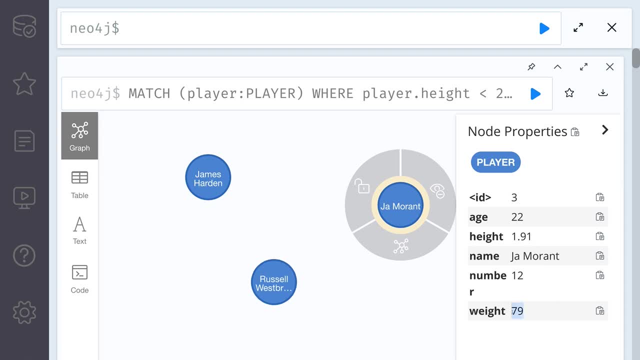 is. it is the weight of the individual divided by the height squared, and what it's supposed to do is just tell you if you're, you know, if you're obese or you're too skinny or you're just right now, a lot of these players are going to have a bmi that is greater than 25, which it means that, hey, they're. 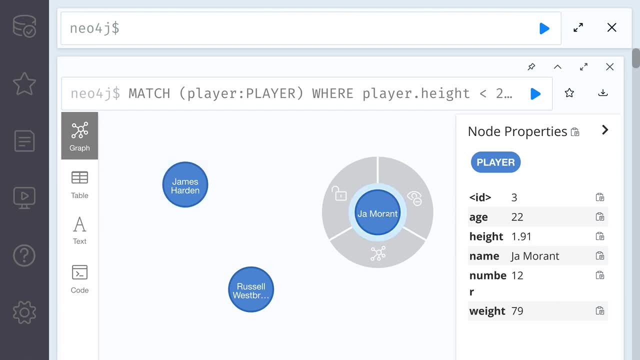 obese, but they're nba players and they're extremely muscular, so they're actually not that obese. but you know, let's just go ahead and calculate it. so over here, what we can say is: you can match player and we're going to say: player, colon player. 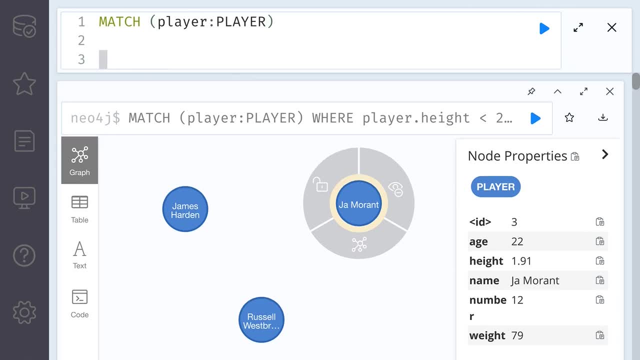 and then let's go ahead and just return the player and then in here. so in the where clause, in the where clause, what we can say is we can have a little bit of an arithmetic statement. so what we can say is we want to get the player dot weight and remember, we want to. 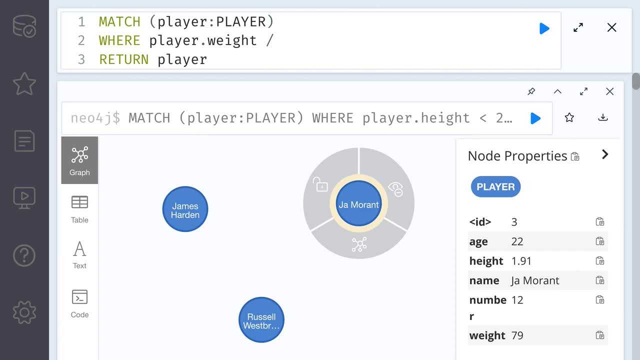 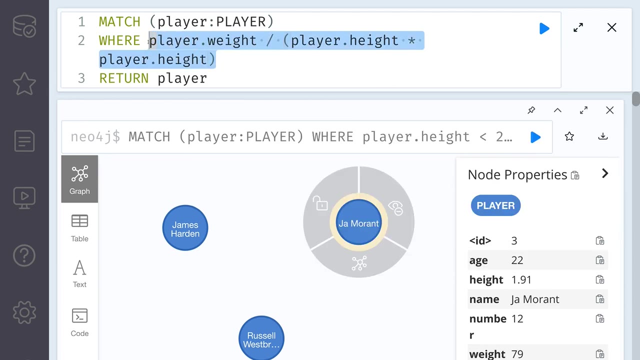 we want to divide it by, and we want to divide it by the player dot height squared. so what we can do here is player dot height and then over here times player dot height, and what we can do is we can actually wrap this whole thing in parentheses. 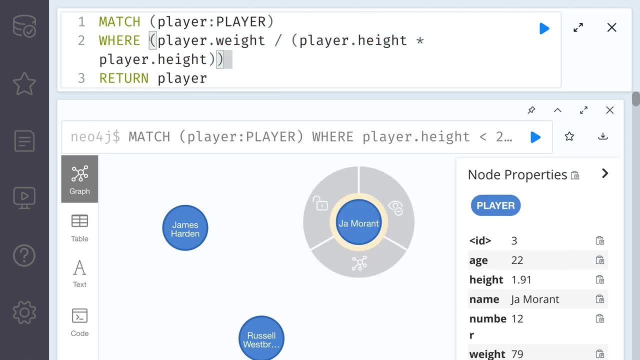 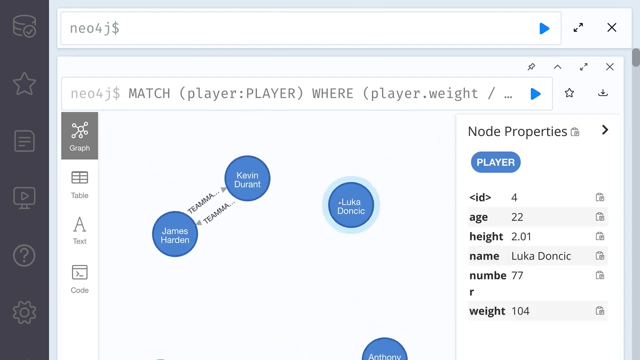 and we can say that this: we want this to be greater than 25, so we want to essentially do this calculation over here and then we want to filter for the players that have this be greater than 25. so let's go ahead and let's execute this and, of course, we get you know the heavier players. 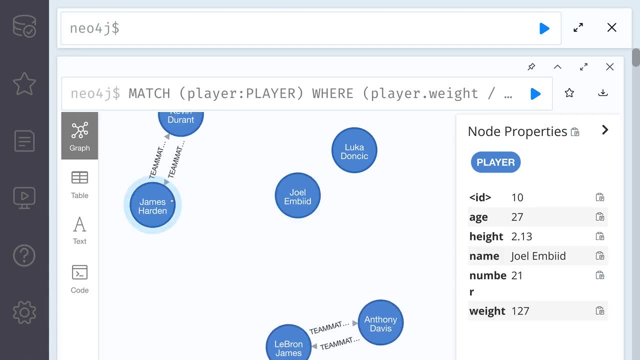 so luka donchic, we get you know. joel and bead, we get james harden. these three players are actually kind of considered almost out of shape all the time, so this actually kind of makes sense. and then over here, lebron ad and then kevin durant. well, they're just freaks of nature that are very 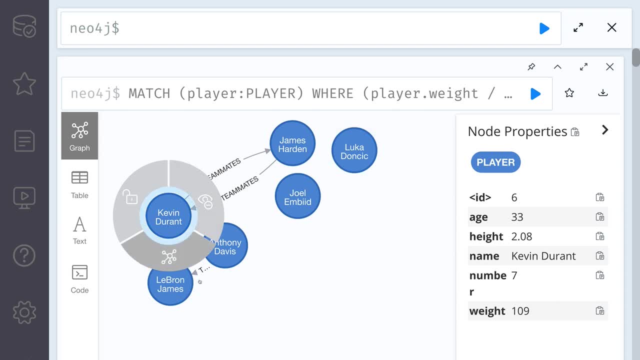 muscular. i'm actually surprised kevin durant is there, but these are very fit people, okay, cool. so we actually did the arithmetic correctly, okay. so now, one thing that i want to note is we have been querying for specific players based on one condition, so you know whether their 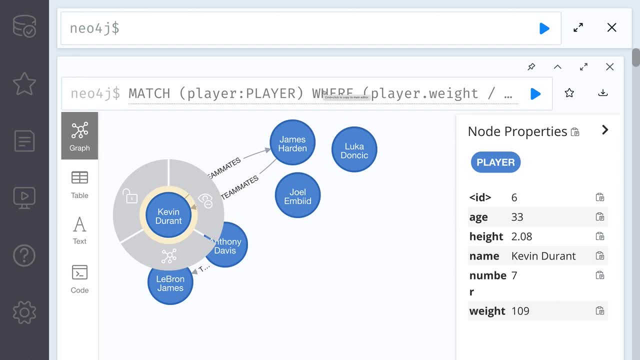 height is greater than two feet, or whether their name is lebron james or whether their bmi is greater than 25. but what if we have multiple conditions? what if, for example, we want to get all of the players that weigh more than 100 kilograms but are shorter than two meters long? how do we do a query like this? 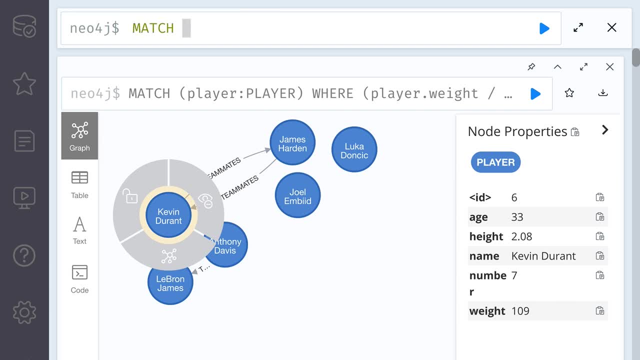 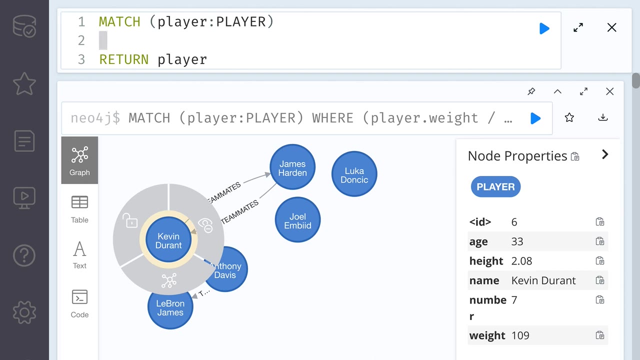 well, let's just get right into it. so in here what we're going to say is we're going to say match, and we're going to match, of course, player, we're going to say colon player here, and of course let's just have our return. we're going to return this player, the player nodes, and over here what we 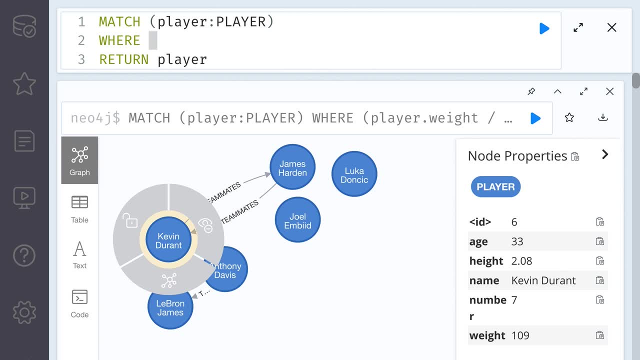 want to do is: we want to make sure that these players are also under two meters long. so, in order to do this, what we can do to to add additional conditions. what we can say is: and so you can say: we want the player to be greater than 100 kilograms, and we want the player to be greater than 100. 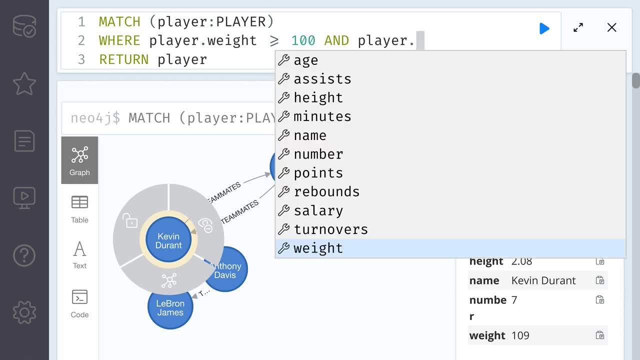 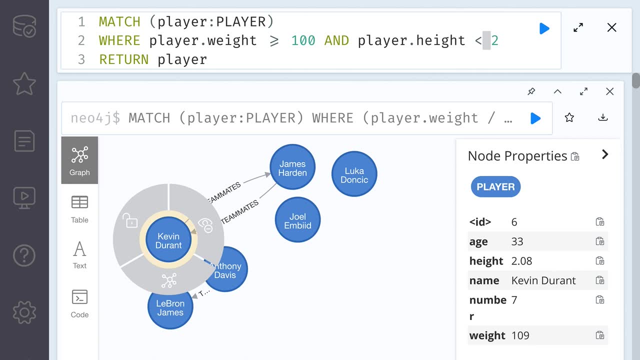 kilograms and we want the player to have a height that is less than two meters. we can say less than or equal to and, by the way, in order to show you what i'm doing here, i'm doing less than and then the equal sign, and what this is doing is just simply changing the- uh, changing the syntax, but 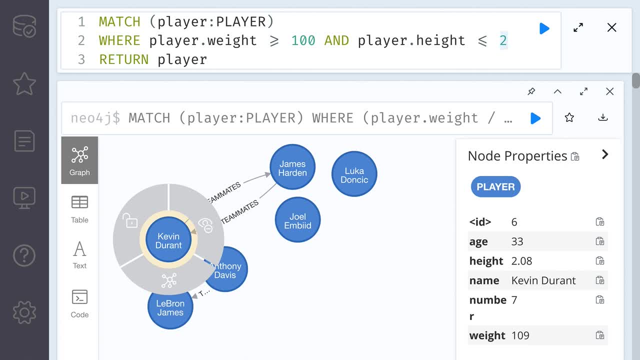 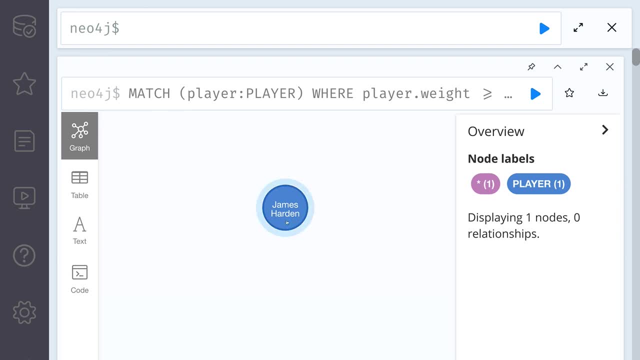 that's exactly what i'm doing here. okay, cool. so if i were to execute this right now, all i get is is james harden. james harden is the only person that is under two feet and weighs, you know, equal, more or equal to 100 kilograms. all right, and that is exactly how we can do multiple conditions. 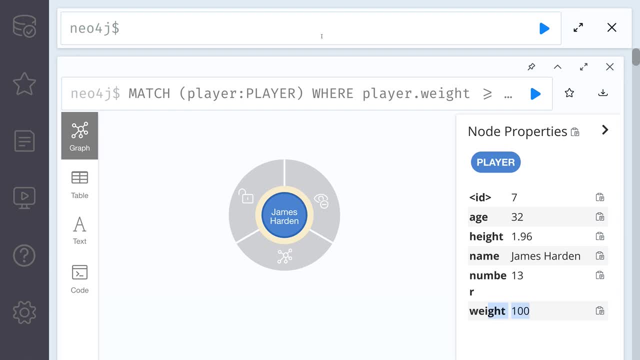 now, of course, what we can do is we can do the um, we can also do a or clause. so maybe we want to get all of the players that weigh more than 120 kilograms, or all of the players that are taller than 2.1 meters, so we want to kind of get the first one of the players that are the same. 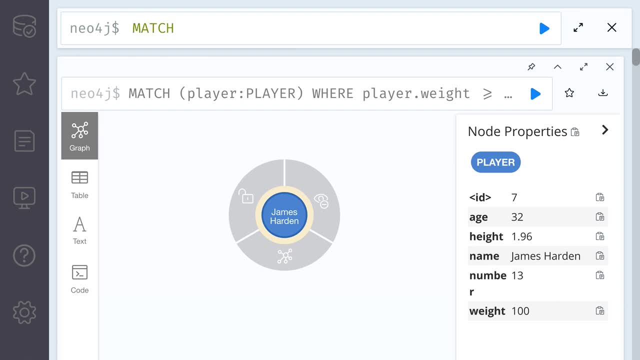 weight as the other players. so that means that we can say all of the players that are bigger than 120 kilograms or all of the players that are taller than two point one meters. so we want to kind of get freaks of nature. so what we can do here is we can say match player. 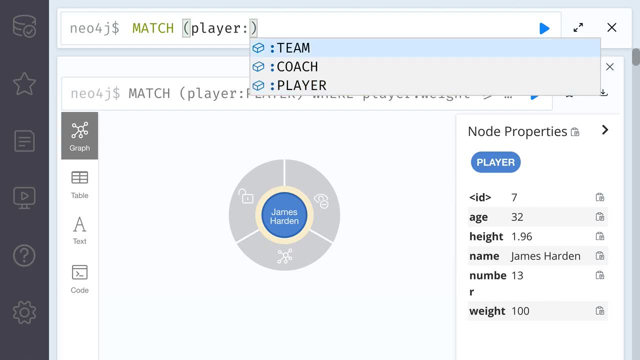 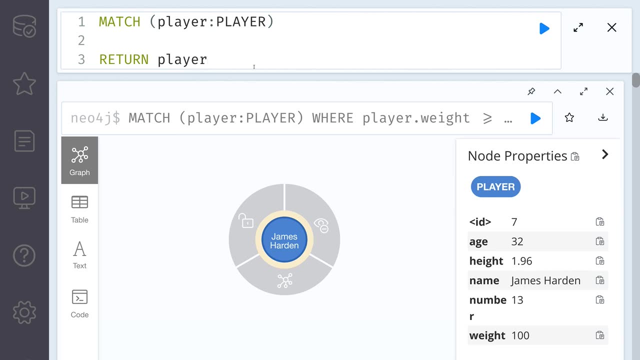 match player. and then we're going to say we want a player, and then we're going to say: return player, and what i'm going to do is i'm just going to copy this command, because it seems like we always write this out, and then in here we're going to say where, and then what we want here is: we want all of the. 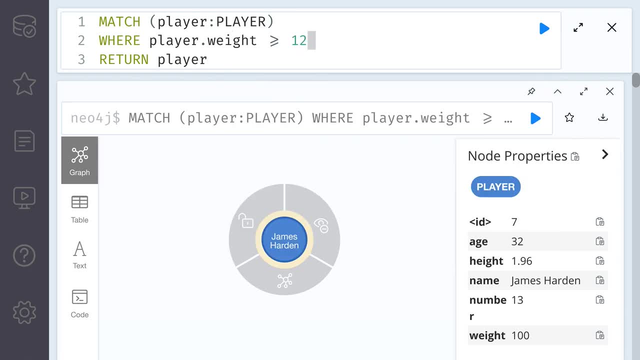 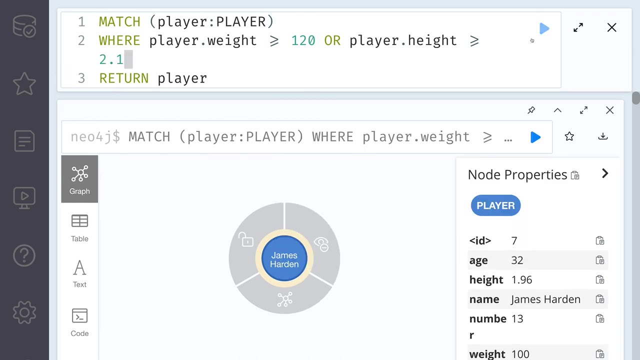 players that are way more so, greater than or equal to 120, and then we're going to say, or the player's height is greater than or equal to, and we're going to say 2.1, and this is just going to get us. you know, the freaks of nature in the nba. if we were to execute this, we get joel and bead, who is well. 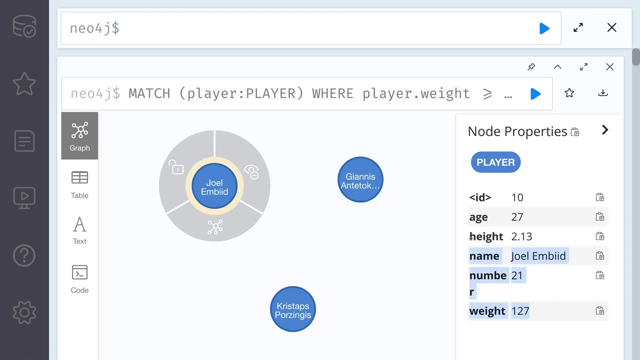 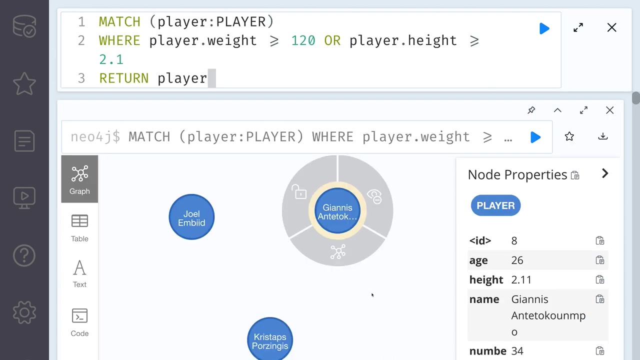 more than 120 and the height is this, so he actually matches both conditions. you get yannis, you get chrisapps, i think that's that's it. it seems at this point, uh, all the players that we get back actually match both conditions. so maybe if i were to change this to see: this is chris taps, so maybe if i were to. 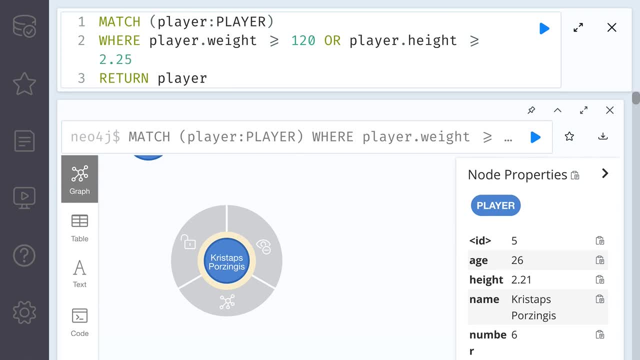 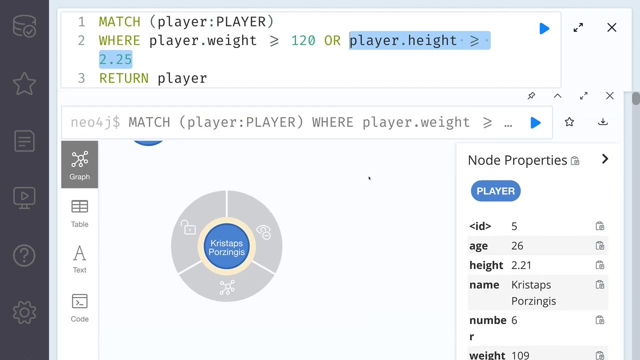 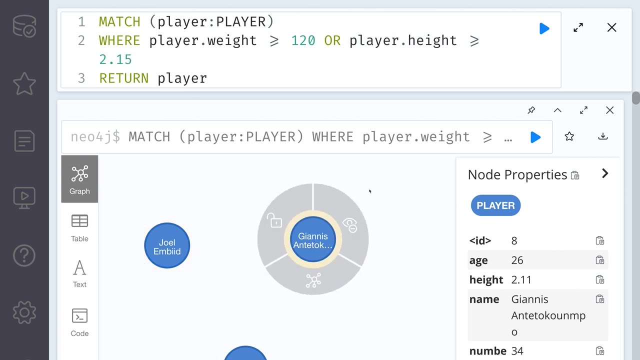 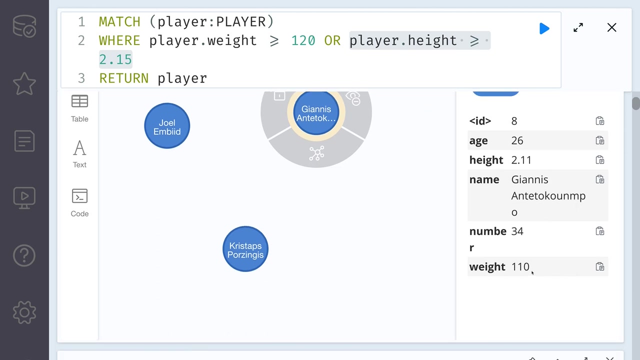 change this to something like 2.25. so at this point, this condition over here is going to not match. actually, wait, yeah, so actually, maybe, if i change this to like something like this: 2.15. so at this point, yannis attiticumpo, he's not going to match this condition, however, he is. 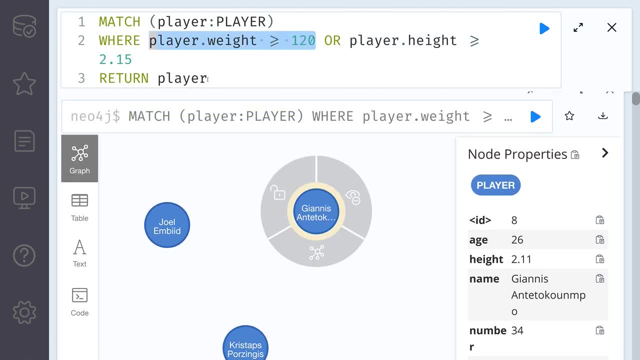 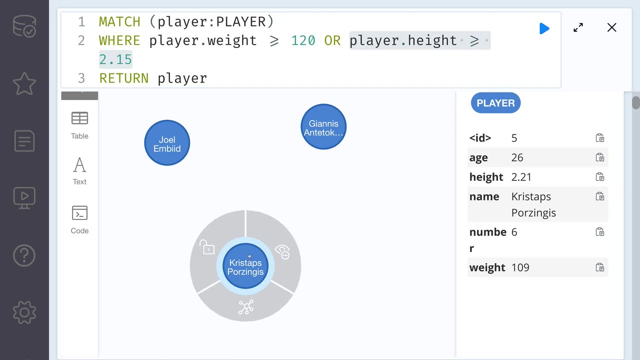 going to. well, he's going to also not going to match this condition, yeah, so this is actually a perfect example. so yannis doesn't match the first condition, but he matches the second condition, so he's in here. same with porzingis: the only person that actually matches both conditions is joel. 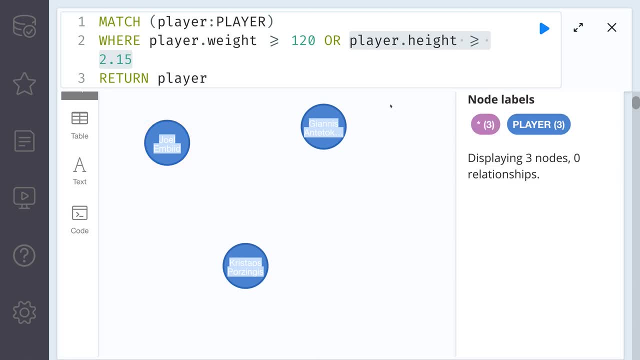 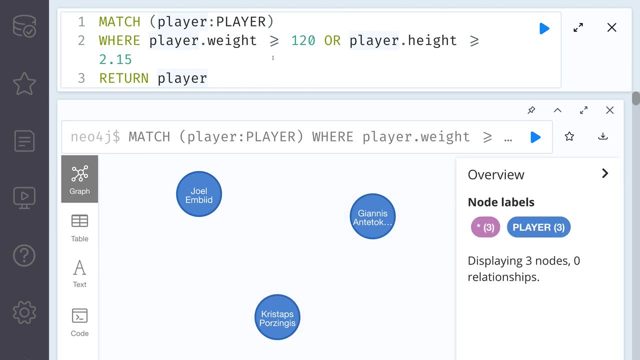 and beat and beat, get him back. of course, all right, awesome. but now what if we wanted to get all the players that did not meet this condition? well, in order to do this, what we can do is we can just flip these arrows instead of saying greater than or equal to. 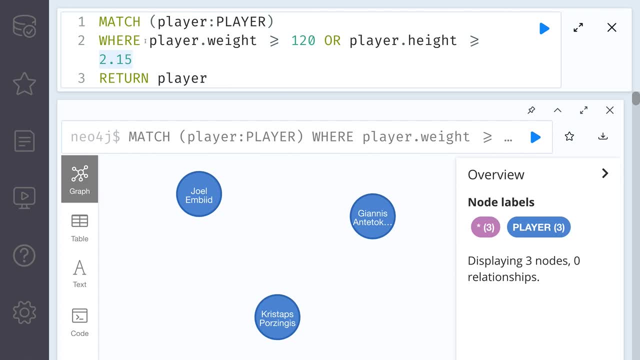 we can just say less than, and over here less than as well, but instead what we can do is we can say not. so what we can say is: here, where not this condition, so where they don't meet this condition, and at this point what we should get back are all the nodes except for joel and bead. so if you were 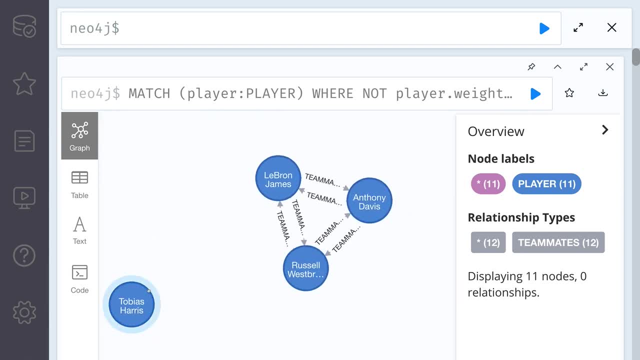 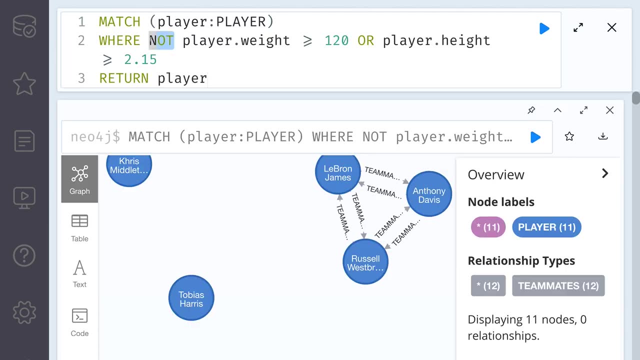 to execute this. you can see here, we don't have joel and b to buy his hair, doesn't have a teammate, and so remember, the knot is just how we can flip things. if we wanted to do that, all right, that's awesome. so what's the next thing that we want to learn? well, right now, what we're doing is we're 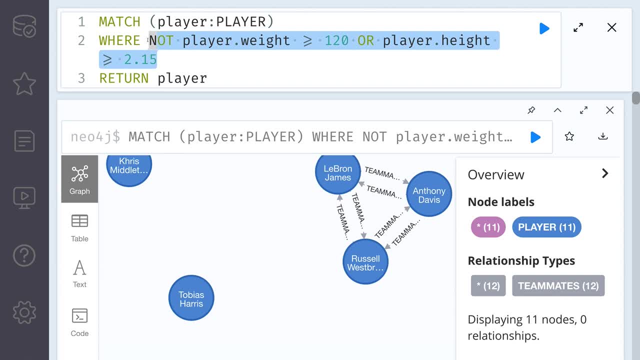 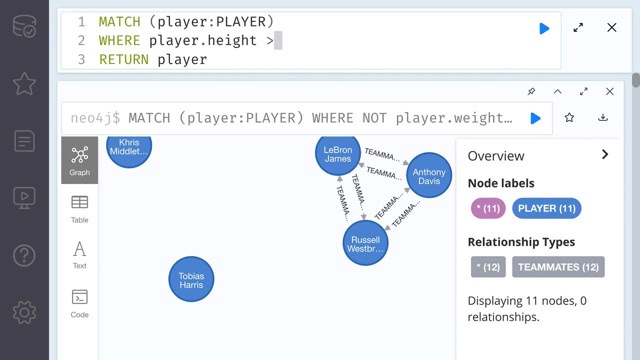 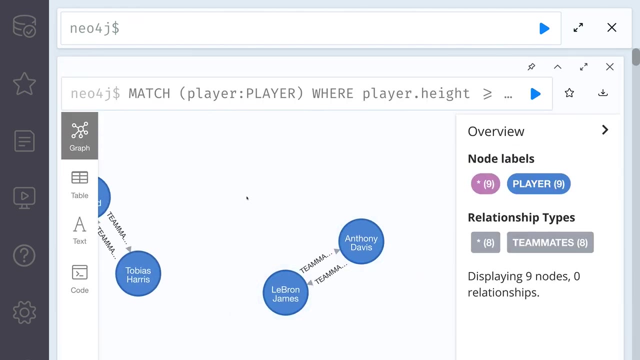 getting back a lot of players. so let's go here and let's just say: where player dot height is greater than or equal to greater than or equal to two, and we want to return all these players. and right now, actually, this is not at that many players. we have what? six, eight, nine players? but what if our 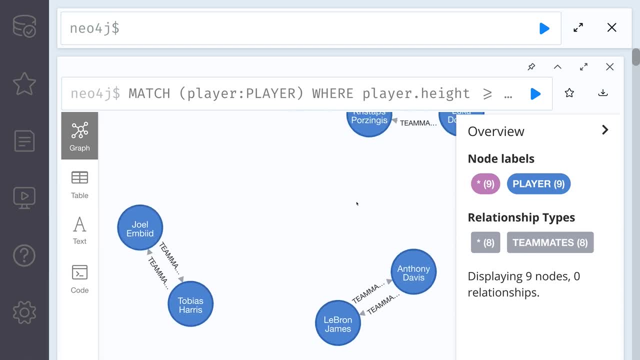 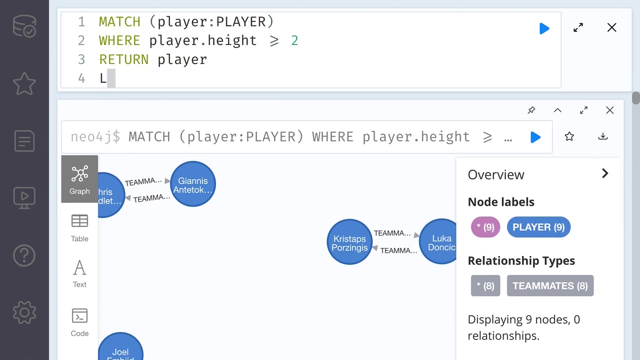 database is humongous and we're getting so many different players, maybe thousands of different NBA players- how do we limit it so we get, you know, maybe 10 NBA players? in order to do this, what we need to do is, right after the return, what we can do is we can say: 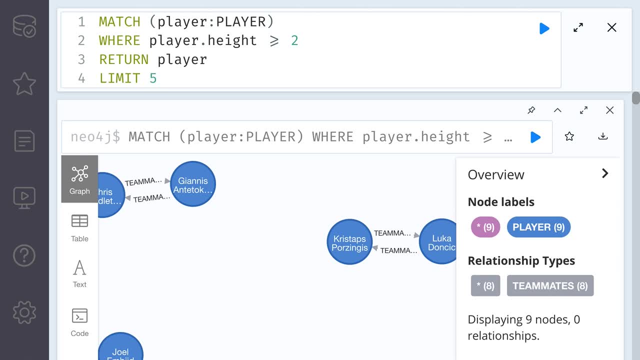 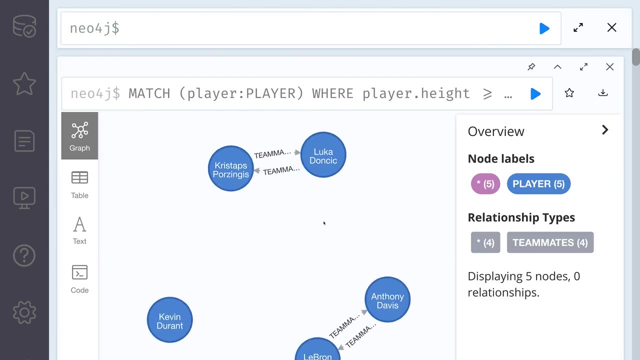 limit and then we can say limit well, however nodes we want to get. back over here we can say limit 5, which will give us five different nodes, and over here you can see, now we only get five nodes and we can actually utilize this if you want to do something like pagination. so instead, 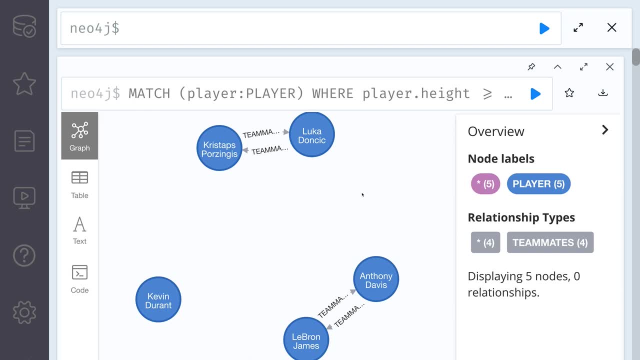 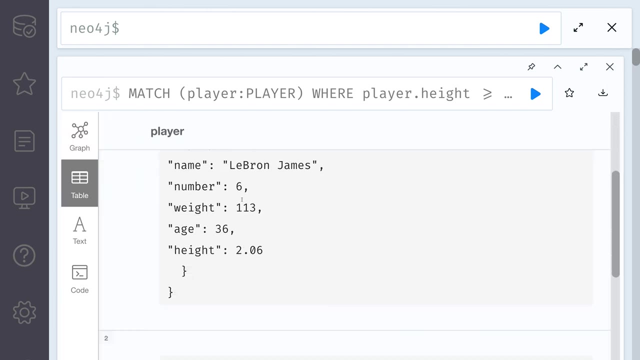 of getting all of the different nodes. we can say limit 10, show the first 10. if the person scrolls down some more, then we can show the next 10.. so, for example, let's just go back over here, let's just say limit 2, so limit 2, and what this is going to do is just going to actually give us 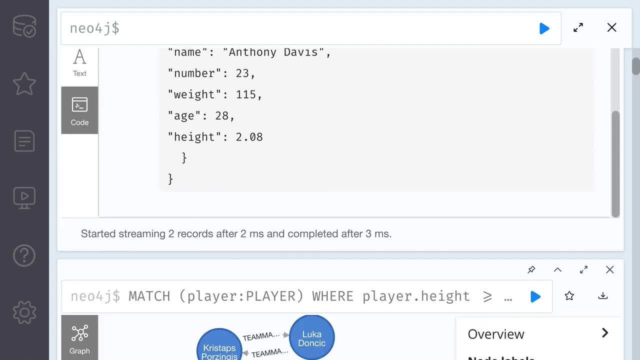 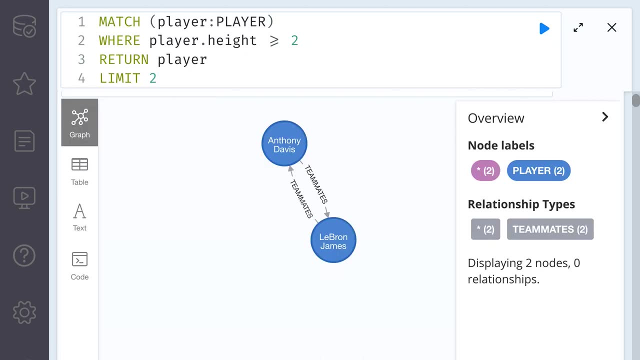 all the players in a particular order. so you can see here that we're getting Anthony Davis and then we're also getting LeBron James. so we get these two players. but what if maybe we wanted to get the next two players? well, what we can do at this point is utilize another keyword called skip. 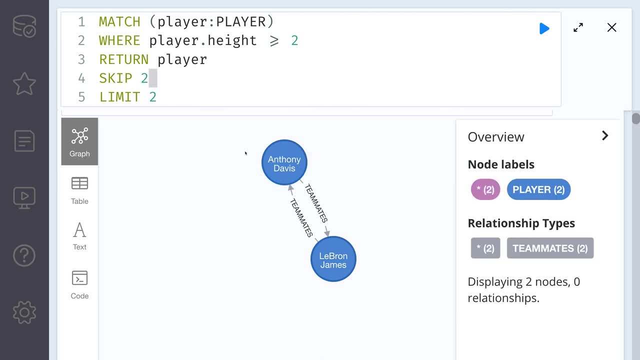 so we can say, hey, we want to skip the first two, we want to get the next two and of course we want to limit it to two. so we want to skip the first two and then get the just the next two. so at this point, if I were to execute, 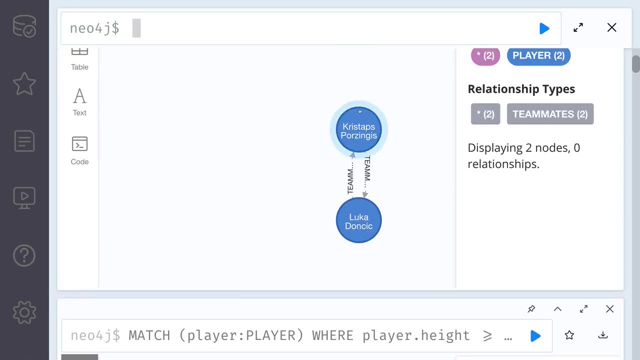 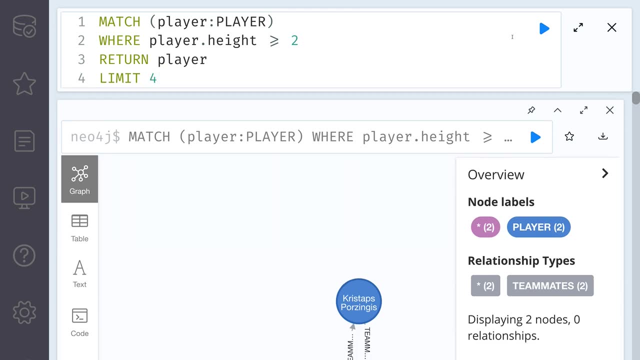 this: we don't get Anthony Davis and LeBron, we get Chris taps and Luca. and just to really explain this, let's get rid of this skip. and then over here we're going to say: limit four. so you can see here that we're getting back. if we limit it to four, we get back LeBron and Anthony Davis and 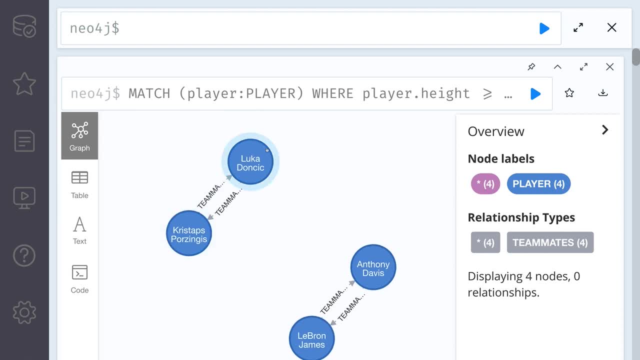 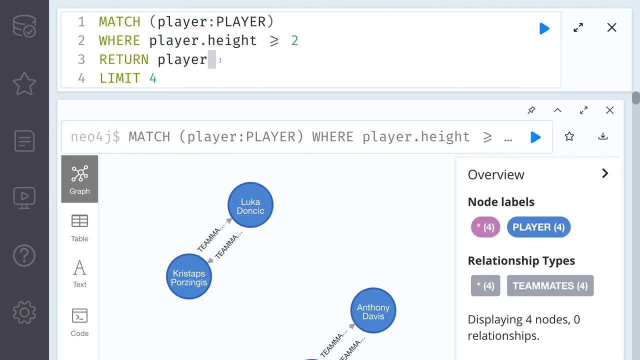 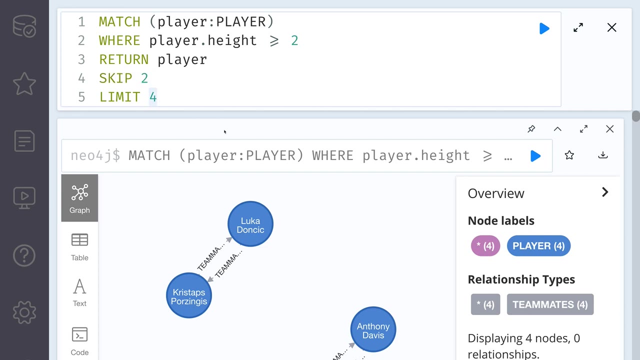 LeBron and Anthony Davis for the first two that we got back, and then over here we get back. the next two are Luca and Chris taps. so, essentially, what we're saying here is what we want to do is: well, we don't want to get the first two, which is uh, uh, which is LeBron and Anthony Davis. we want to. 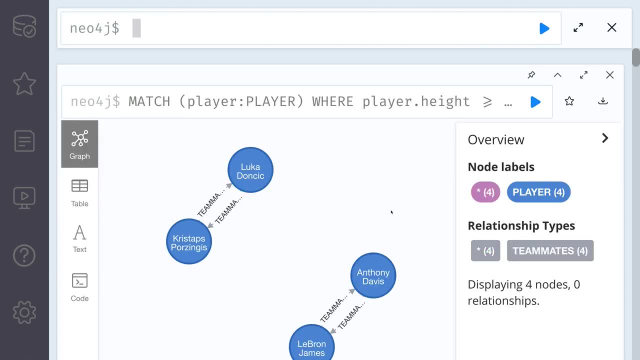 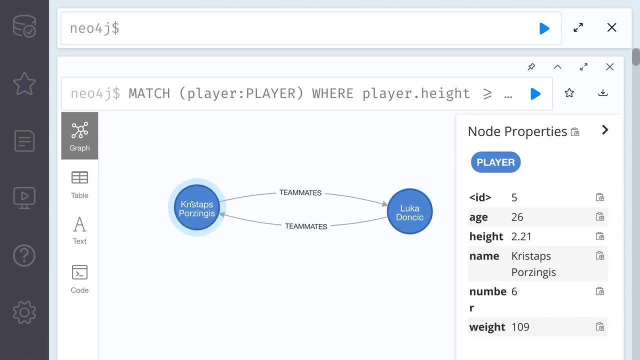 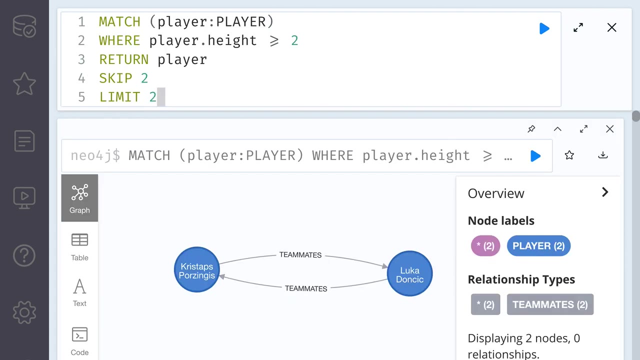 get the next two, because, again, we're limiting it to two. so if you were to execute this, again we get back those two players. so the next thing that we can actually do is order by specific players. so maybe what we want to do here is, well, we want to get all of these players and instead, 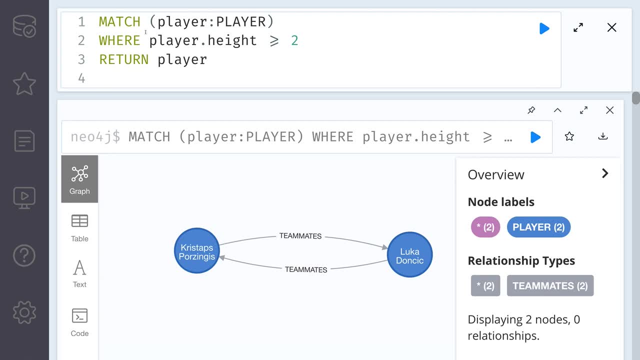 what we want to do is, instead of ordering by whatever their, whatever Neo4j is ordering these players by, we want to specify that we want to order these players by, maybe, their height. we want to get the tallest players first. so we're going to say order by player dot height and we 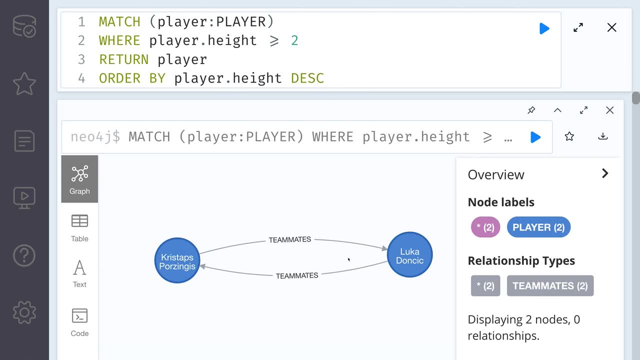 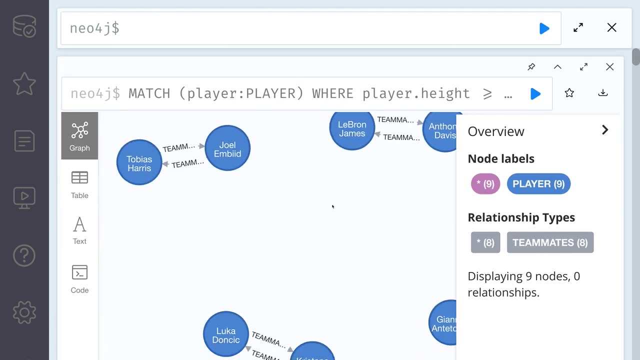 want it in descending order. so we start from the tallest and we descend down to the lowest. so if you were to execute this in the node format, it doesn't seem like it we're ordering them in any way. but remember, the node format over here is just showing us how the data is going to look, what we 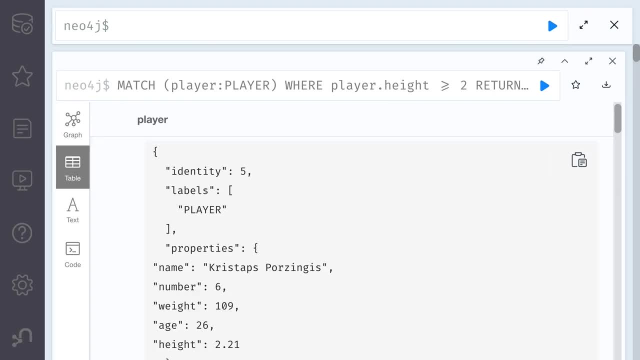 ultimately get back is something like this, and you can see here, if I were to zoom out, we get Chris taps forcing us first, who is the tallest player, and you can see here that now we're, you know, we're descending, we're descending. of course, what we can do is ascend so we can get the shortest player first. 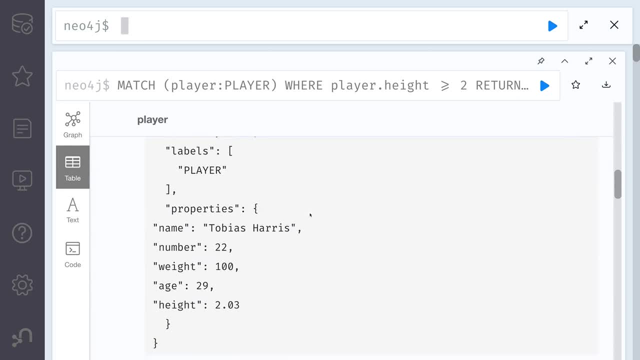 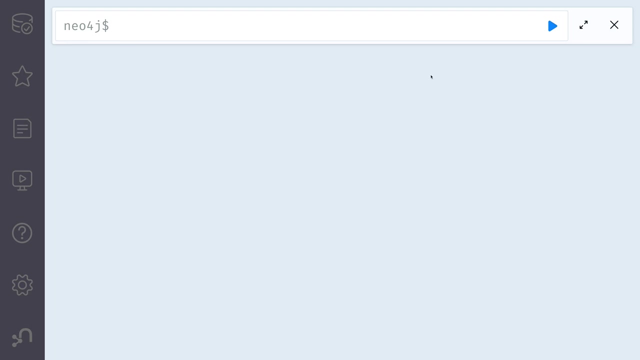 and at that point we get Luka Doncic and you can see now we're ascending. all right, awesome, and that really pretty much concludes filtering for notes. we've actually learned quite a bit as to how we can filter notes. the only thing that I haven't really taught to you is how we can filter. 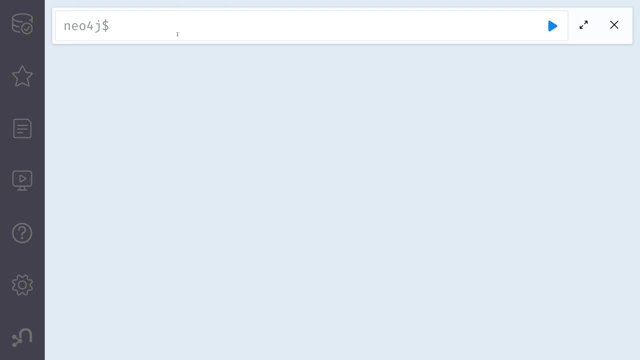 for multiple nodes at the same time. so, in order to do this, what we can very simply do is say match, and then we can say match, and of course we have these parentheses to specify that we want a player. so we're going to say player, we're going to say player, but what if we also wanted to get? 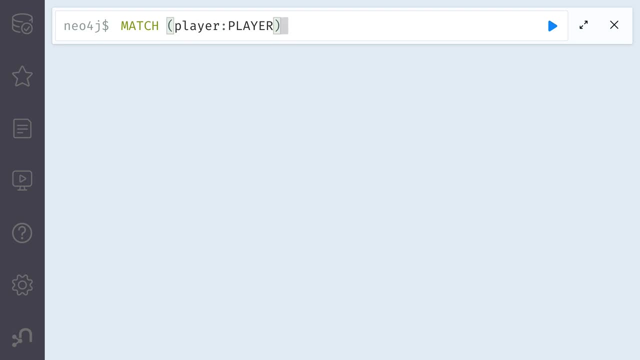 the coaches. in order to do this, all we have to do is say comma and then we say another set of parentheses because we want to get another set of nodes. so over here we can say coach and then over here we can specify that we want the coach label and then right down here we can return both the 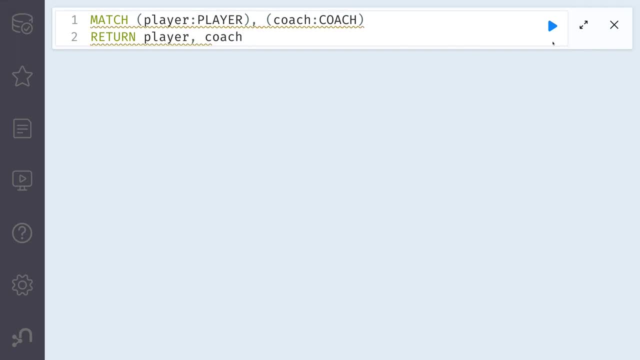 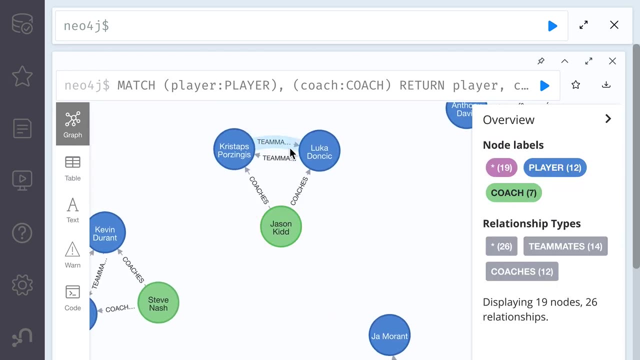 player as well as the coach, and if I were to execute this, if we were to execute this, you can see here now we get both the player as well as the uh as well as the uh coaches notes and we also get their relationships. now, of course, we can also add where clauses in here, just the same, so we can say: 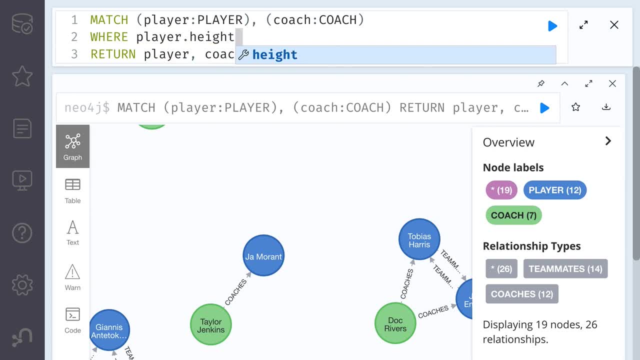 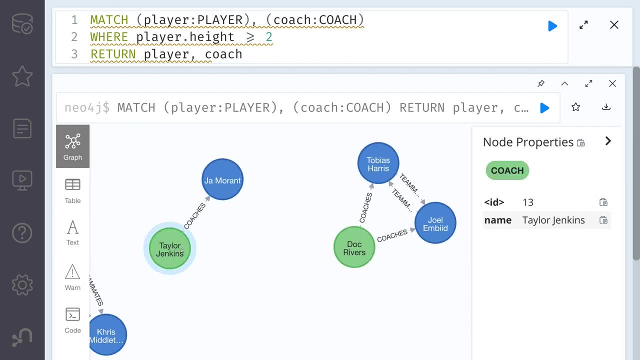 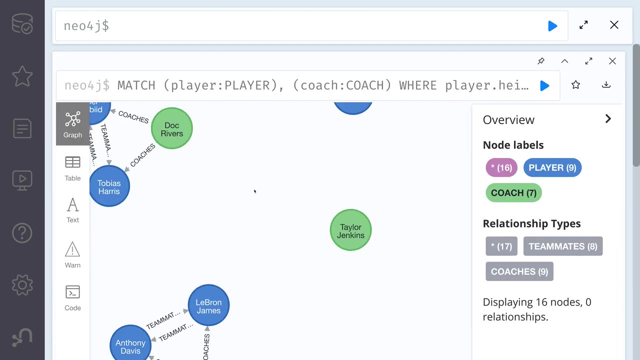 where the player dot height, where the player dot height is greater than or equal to two meters, and we can of course add additional where clauses for the coaches as well. so that's just something that you guys should probably know. so now we don't have the shorter. 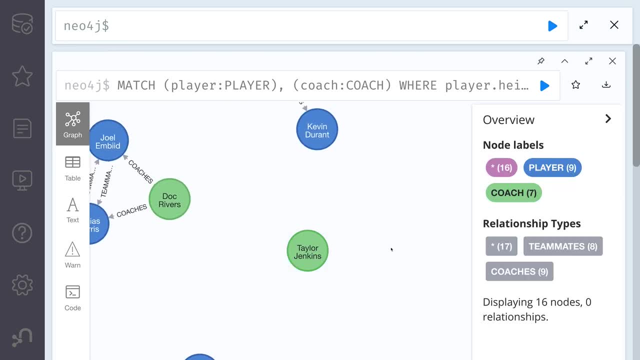 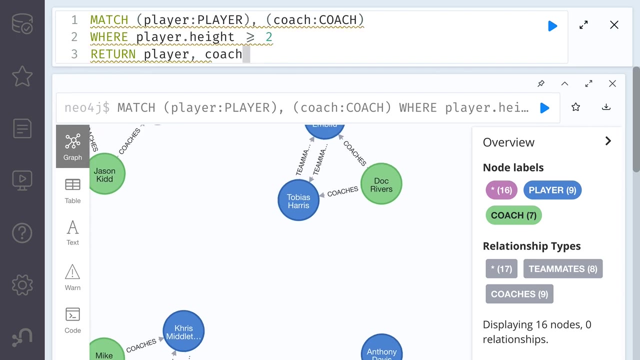 players. so, for example, Taylor Jenkins doesn't have his player because he's too short, and now Steve Nash only has one player because James Harden was too short. so I hope this is making sense and of course, I'm gonna highly suggest that maybe try to query for the team as well. 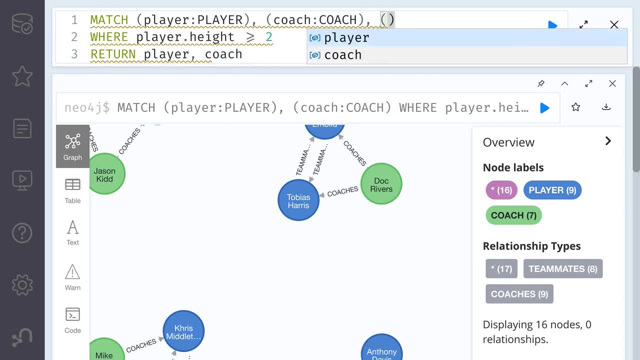 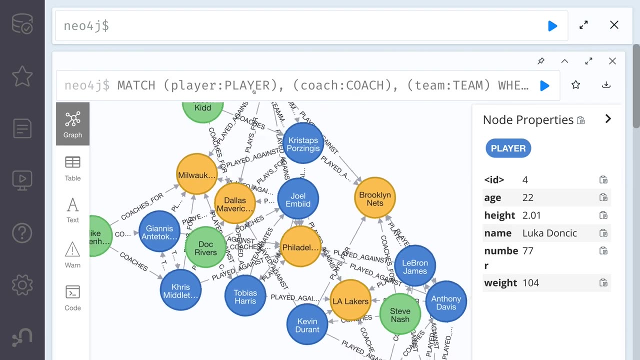 how could we go about doing that? well, we would go here and we would say team, and then we can say something like we can label it team and then over here we can just return team. at this point we get everything back. now this is looking very similar to what we had at the. 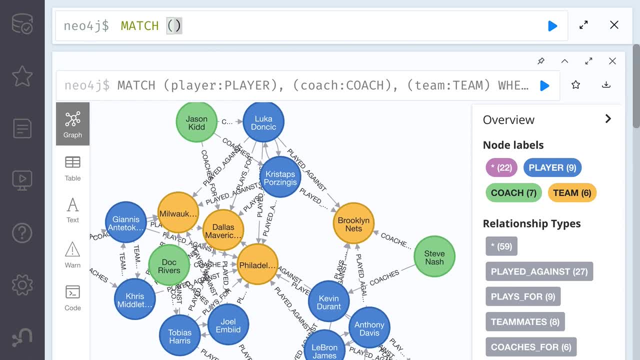 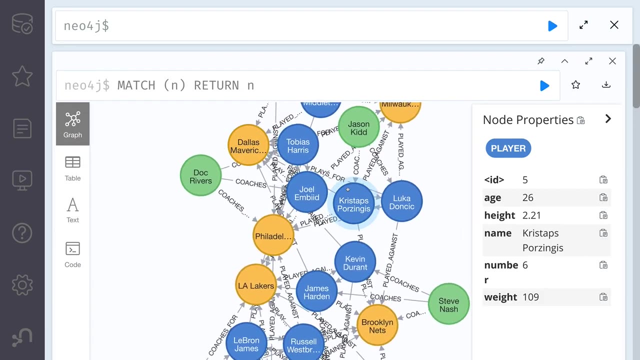 very beginning and remember we had something like this at the very beginning. so if we don't specify a label, we get all of the notes back, regardless of the label, and that is exactly what we did in the very beginning and that's what we got all right. cool. so the next. 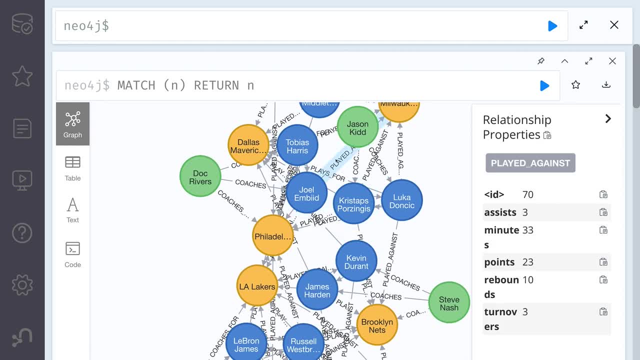 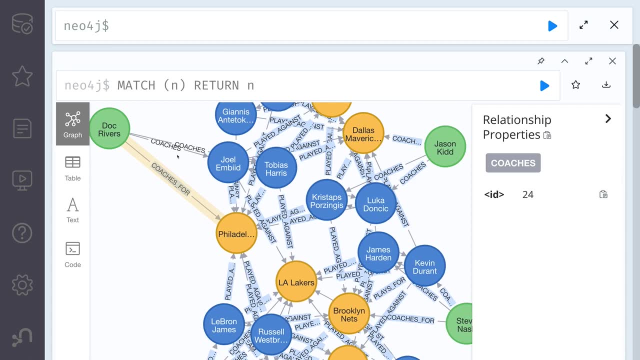 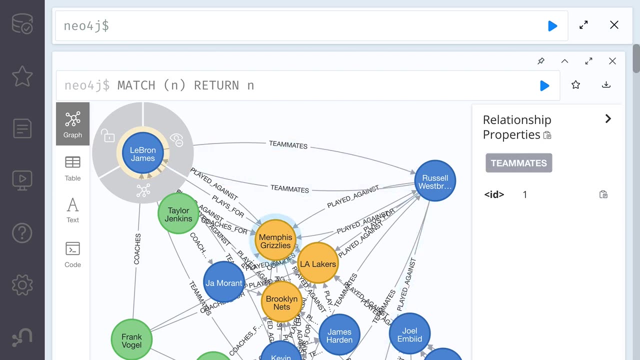 thing that I want to teach you guys is querying for relationships. so remember all of these nodes, have these relationships, and let's actually start querying for specific relationships in this section. what we're going to start doing is querying for specific nodes based on their relationship, and probably the best example of this is if we wanted to query for all of the players that play for a. 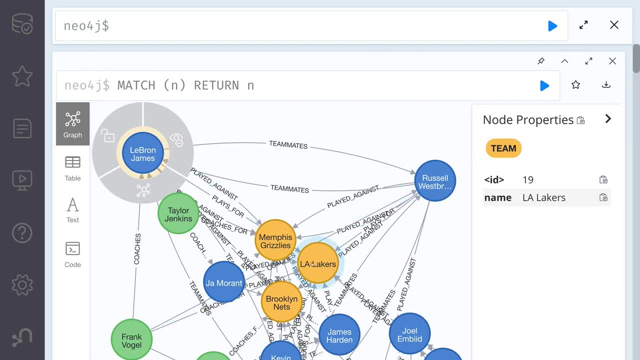 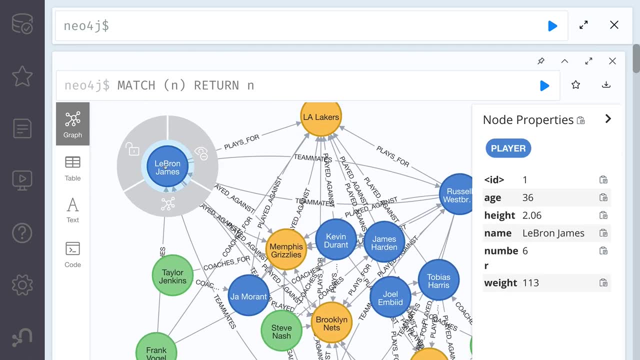 specific team. for example, maybe we want all of the players that play for the Los Angeles Lakers. now you might be thinking: okay, well, LeBron James, he plays for the Los Angeles Lakers, so maybe we can query for all the players based on their properties. but there's no properties that links LeBron James. 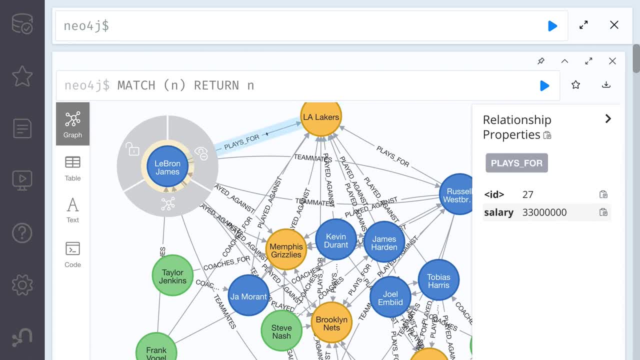 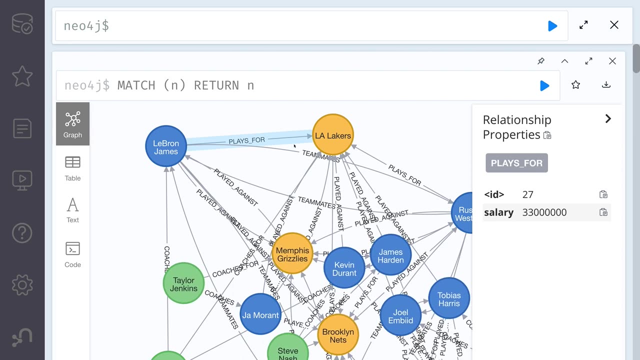 to the Los Angeles Lakers instead, this relationship right over here, it's the one that links LeBron to the Lakers. so how are we going to query for specific nodes based on their relationship? well, let's get into it. let's actually write a query where we query for all of the players that play for the Lakers. so the first thing that we have to 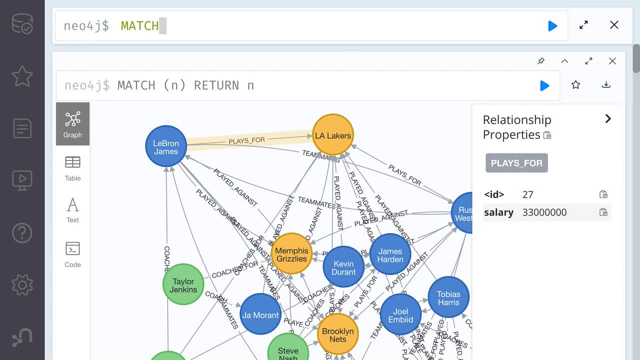 do is specify the keyword match. that is well, that's a given. we want to query. you always have to specify match and then we want to query for the player that we want to query for the player, that is, players. so let's say that we want the player nodes and let's specify that we want the player. 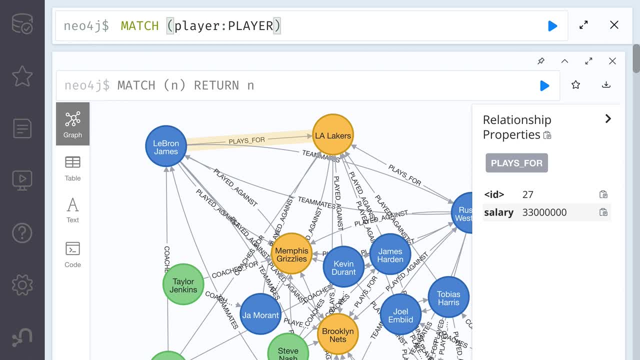 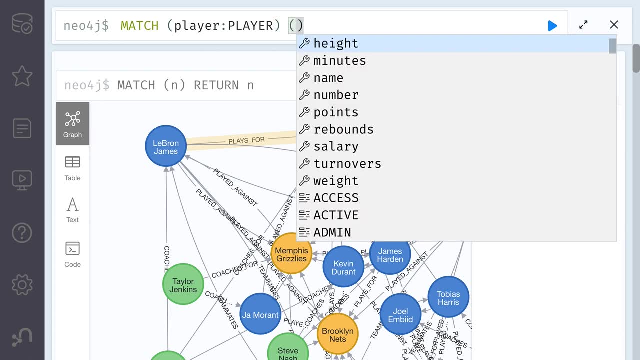 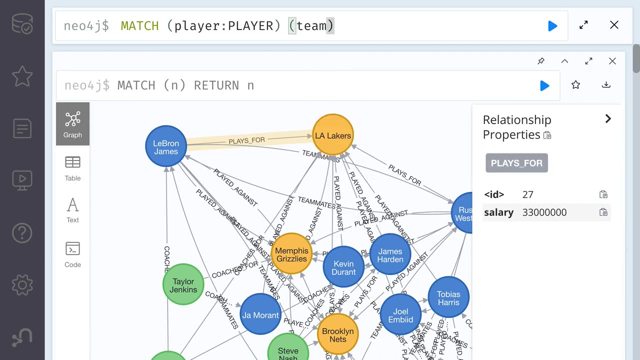 however, what we want is we want the players that play for the Los Angeles Lakers, and so really, what we need here is two nodes, and then this is going to be the team, and this we can label it as team, so we can, over here, say that this node is team, and we want to specify the relationship between these. 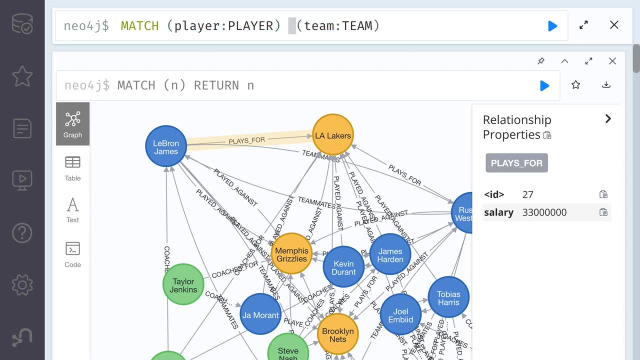 and we actually specify the relationship between these nodes with an arrow, so we do a minus sign and then square brackets, and then another minus sign, and then the- uh, the triangle, the right triangle, and over here what we're saying is we have this player node, we have this team node and 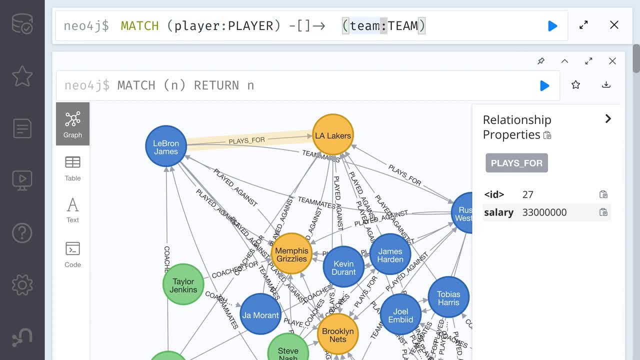 then we have this relationship between the player node and the team node and then inside of this square bracket, we can specify anything that we want. we can specify what relationship we can have, because over here, if I do colon, we have different labels for these relationships, like play for played. 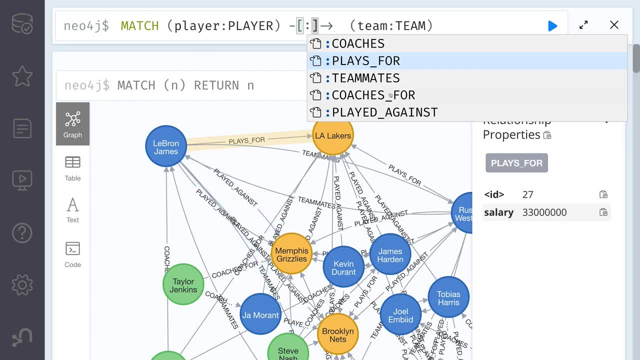 against played. whatever, we can specify exactly what relationship we want. in this case, we want the place for relationship. so this is how we specify a relationship. again, we have the player node and then over here we have the team node and over here we have this relationship and remember, this is going to be a minus sign, minus sign arrow, and then over here. 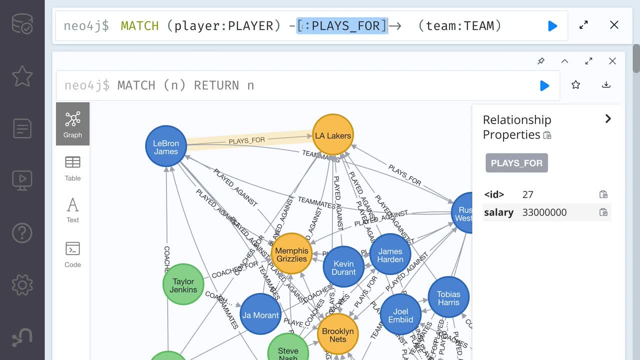 in the square brackets. we're going to define exactly what we need, and we can also call this whatever it is that we want. we can give this a very variable name, called relationship. so the other thing that I want to note is: remember this is one directional. a player has a place for. 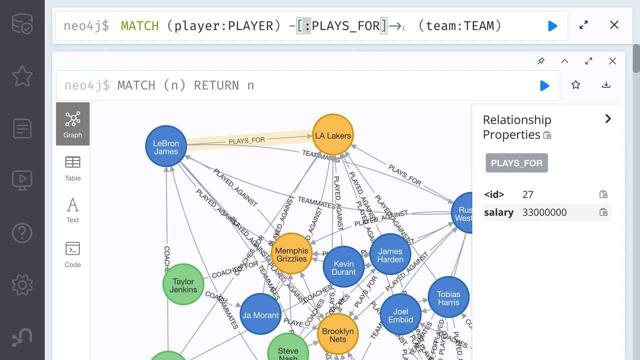 relationship with a team, not the other way around, and that's why the arrow is going this way. you could also move the arrow over here here like this if we wanted to, but of course, then we're gonna have to change this to team and we're gonna have to change the other one to player. so remember, we're moving in one direction. we have to. 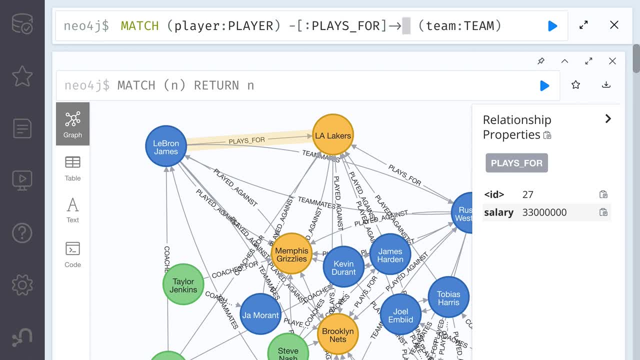 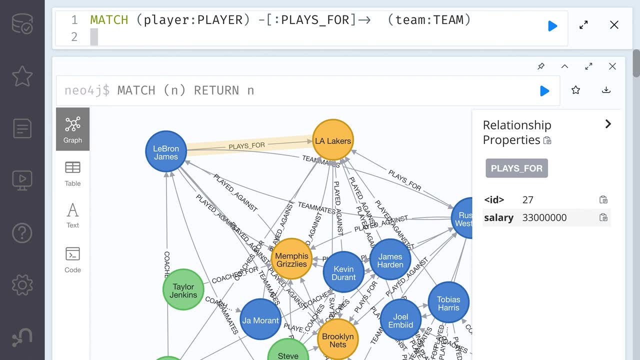 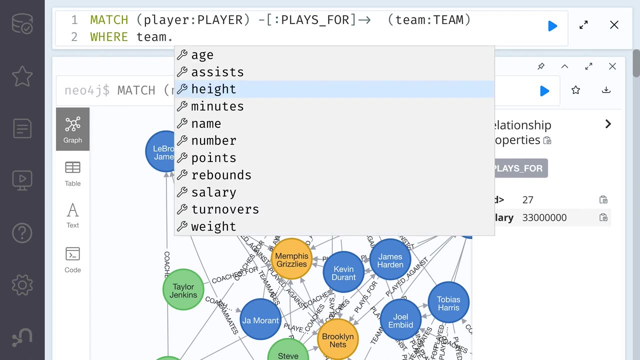 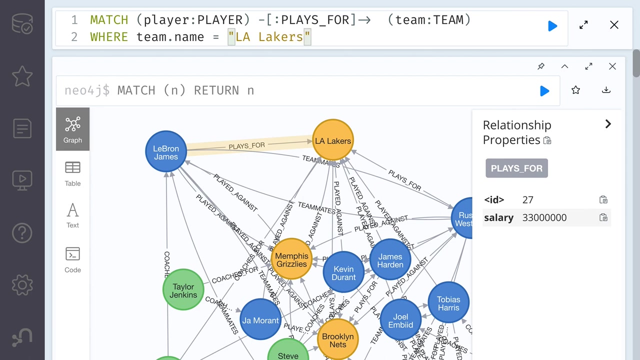 specify the direction. all right, cool, so let's go ahead. and we have this thus far. now what we want to do is we want to return all of the players that play for a specific team. so now what we can do is simply say where teamname equal to Los Angeles Lakers, and this is also going to filter the team as well as the players. so the 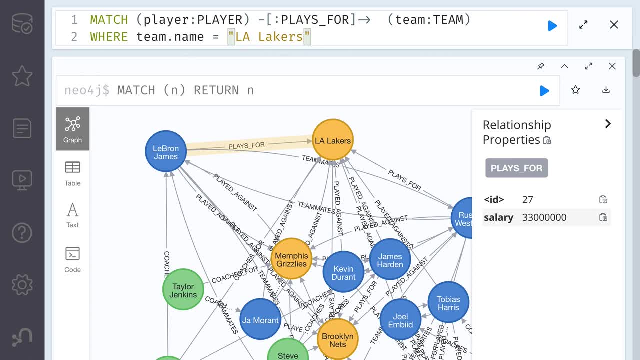 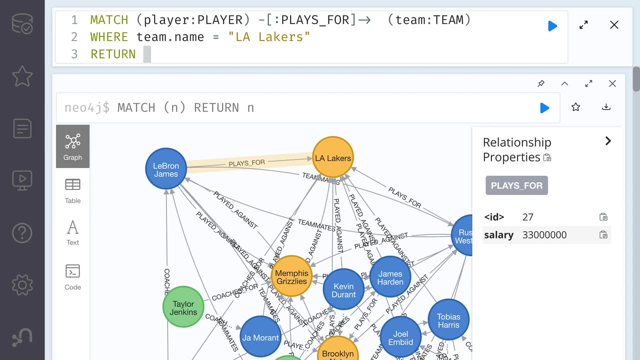 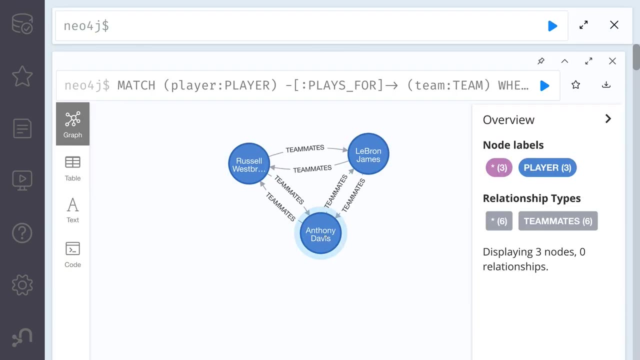 players also have to play for the Los Angeles Lakers, and then what we're going to do is we're going to return, we're going to return the player, so it's going to return the player, and if you were to execute this, you can see. now we get all of the players that play for the Los Angeles Lakers, okay. 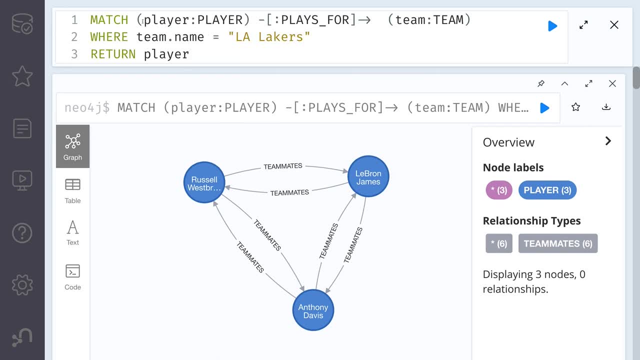 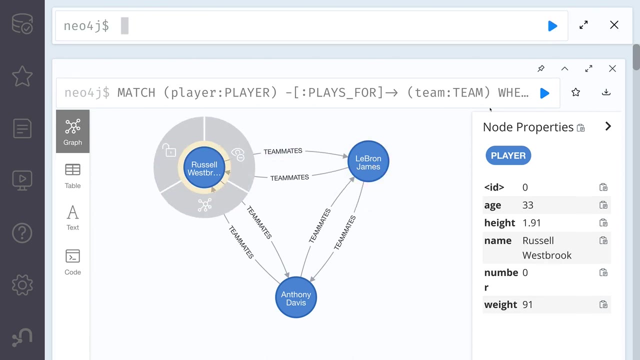 I hope that makes sense again. we have a node here for the player, we have the relationship, we have the team over here, we have our wear clause and over here we're returning the players that play for the Los Angeles Lakers, which are all of these, and of course, if we wanted to, we can also return the team itself, so we can go. 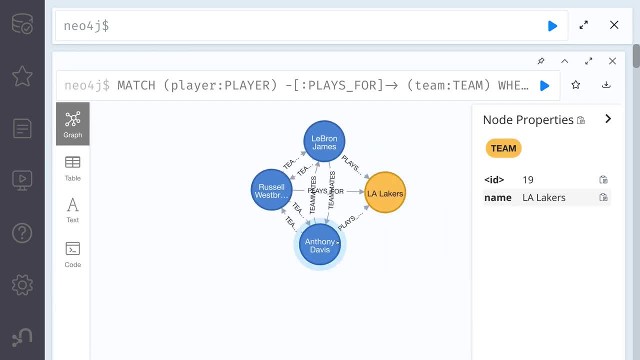 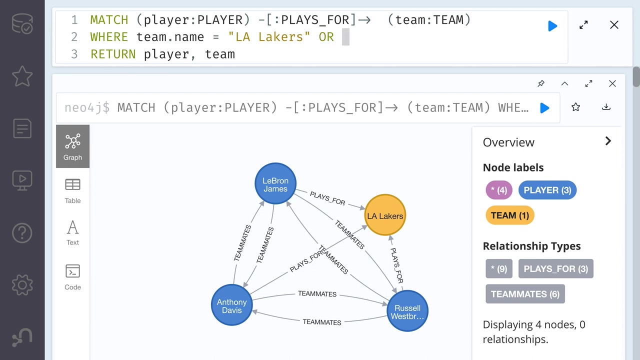 here and now we have this relationship and it looks kind of wacky, but again we have Russell that plays for all of these teams. so Russell, LeBron, AD, okay, cool. and of course we can have more complex queries if we want to. here, you know we want. or the team dot name is: maybe the Mavericks, maybe you want to get the. 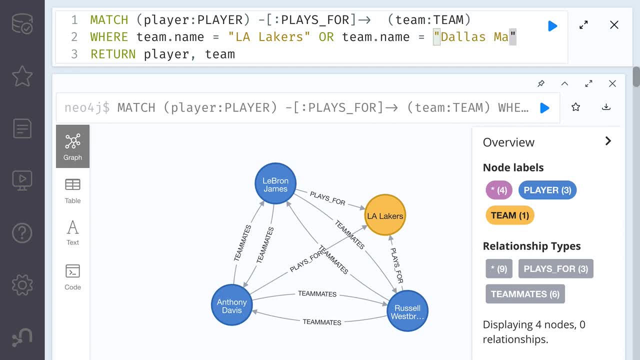 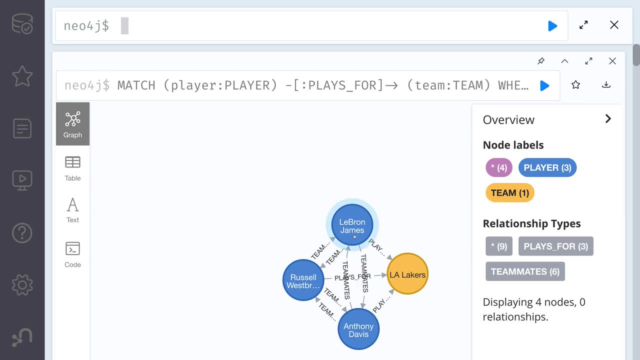 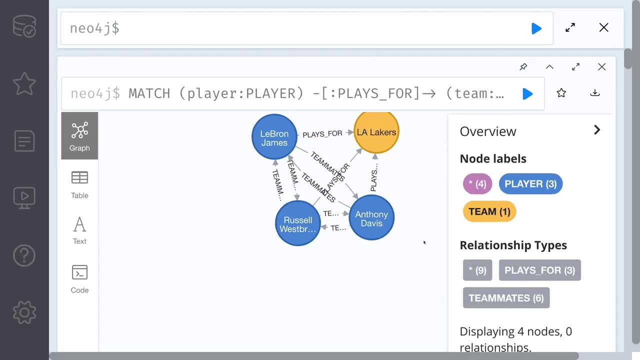 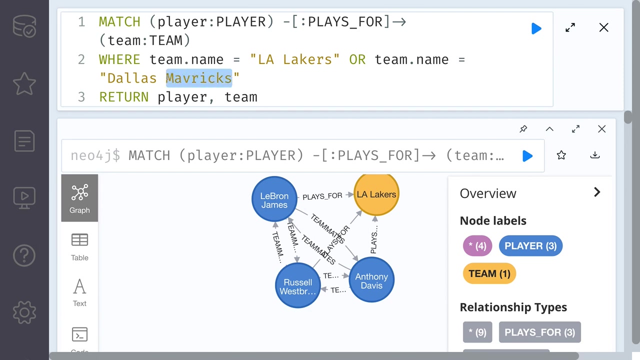 Lakers and the Mavericks. So we can say Dallas, Mavericks, Mavericks, And if I were to execute this, then we get: where are the Mavericks? Let's zoom out here. Okay, maybe we made a typo because we should have the Dallas Mavericks in here as well. Dallas, yeah, I misspelled this, So Dallas. 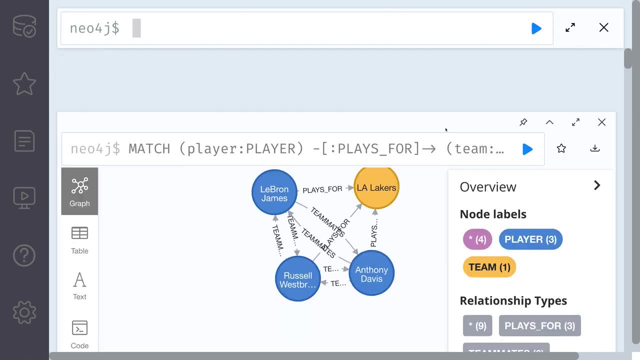 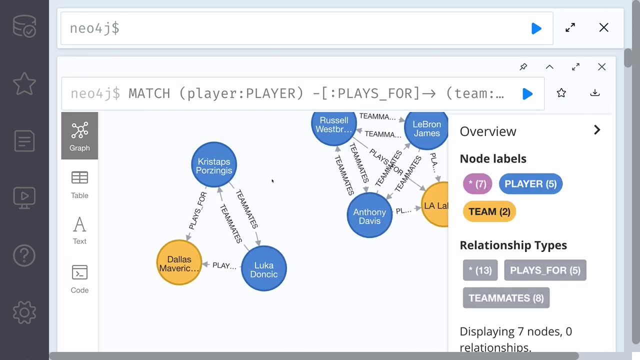 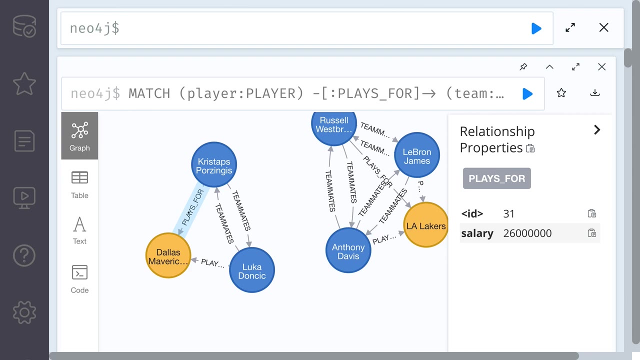 Mavericks, If I were to spell that correctly. you can see, now we have these relationships. Cool, All right, that is awesome. So now what I actually want to look at is if you go to the play for, if you click on any play for a relationship, you can actually see that this relationship 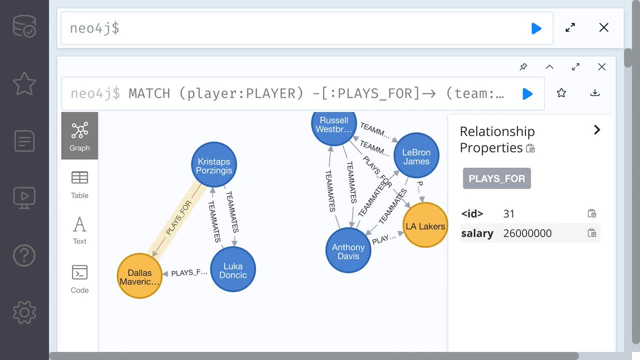 itself has a property called salary. So, remember, nodes can have properties, relationships can also have properties And you know these properties can have whatever it is that they want in them. Now, over here for the place for we have the salary property. So let's actually write a query where we 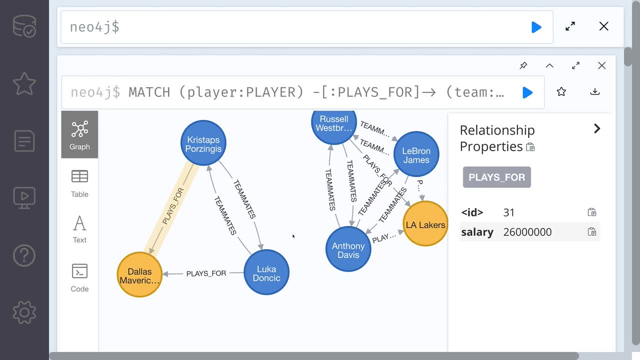 query for all of the players that have a salary that is greater than 35%- $35 million. So we want to see who's like the richest players. Now, all these players are making incredible money, But let's just get the ones that are making more than $35 million a year. 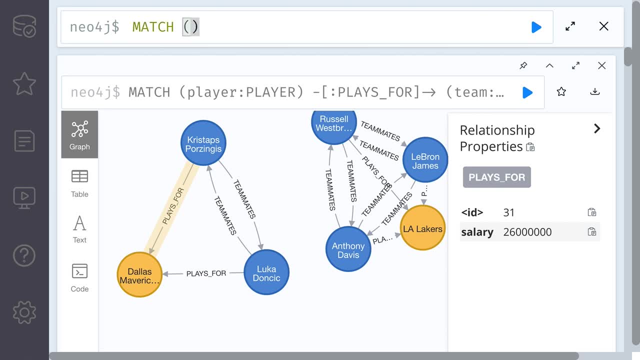 So let's go ahead and let's do this. So we're going to do this from scratch. So we're going to say: well, we want the player node And we want to get the, we want to get the play for relationship, because that's where the property, salary property- exists. So let's specify this with the label. 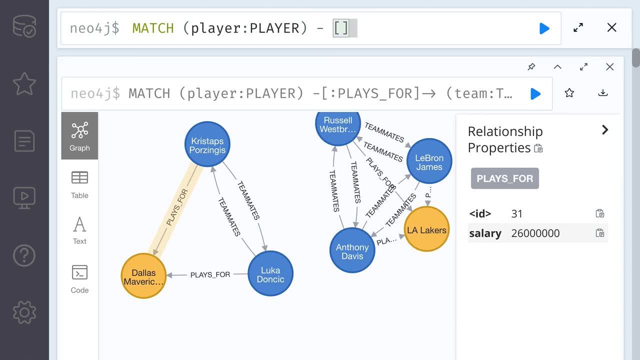 we're going to say we want to get the team, So we're going to say over here team and we're going to say colon team And over here. what we want is we want the place for relationship And we can actually give this. 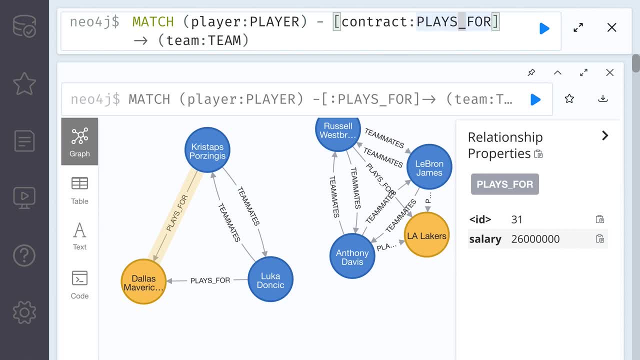 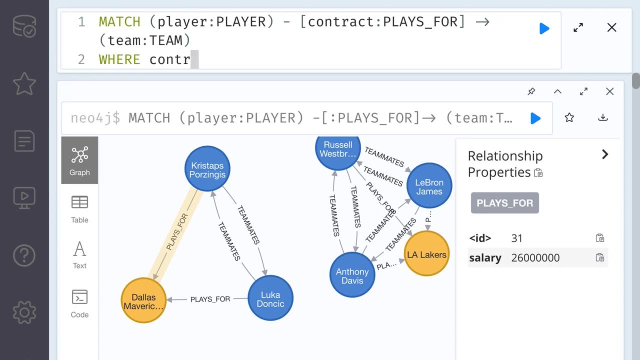 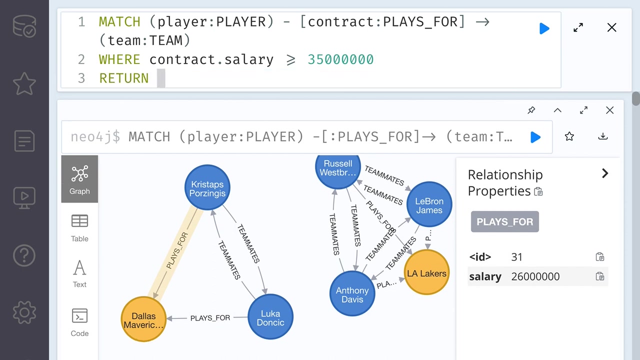 a variable name. I'm going to call it contract. So I'm going to call this contract. So now what we can do is we can simply say: where contract dot salary is greater than or equal to $35 million, Let's make sure that we get a type in the 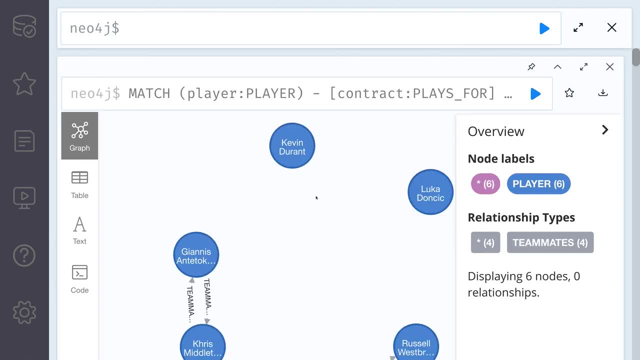 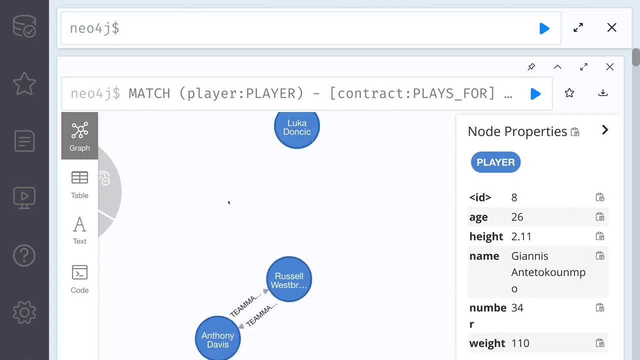 �미는 $35인, or equal to 35 million. So let's make sure that I have the right zeros, And then what we can do is simply just return the player, And because we're not using team here, we can just simply omit this over here. So let's go ahead and execute this, And now you can see, we get Kevin. 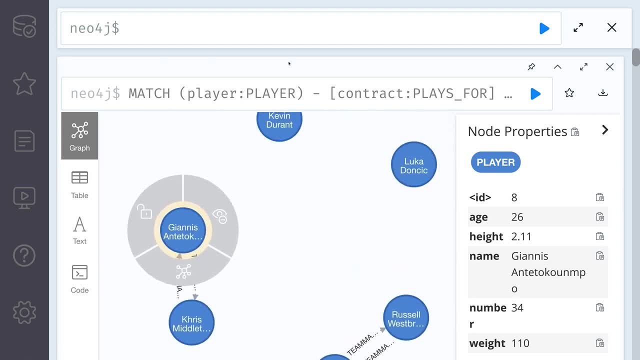 Durant, we get Luca, we get Russell, we get AD, Chris Milton and Giannis. Surprise, LeBron's not here. Oh well, I guess LeBron's not making $35 million. so that is the query, and if we wanted to know exactly how much they're making, then we need 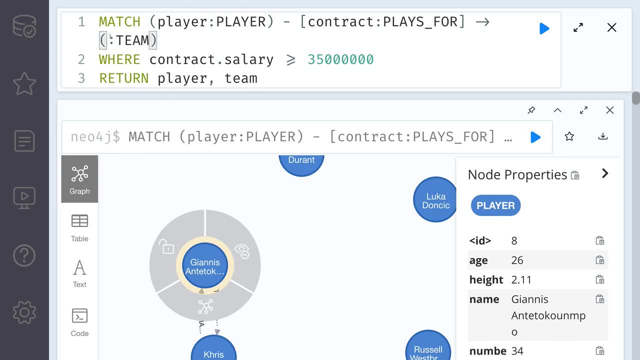 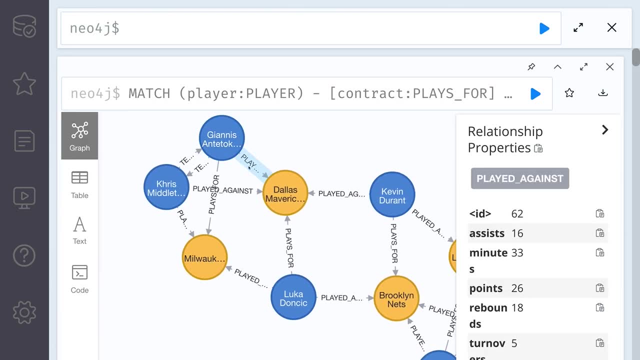 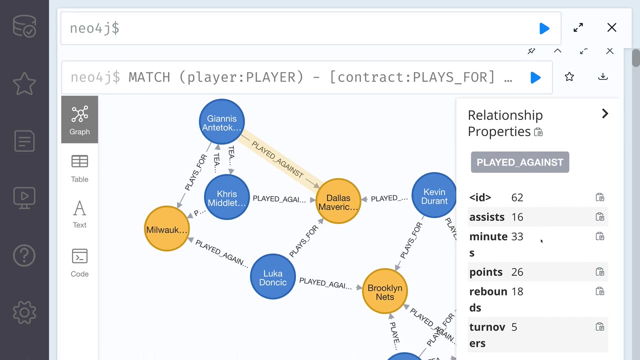 the relationship. so this time we might need the, the team, so we can see the relationship between the team as well as the player. so now we have yannis, who plays, so this is plays against, so played against, so this is not plays for. this has another set of properties which is like the actual. 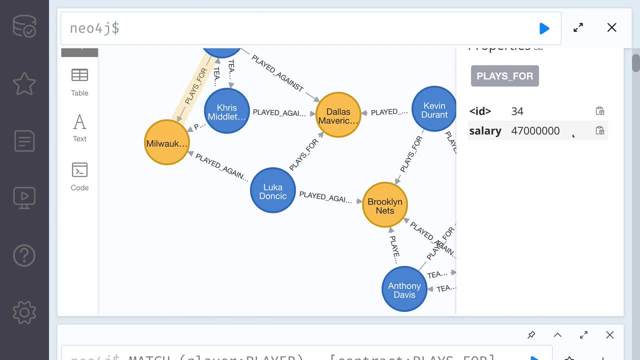 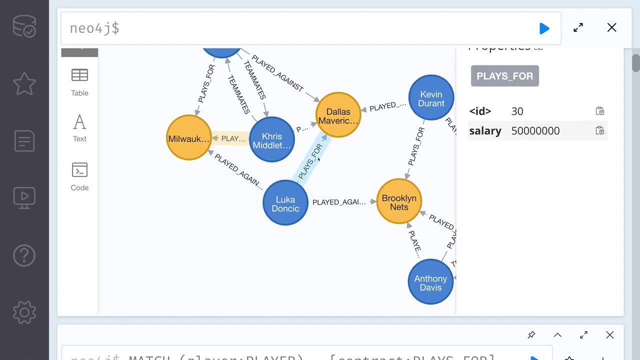 points that they got the minutes or whatever, but if you go to plays four, okay, yannis is making 47 million. if i go over here, chris milton's making 43, luca's making 50 million. i wish i could make 50 million. oh, my goodness, we got kevin durant. he makes 45 million and we have anthony davis is probably the poorest one out of them. we might need to make a gofundme page for anthony davis davis- only 38 million, wow, while everyone else is making 45 million plus. okay, so you guys get the point. so that is. that is well pretty much it. so let's actually make one last, relatively 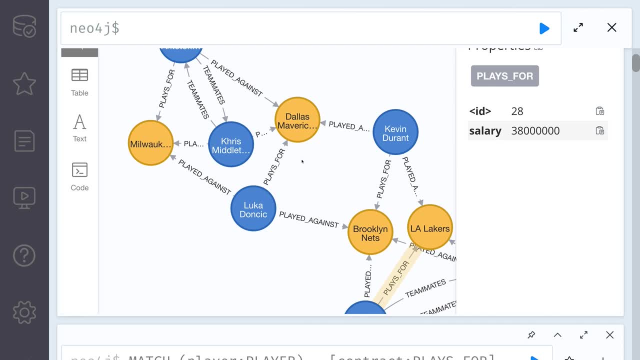 complex query. let's now do something, and i highly encourage you to try to do this on your own. this is a little bit tougher. i want you to get all of lebron's teammates. so all of lebron's teammates that make more than 40 million dollars. so let's actually try that query out. 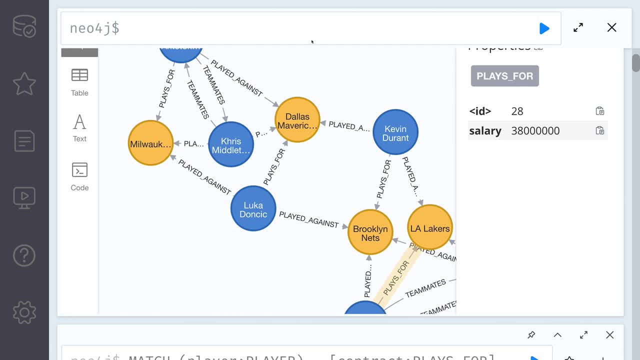 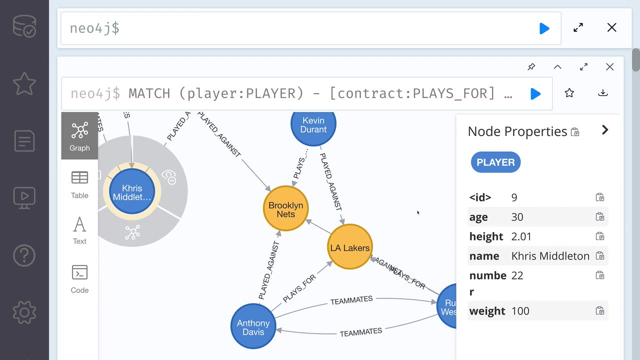 so i'm going to give you guys five seconds to try it on your own- five, four, three, two, one. hopefully you guys paused the video and gave that a go. now, remember, the problem is we want to get to all the lebron's teammates that make more than 40 million dollars, so this is a relatively complex problem. 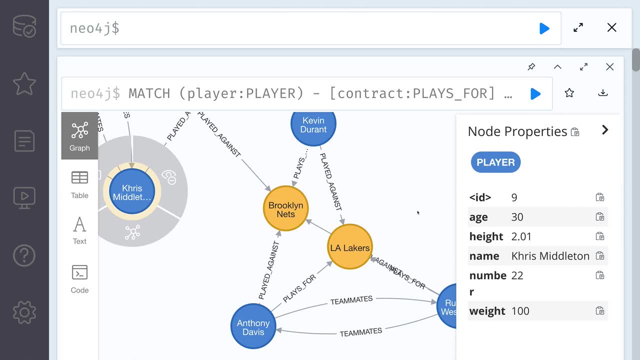 but we can actually simplify this problem into many well smaller problems like this one. so let's first, for example, the first thing that we probably want to do is figure out a way to query for lebron's teammates and then, once we get lebron's teammates, we can query for the players that make over 40. 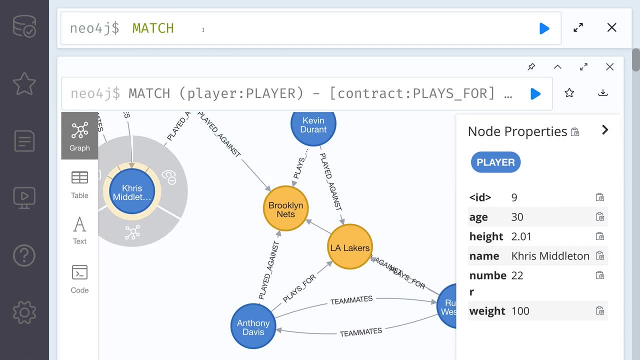 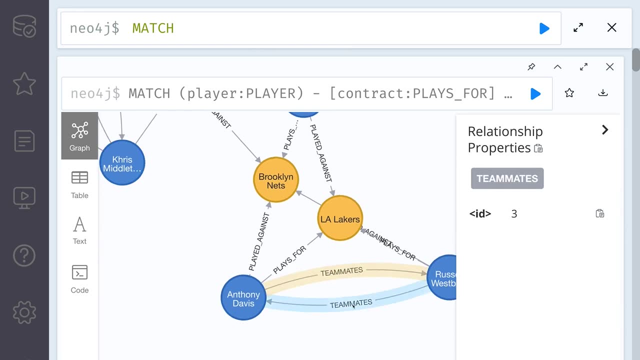 million dollars. so let's begin by just getting all of lebron's teammates so to do this. what we're going to represent his teammates, we're going to have a relationship between them, which is the teammates relationship right over here. So the first one is going to be LeBron and this is going to be a. 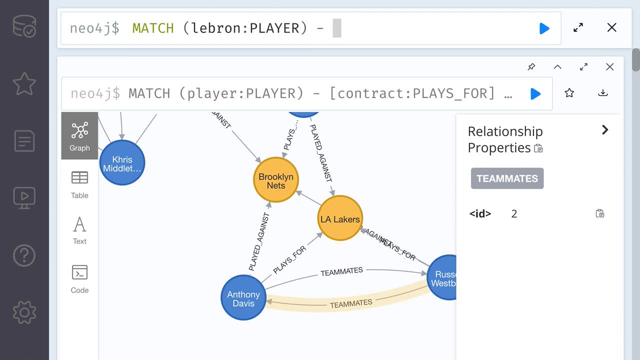 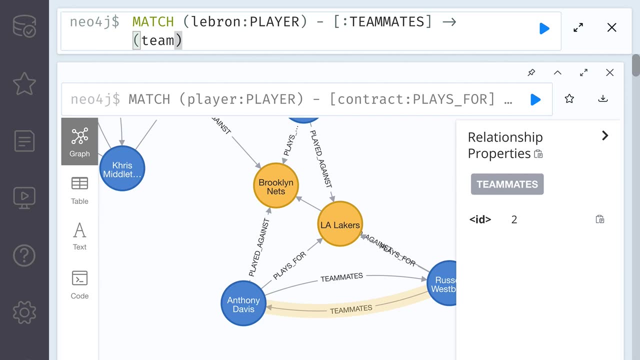 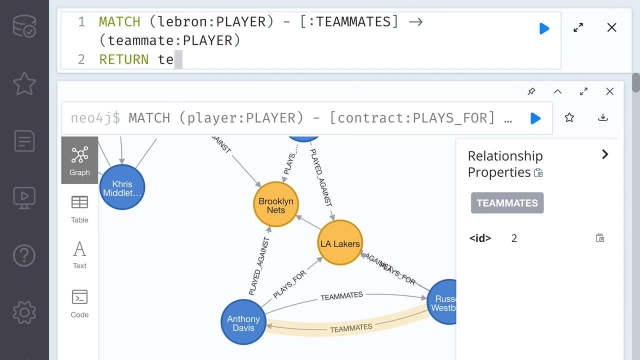 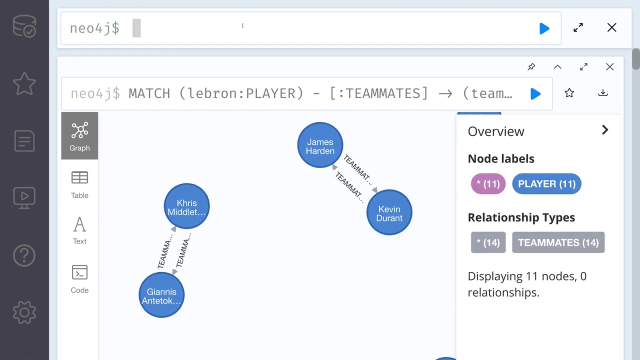 player- And we're going to have LeBron- the LeBron node- have a teammates relationship with the well, with another player that we're going to call them a teammate, And now what we can simply do is just return the teammate, And if we were to execute this, we would get nothing. So this is not what. 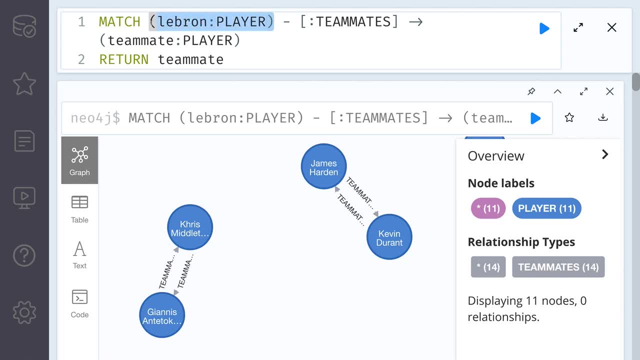 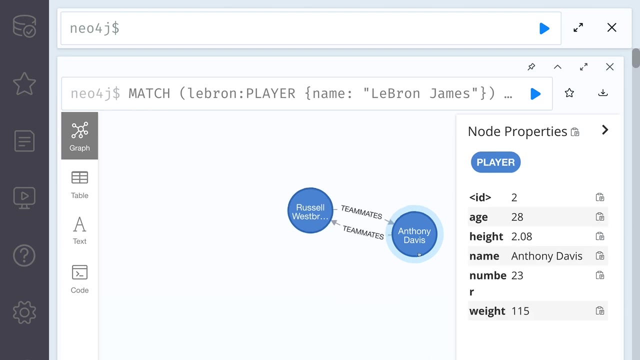 we're getting, And the reason for this is: right now LeBron is anybody. we have to actually filter for the actual LeBron. So what we can do here is you can say: simply name LeBron James And now we can. we only get Russell Westbrook and Anthony Davis, which are LeBron's teammates. So now what? 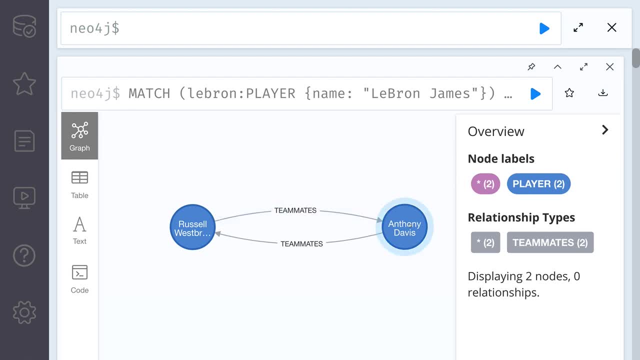 we want to do is we're going to have a relationship between them, And we're going to have a relationship between them, And we're going to have a relationship between them, And what we want to do is we want to get the salaries of these two players. So let's go back here, click the up key And remember the. 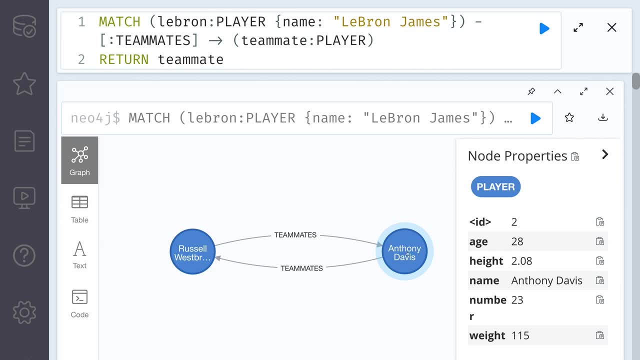 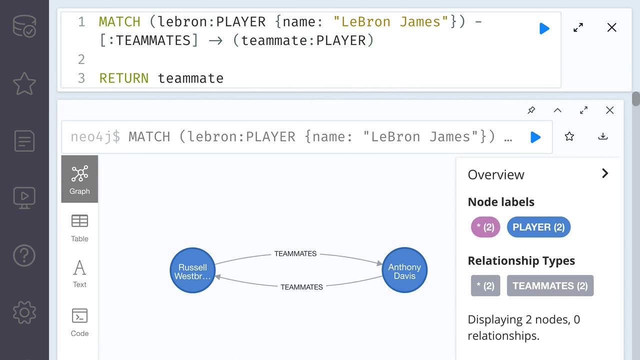 salaries lives in the relationship between the player node as well as the team node. that plays for relationship. So what we need to do is we need to get the, we need to get the players, So we need to- sorry, we need to get the team. So we can actually do this by having another match. So this 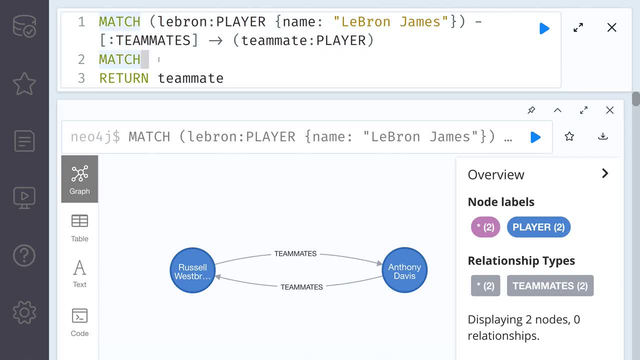 is the first time we've actually done this. we can actually have another match. So we can actually have as much matches as we want to query for specific things, and over here we can say that we want the teammate node to have a relationship or we want to query for the teammate node that has a place. 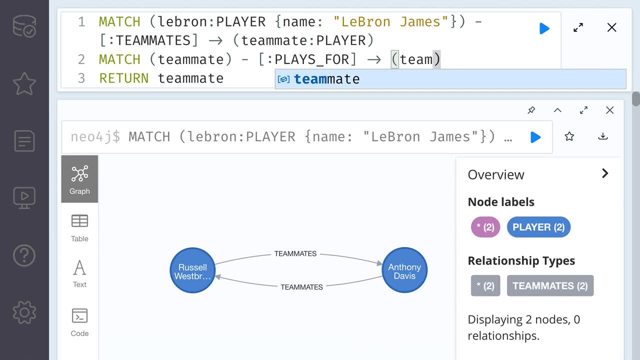 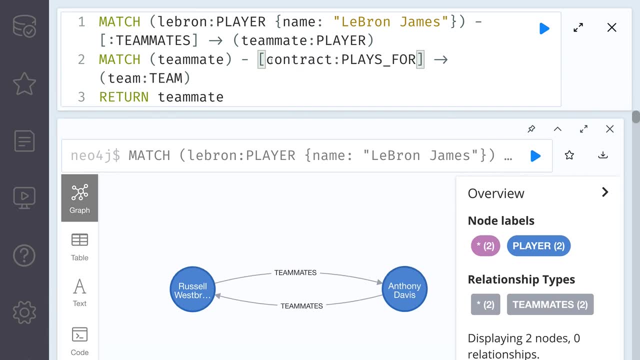 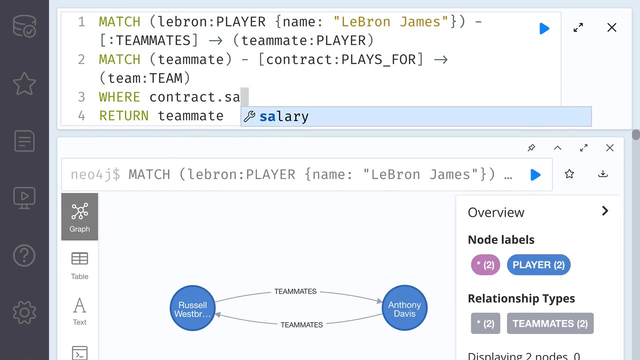 for relationship with the team node. so with the team node, and we can actually call this over here: the contract. and now what we can simply do is just filter where the contractsalary is a greater than or equal to 40 million. so let's, let's make sure I have enough zeros in there. one. 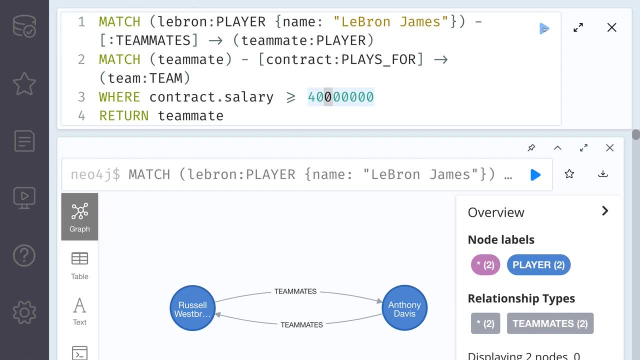 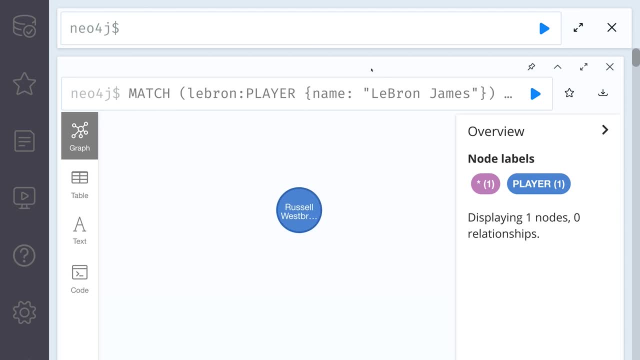 two, three, one, two, three, forty million. so let's execute this. and if we were to execute this, we only get Russell Westbrook, who's making more than 40 million. so I hope that query makes sense. over Over here, we're getting all of LeBron's teammates. 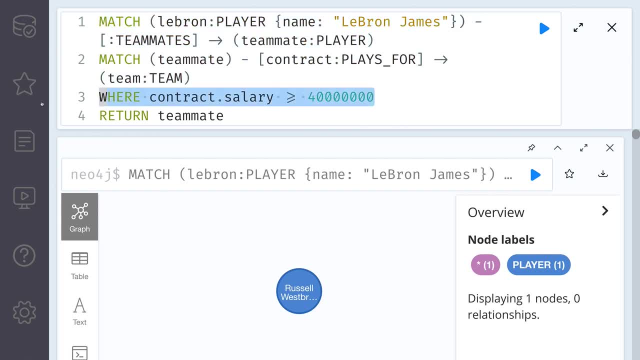 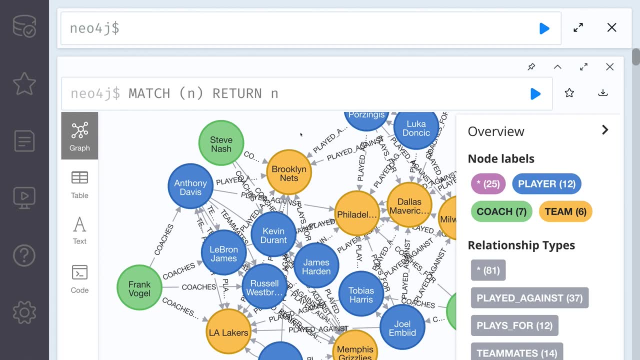 Here we're just getting access to that contracts relationship. Here we're doing the filter and then we're returning those teammates. The last thing that we need to learn when it comes to querying data is aggregation. So aggregation is the process where we have multiple data sets and we aggregate them into. 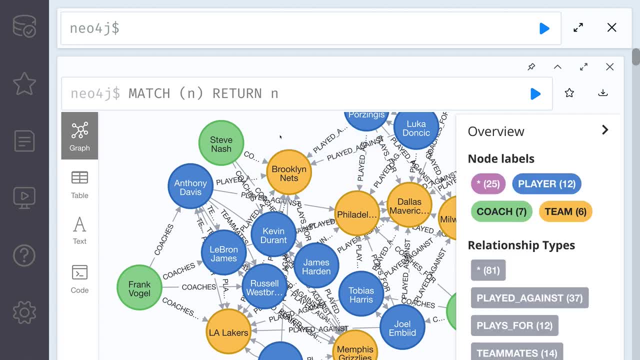 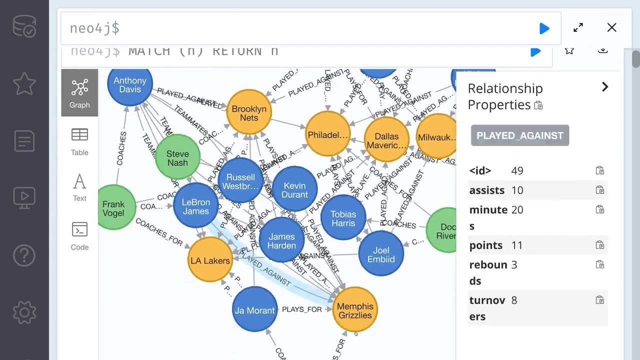 one value, And the best way to actually learn it is to just go through an example. So we're going to go through an example where what we want to do is return the player's names as well as the number of games they played. So, in order to determine the number of games a specific player has played, there is this: 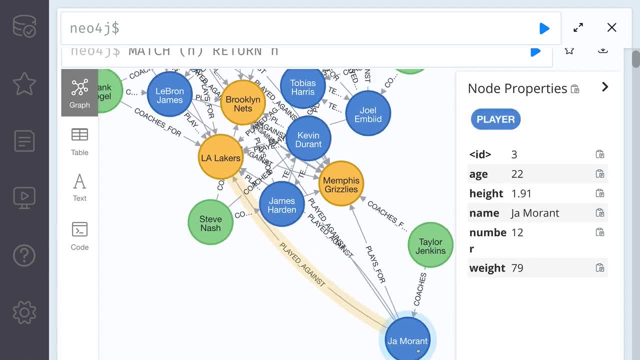 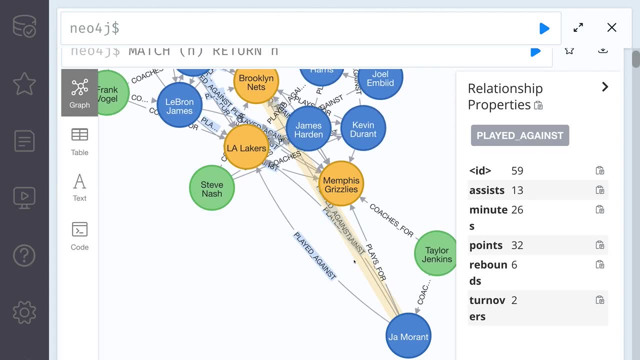 played against relationship. So what we want to do is we want to go get a specific player and then we want to get all of these played against because, as you can see, we have multiple. It might be difficult to see, but we have played against here, played against here, played. 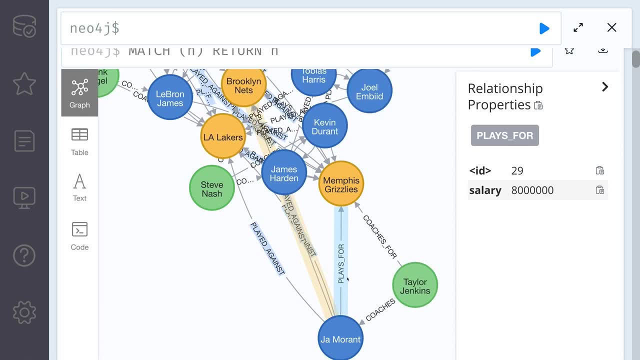 against here And we just simply want to sum them Or just count How many we have, And that right there is aggregation. We're getting all of these played against relationship for that specific player and we are aggregating it into one value, which in this case, is the sum or the count. 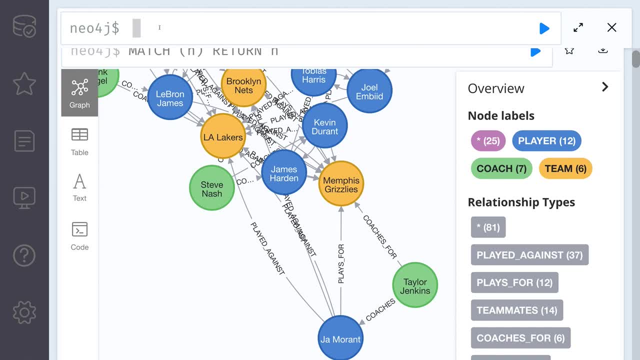 So let's actually do that right now. So the first thing that we want to do is: well, we want to specify that we want to get the player. So, of course, we want to get the player because we want to get the player node, And the played against relationship is going to be with. 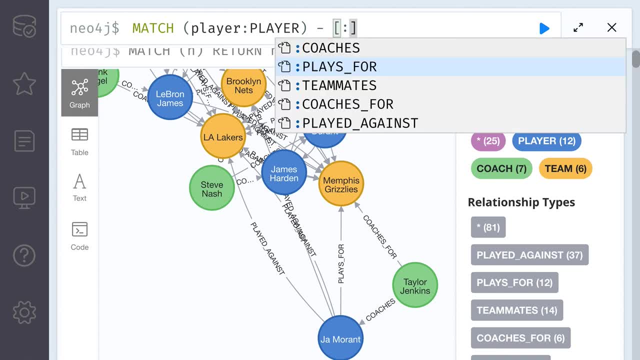 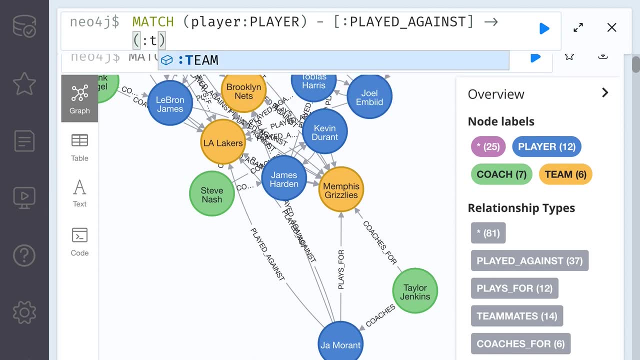 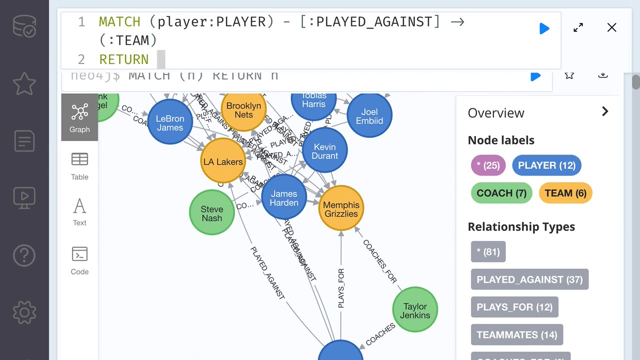 The team node. So over here we can specify that we want the played against relationship, And then this is going to be on the team node itself. So the team node, And so now all we simply have to do is return the playername because we want the name. 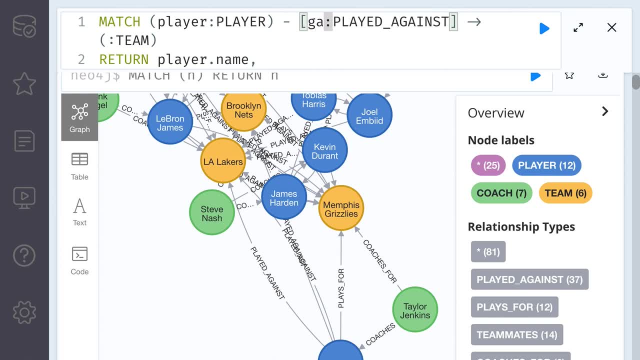 And then what we can do is we can give this relationship a variable name, called games played, So games played, Or game played, And then over here all we need to do is just very simply say: count game played, So how many game played does this specific player have? 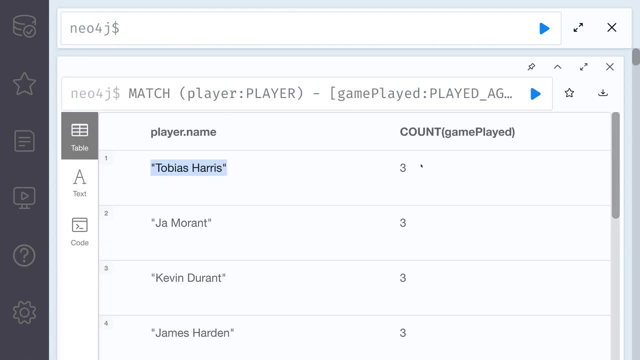 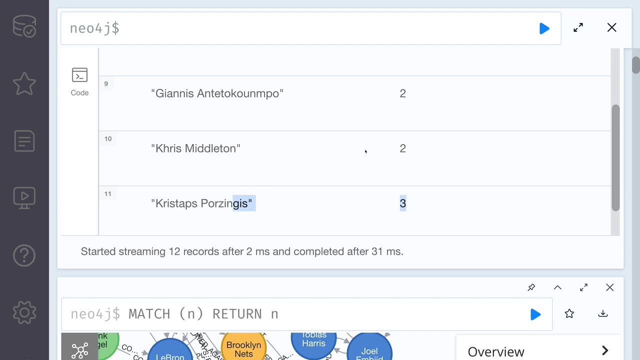 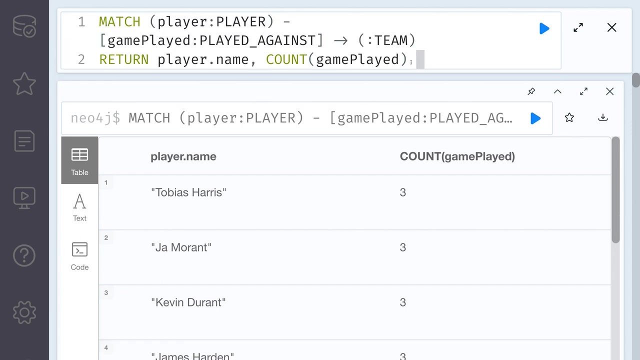 And if we were to execute this, you can see, here we have the name as well as the number of games that that player has played. So you can see. you know, Porzingis has three, Milton has two, Yiannis has two, etc. So that right there. so this, right here, is an aggregation, because we're aggregating the. 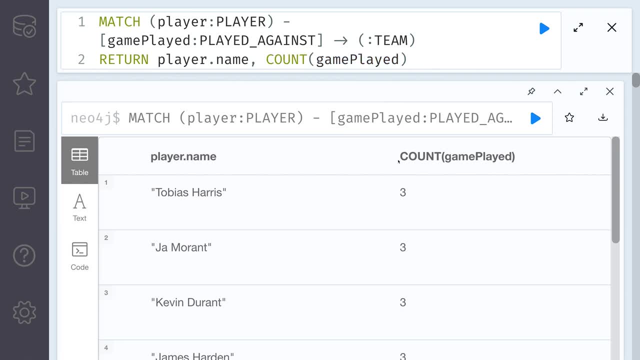 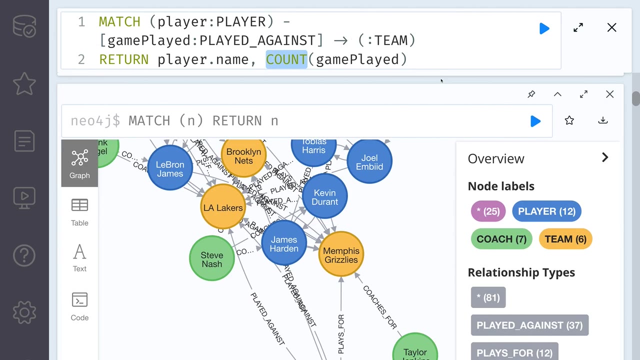 number of games played Into one specific, specific value, which is the count. All right, Awesome. So now, because we know aggregation, we can actually do some really cool things. So this played against. so let's go back over here. This played against property actually has different or played against relationship has. 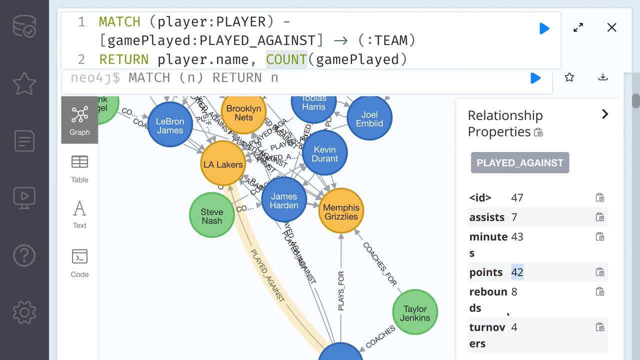 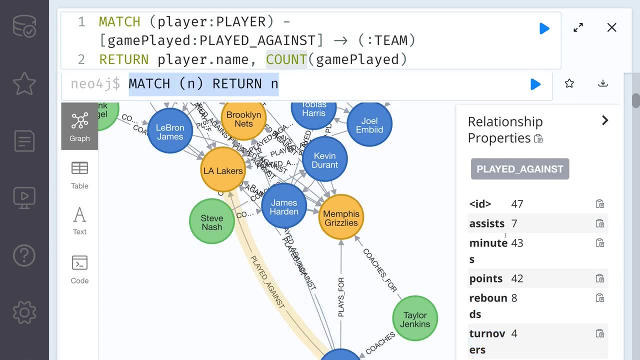 different properties within it. It has the minutes, it has the assists, it has the points, it has the rebounds, it has the turnovers. So So now what we can do is we can aggregate these properties as well, So we don't have to aggregate the relationship itself. we can aggregate the properties into. 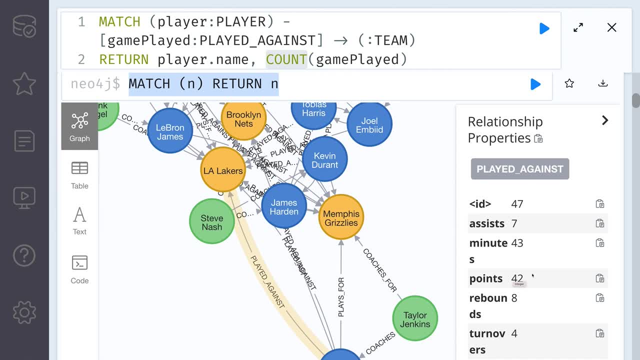 a specific value. So maybe what we wanted to do is: well, we want to get, we want to get all all the players names as well as how much they average per game. So how much points the average per game? So we can actually do that very easily by switching out this from average. 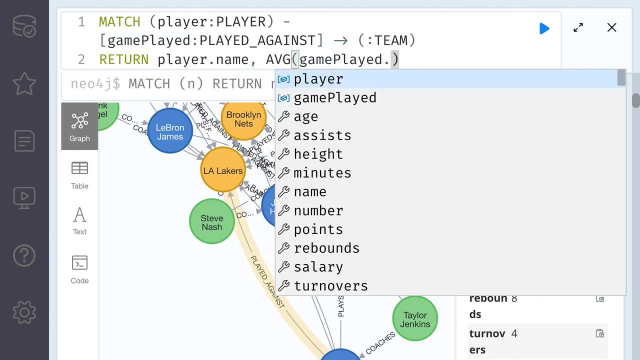 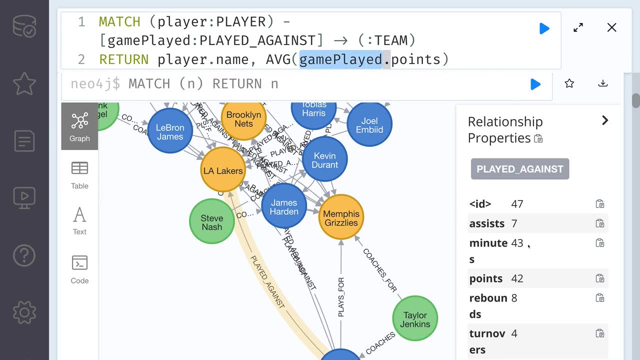 And what we want to do is we want to get the average of their points. remember, the games played is a property that has the games played is a relationship that has the points property. So if you were to query for this and if we were to scroll all the way up, you can see. 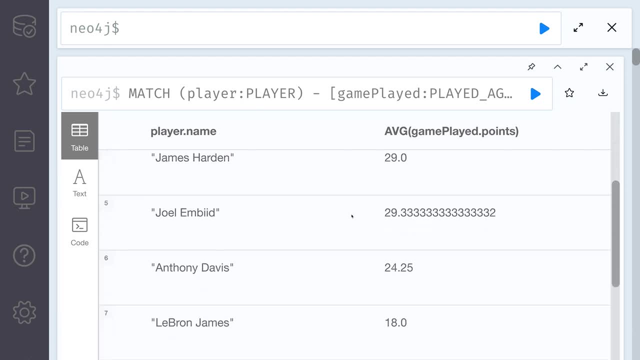 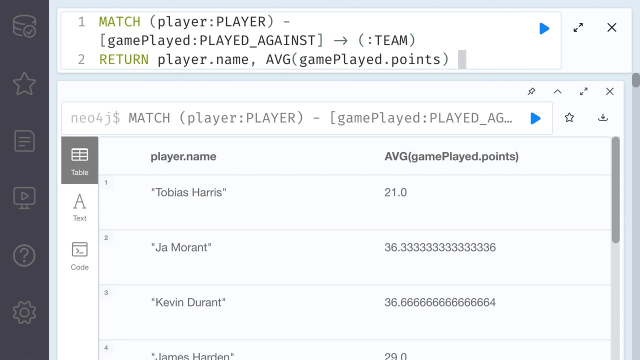 here. we get their average points per game. All right, Awesome. So now, of course, we can do some really cool things. if we wanted to get maybe the highest highest- A person that scores the most points, highest points per game we could do is we can actually. 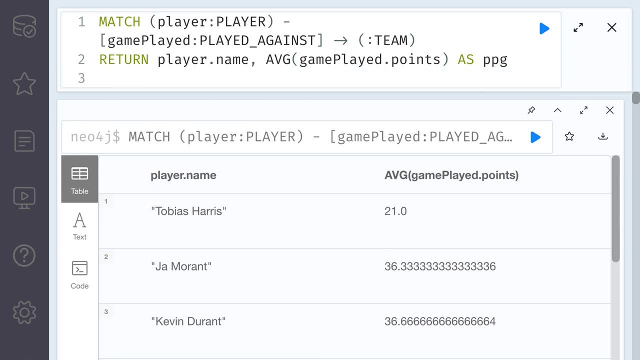 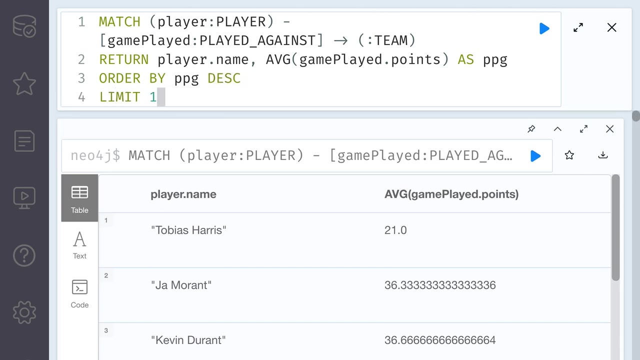 alias this we can say as points per game, and then down here what we can do is we can actually order by- and we can make this whole capital case order by points per game, and we can make a descending order and then, very simply, we can just limit it to the first person. 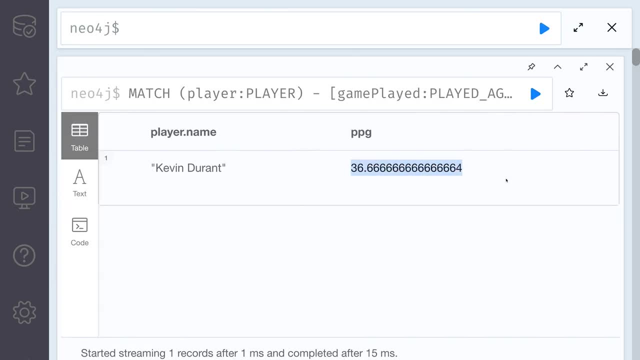 And if you were to execute this, we should get Kevin Durant, who is averaging thirty seven points Again. now there's a bunch of different methods that we can utilize, such as some: which sums up well, you guys probably get the point. it sums up a bunch of values. 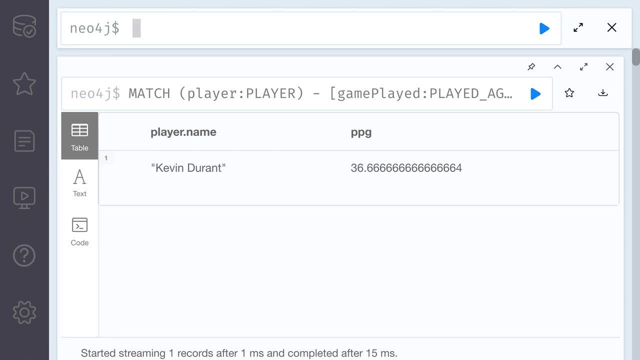 You also have Max and men. that we won't get into because I don't want to make this course too, too long, but you probably get the point. Max is going to get the maximum value, man is going to get the minimum value. OK, my good friends, in this part of the course, what we're going to do is we're going to learn. 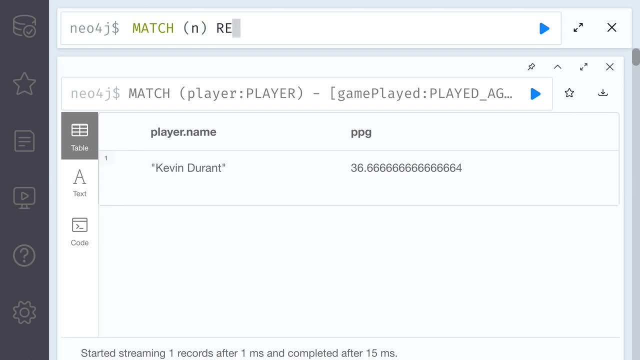 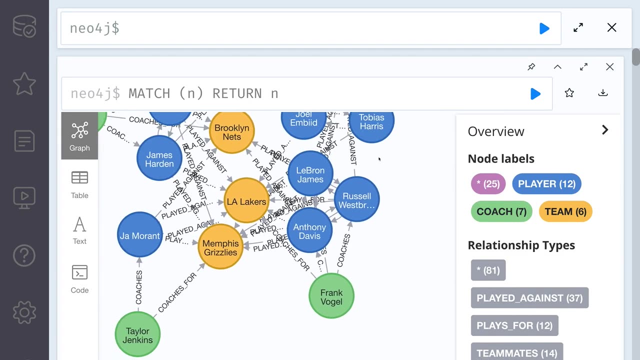 how we can delete nodes. So the first thing I want to do is let's just return every single node that we have And let's say what we want to do is delete John Moran. Let's say for some reason he's out of the league or we don't want him inside of our 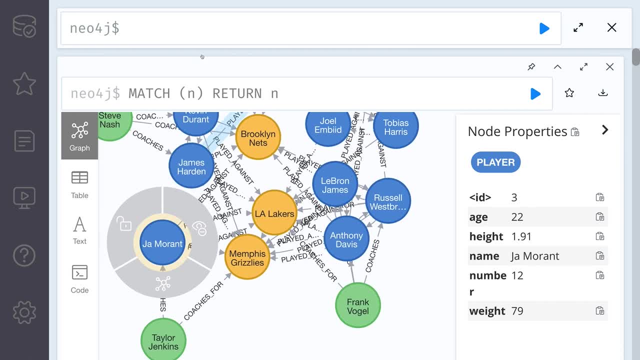 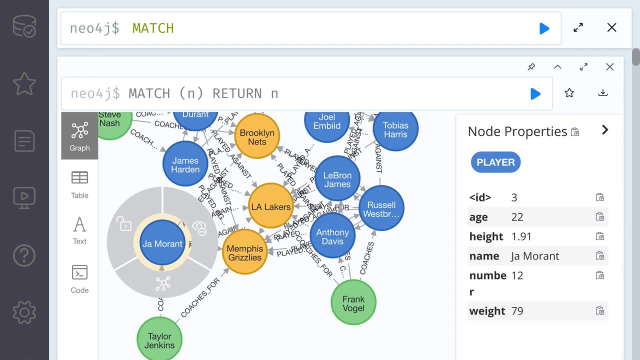 database. So, in order to delete John Moran, the first thing that we need to do is find John Moran to note that John Moran to note. So over here we can specify match node. We can also say that the name is going to be John Moran. 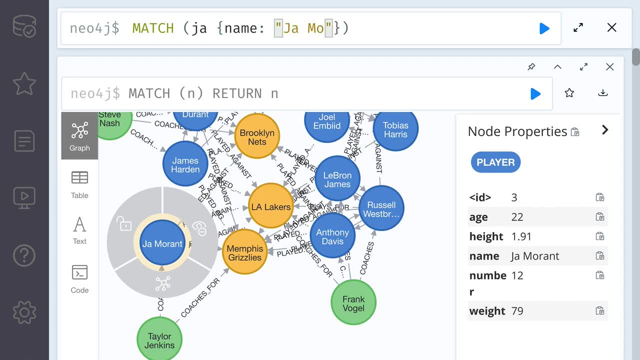 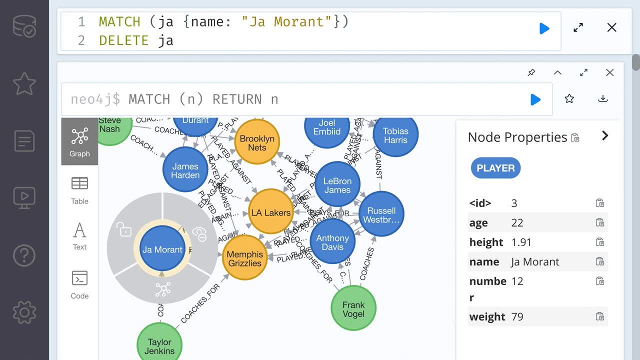 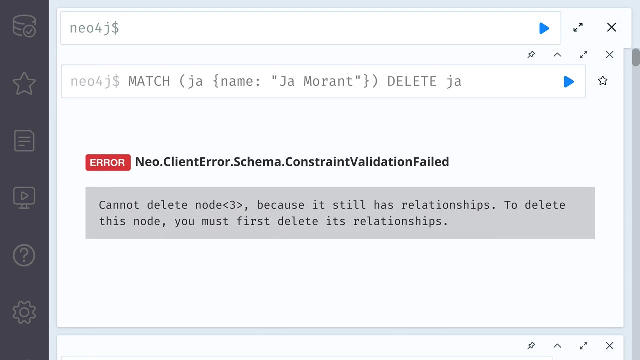 So we can say: jaw more rent. So you can say: John Moran. And then what we can simply do here is say: delete jaw. Now, if you were to execute this, we are going to get an error, And the reason why we're getting an error is because jaw has relationships. 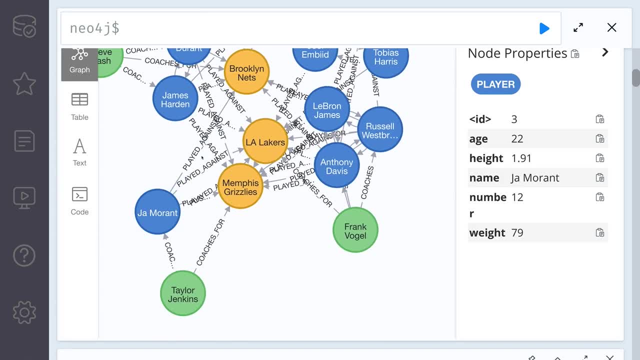 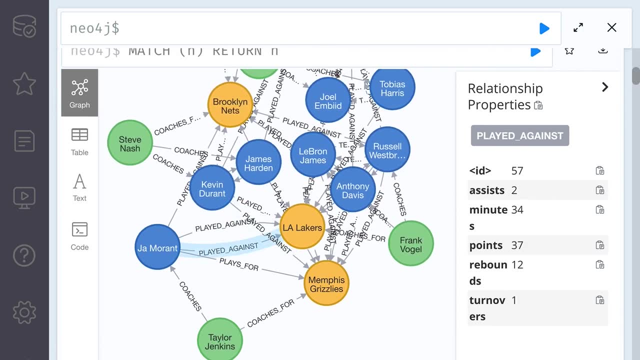 And so if I were to go here, you can see jaw still has the played against relationship as well as the played for relationship. OK, So what we need to do is we need to delete the. we need to delete the node as well as those relationships. 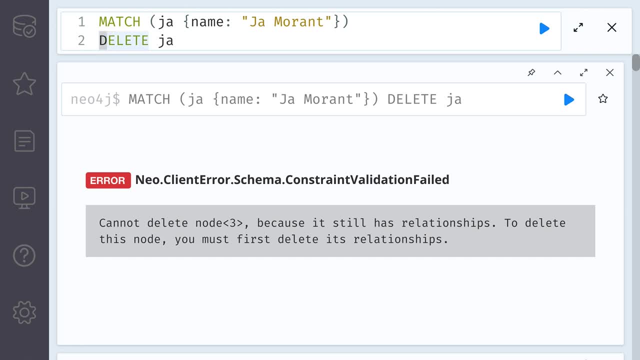 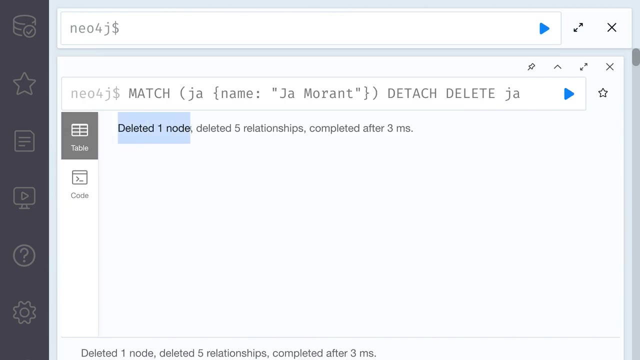 And a very quick way to do this is by prepending the detach keyword, And what this is going to do is going to detach all of the relationships, thus deleting them, And then it's also going to delete that jaw node. So now, if we were to execute this, it has been deleted. 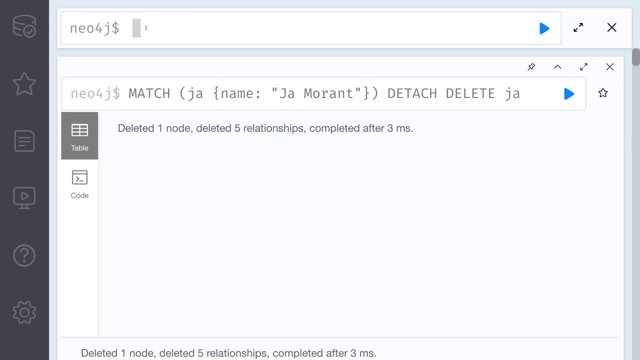 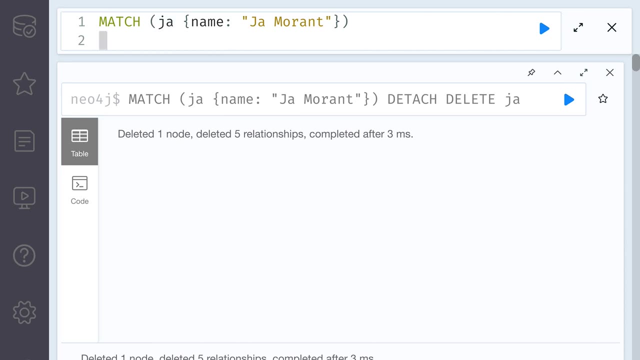 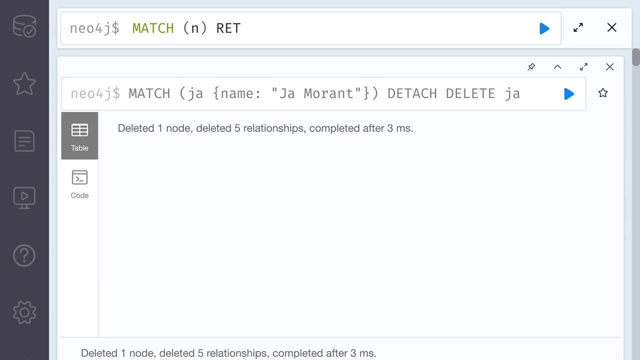 So we have one node deleted as well as five relationships. So if we were to try to do a match, you know, get all the nodes, let's do that again here. Let's do match and match and return and return. and if you were to execute this, you can see. 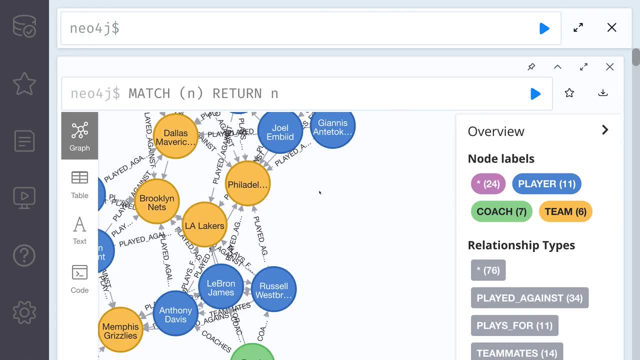 here. jaw doesn't exist anywhere. OK, So now let's actually talk about another thing that I want to delete. Let's say we don't want to delete the actual node itself. Let's say we don't want to delete the actual node itself. 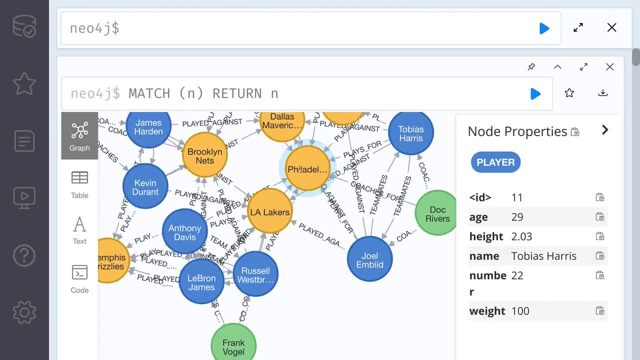 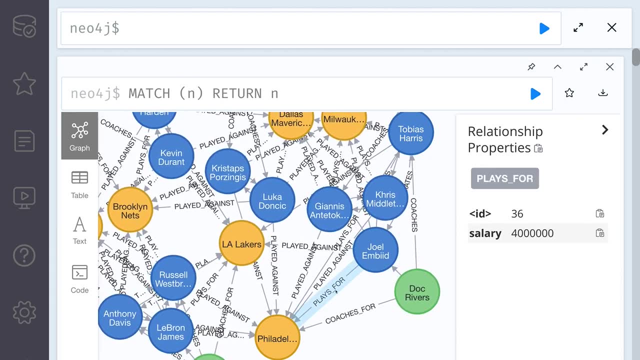 Let's say we don't want to delete the actual node itself, But we want to delete the relationship. So, for example, let's say Joel Embiid got traded, or he decided to retire or whatever, and thus he doesn't play for the Philadelphia 76ers. 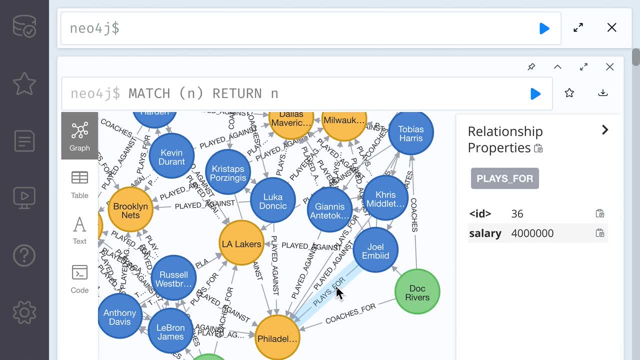 And so we want to actually keep Joel Embiid, but we do want to just delete this relationship. In order to do this, this is going to be very simple: We have to find that relationship. So we're going to say: over here, Joel, and then we're going to say that the name, name is. 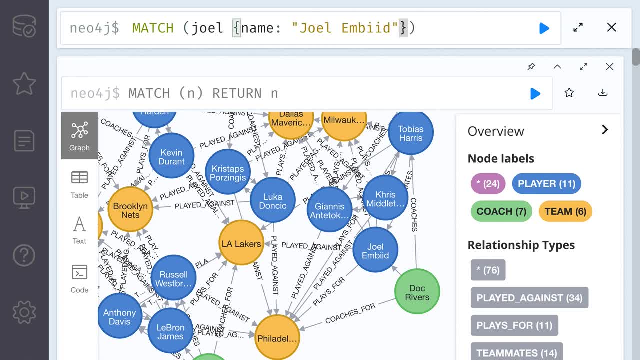 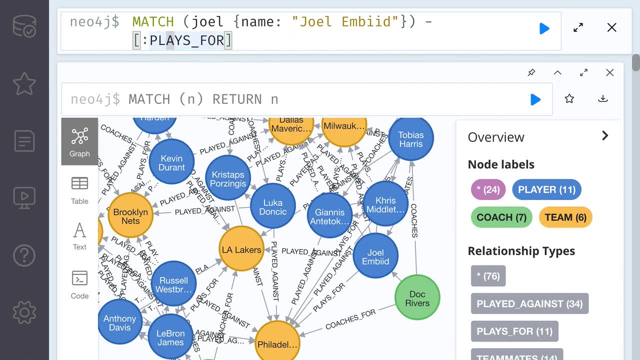 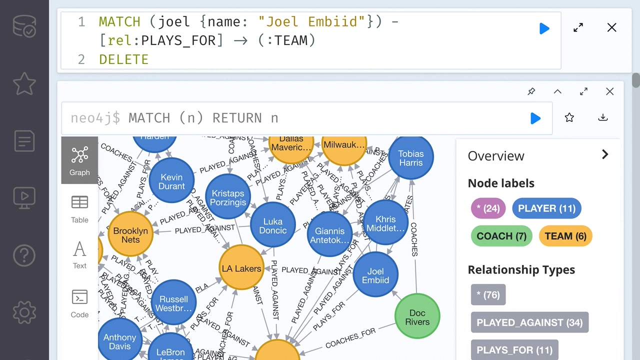 Joel Embiid. and then, over here, we're going to say that we want the place for relationship and we can give this a relationship of rel. and then, over here, we're going to say that this is going to be with the team, And now what we can simply do is delete. we don't have to add the detach, because here, 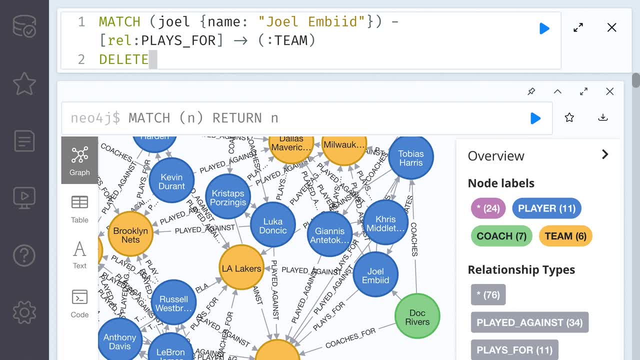 we're just deleting a relationship and we can just simply delete the relationship and remember this relationship is only going to be the place for relationship, which is going to be one. If we have a multiple relationships, we can actually just filter for whatever relationship that we want. 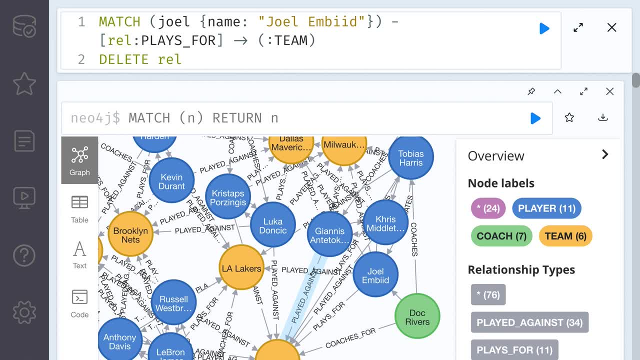 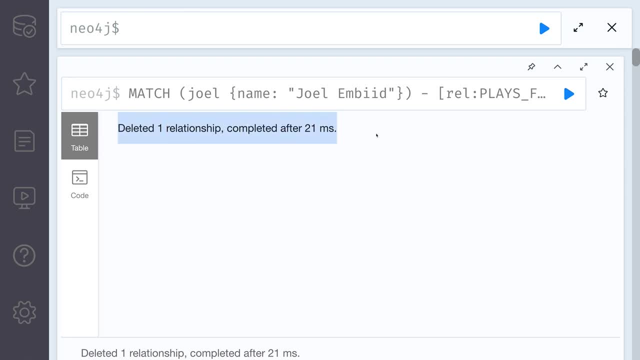 For example, maybe we wanted to delete a plate against. we can filter for maybe with the ID that we want and then that would get deleted. So if you were to execute this, you can see here that no node was deleted. but now we have a relationship deleted. 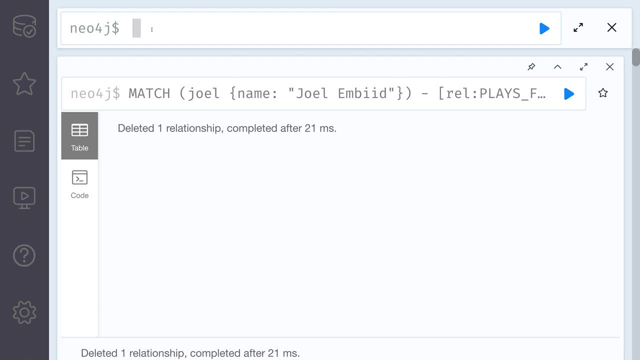 Okay, cool. So that is really all we have to know with deleting nodes, So it's not very difficult at all. And now what I want to do is I want to delete every single node in our application, and I highly encourage you to try to do this yourself. 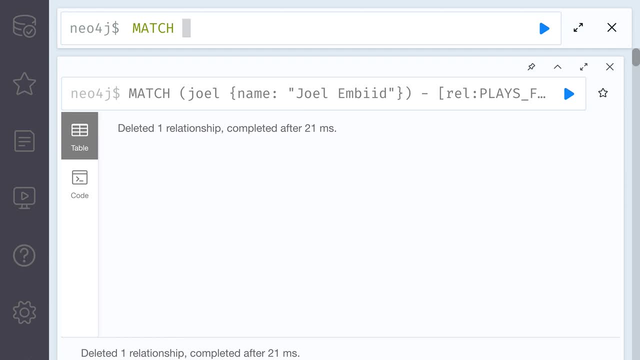 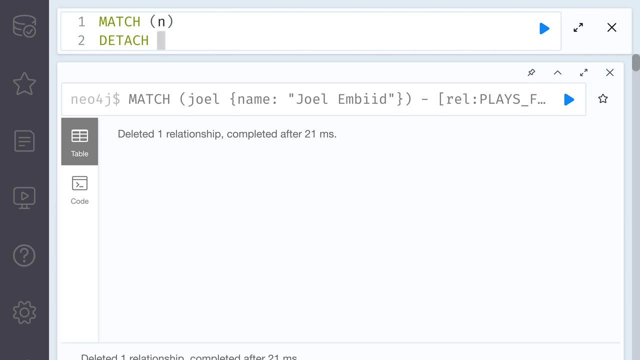 So 5, 4, 3, 2, 1- hopefully you pause the video- So to do this, what we're going to do is we're going to get every single node and then we're going to detach everything, So we're going to detach all the relationships and then we're just going to do delete and 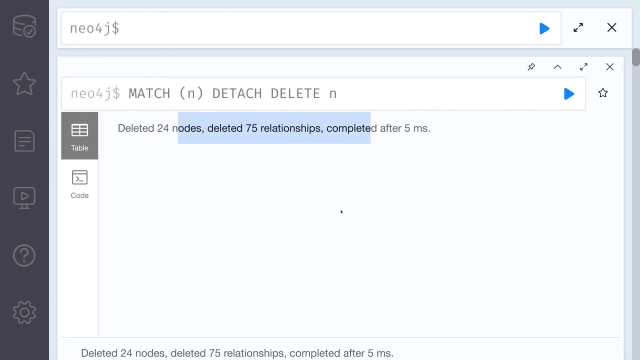 so execute that, And now we get 24 nodes deleted. Yes, We get 75 relationships deleted. And the reason why we did this is now we're going to start learning about how to create data and then, later on, we're going to learn how to update data. 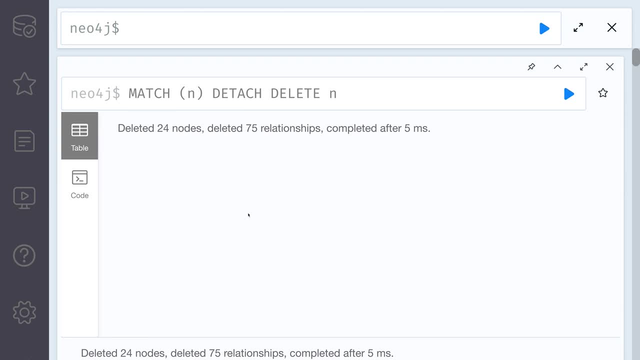 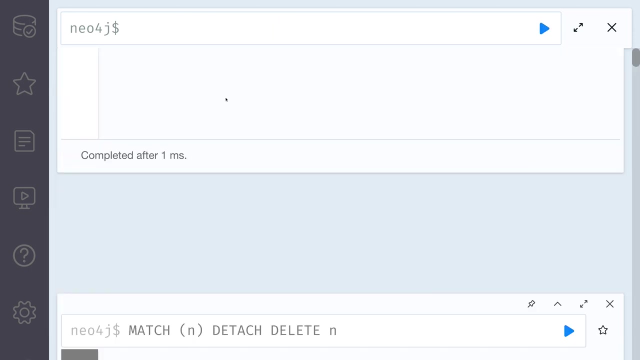 And so I want to just have a nice clean slate. Let's start adding back some of the data that we deleted, because right now, if we did a match and return and return and we're going to get nothing back because, again, we deleted absolutely everything. 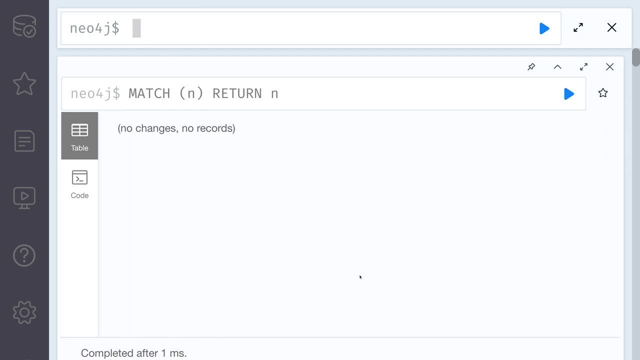 So the first thing that I want to do is what I want to do is create a node that is going to be representative of LeBron James. So we deleted everything. Let's just add a node that is going to be player, and it's going to be LeBron James. 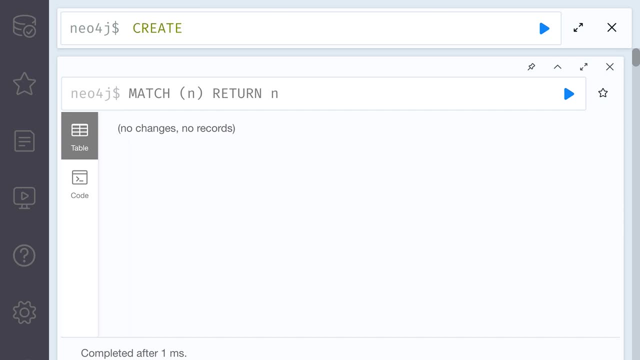 So let's go ahead and, in order to do this, we're going to utilize the, create a keyword, and then we're going to specify the node itself. So the first thing we can do is we can specify the label, so we can say that the label is. 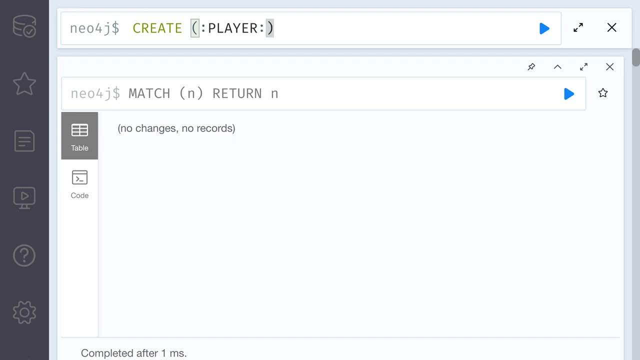 going to be player, But of course LeBron James. so we're going to say label player, and we can also specify multiple labels onto a node. This is something that we haven't seen before, but a node can have multiple labels. So over here we have a player, we have coach. 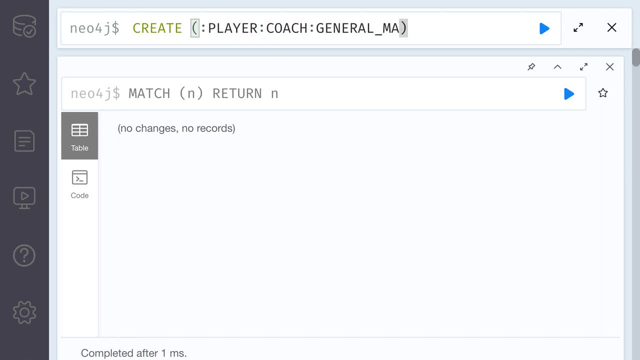 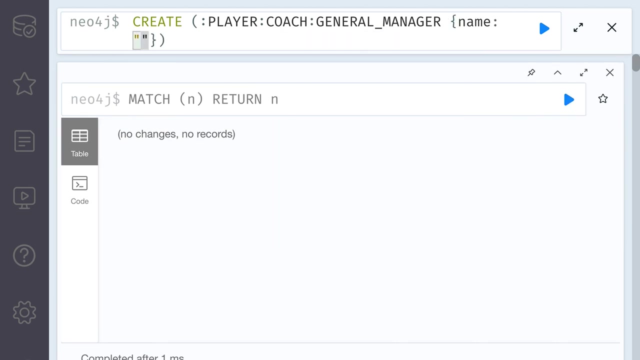 Let's also give him a general manager label. So general manager. Now, of course a node can have a label, but it can also have properties. So let's go over here and we can also specify the property properties with these curly braces, So we can say name, and then we can say LeBron James, LeBron James. and then we can also say: 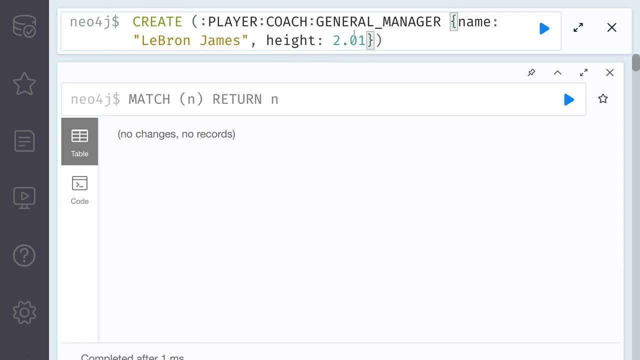 the height is, you know, two point zero one meters, and of course, we can continuously add more and more, But this is the only query that we need in order to create a brand new node. So what we can do here is we can actually get the query, assign it a variable name and 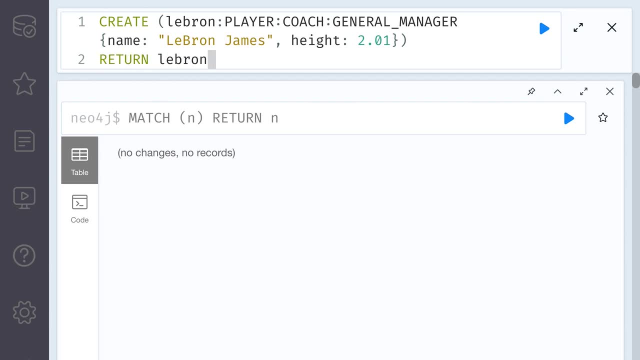 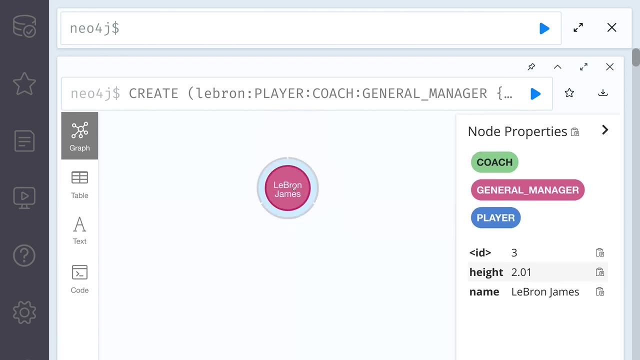 we can simply return it. so we can say: return LeBron. And if we were to execute this, you can see here that we get this LeBron node. he has these three labels And if you click on the properties, he has height as well as name. All right, 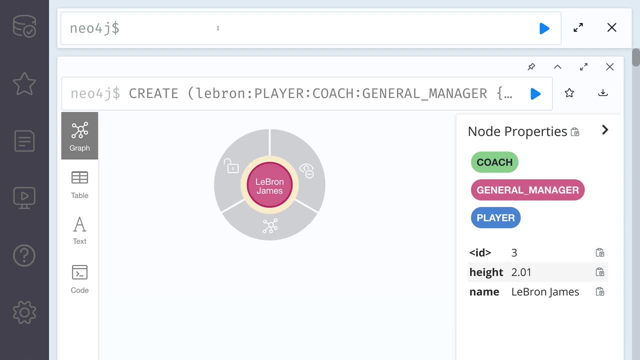 Cool. So let's actually just go ahead and let's delete this node, because now what we want to do is actually, you know what, let's just leave this node. and now what we want to do is we want to create a node as well as the relationship. 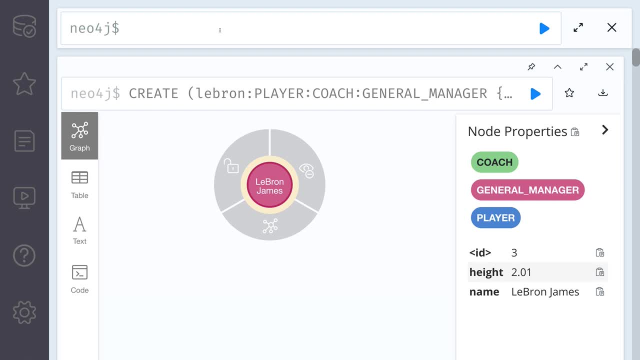 So let's create Anthony Davis And let's create a relationship as well to another node that we're also going to create, which is the Los Angeles Lakers. So, in order to do this, what we're going to do is specify, create and then, over here we're. 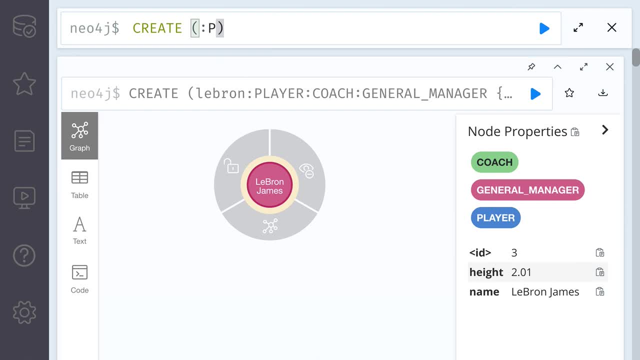 going to give Anthony the player tag or the player label, So we're going to say player and then, just like we did match, we're going to have our, our relationship And, of course, because this doesn't exist and we have the create keyword, we're going to 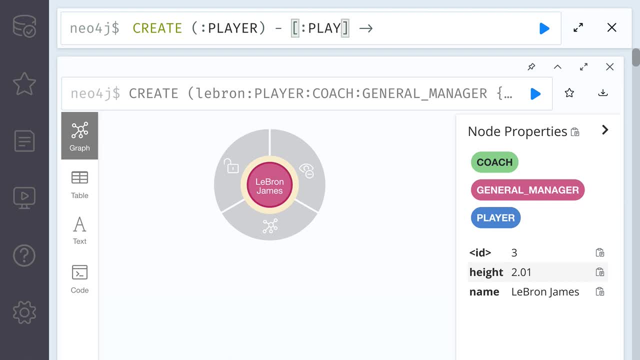 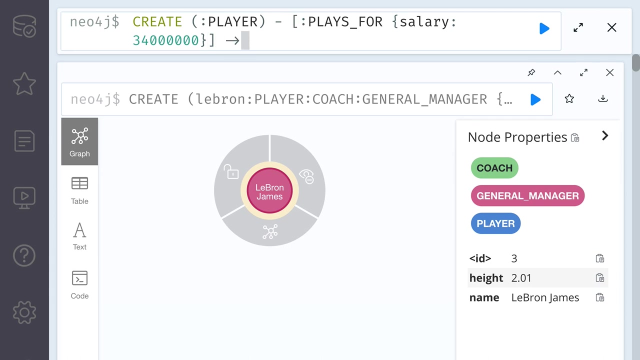 create it, And then over here we can say: simply place for, so, simply place for us. over here we can add that, and we can also add properties in as well. so we can say: salary of thirty four million dollars, thirty four million dollars. and then we can have another node that we 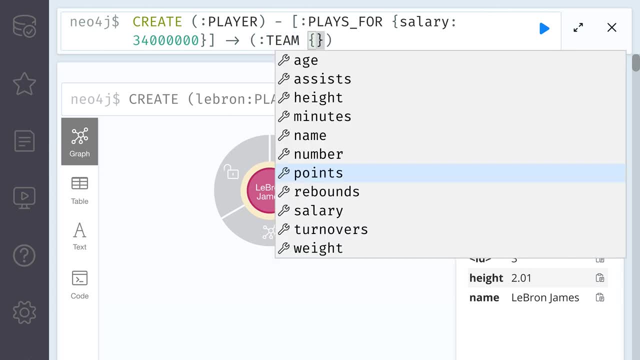 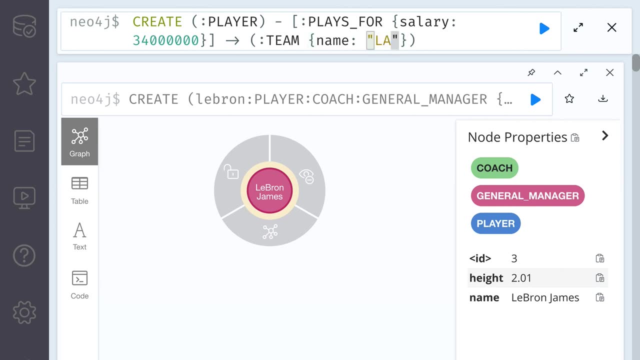 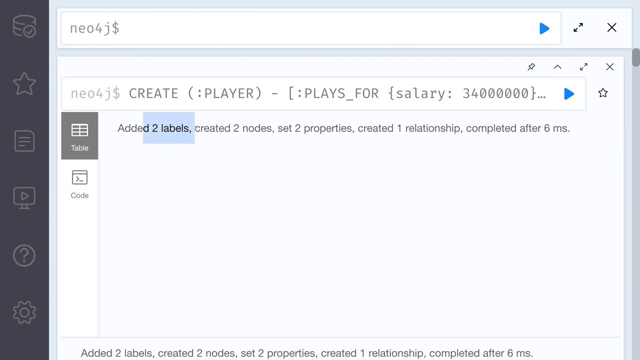 can create and this is going to be called team and we can give this the name, give it some properties name of let's give it LA Lakers. So if we were to execute this, this is going to pass. we have created two labels. we've created 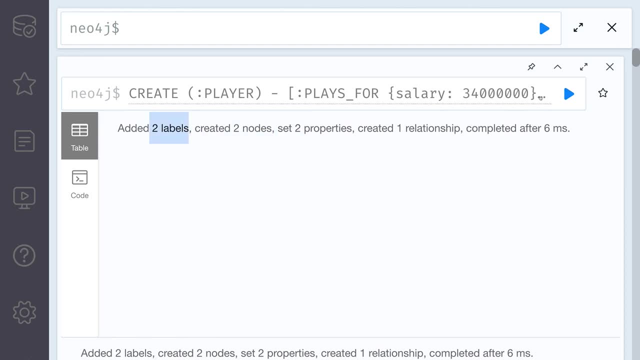 some nodes and everything. So the two labels are for the Los Angeles Lakers and for Anthony. The two nodes are again for the team and the player, and then we have some other properties. So now what we can do is very simply do match and return and to get all of the nodes as 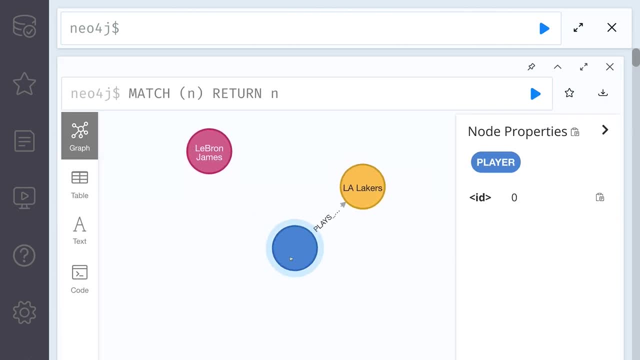 well as their relationships, and we should see this Now. The only issue that we're facing- And that's actually my bad- is I forgot to give the this particular node the property of Anthony Davis, but I hope that's kind of clear. that was my my apologies. I completely 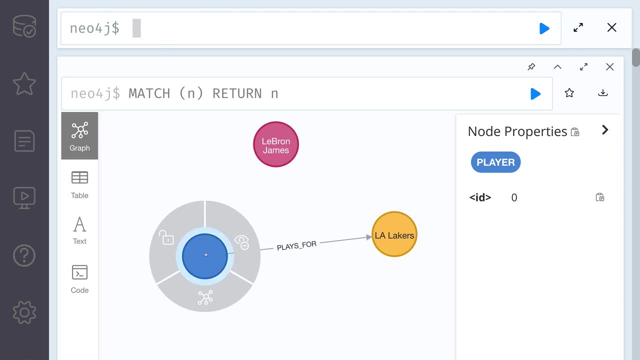 forgot about that. So let's just assume that I did this. remember the same way we do it, the same way that I showed you with the curly braces. But now let's say we have existing data, so we have LeBron James and what I want to do. 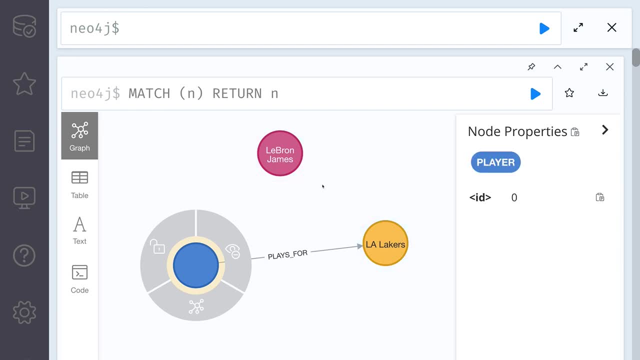 is, I want to add a relationship Between these two nodes. So I don't want to completely delete the Lakers and LeBron James and create them all at once. I already have the relationship and I just already have the nodes and I want to create the relationship. 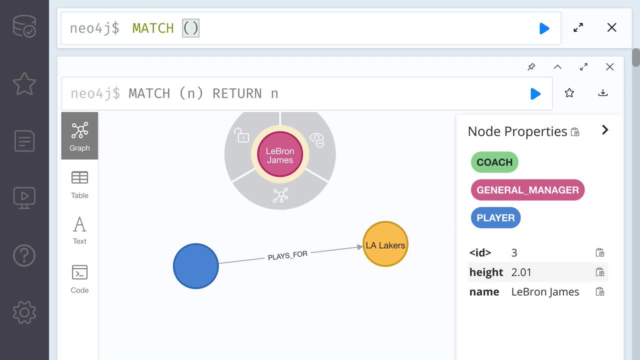 So, in order to do this, all we need to do is very simply get the node that is representative of LeBron James, So we can say this is going to be. We can just say simply: well, again he's everything. so we could just say: player, we can call this. 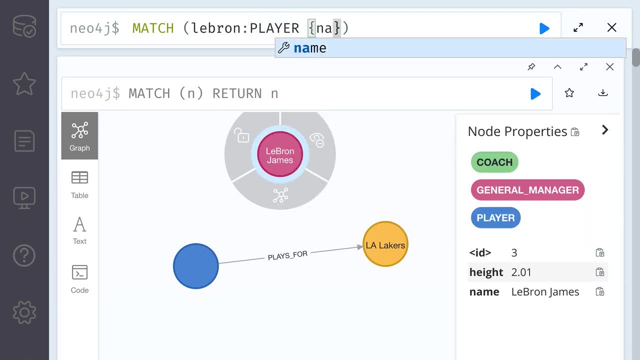 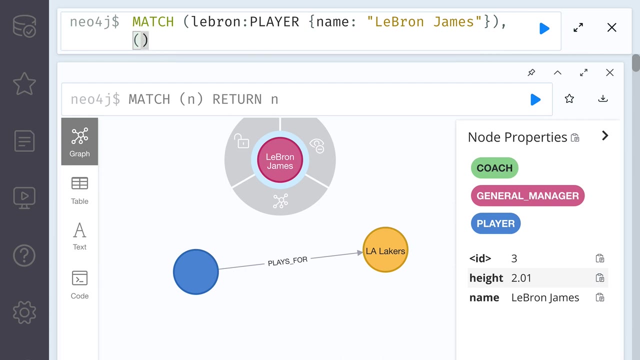 LeBron. And then we can Say: We can say that the name is going to be LeBron James. And now we also need to get the team the Lakers. so we can do comma. we can have another node here and we can say: well, the Lakers. 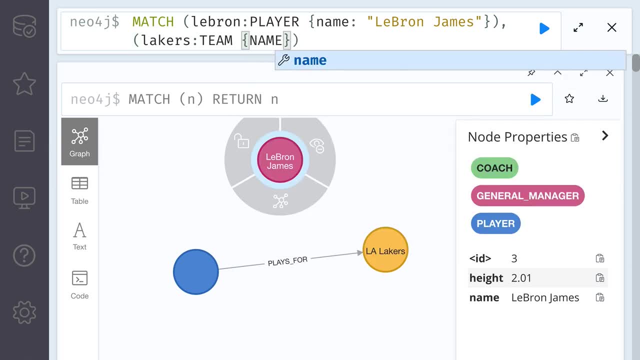 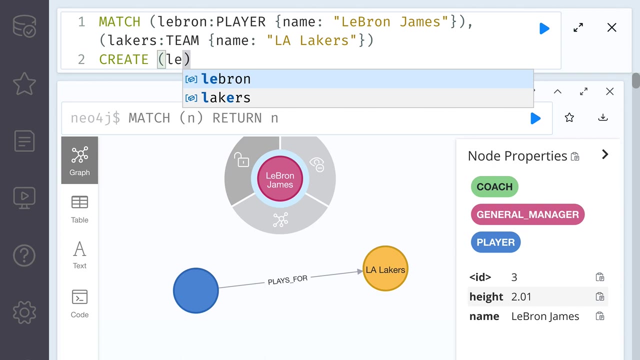 Which is a team, and over here we can say that the name Is the Lakers, so L a Lakers. So now what we can do Is create the relationship between the already existing LeBron node, so we can say LeBron, And then what we can do here is say: hey, we want a relationship. 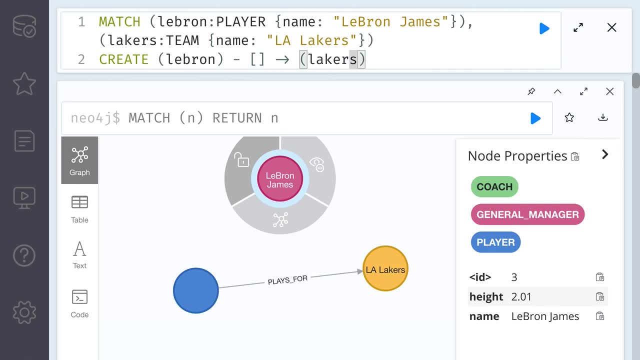 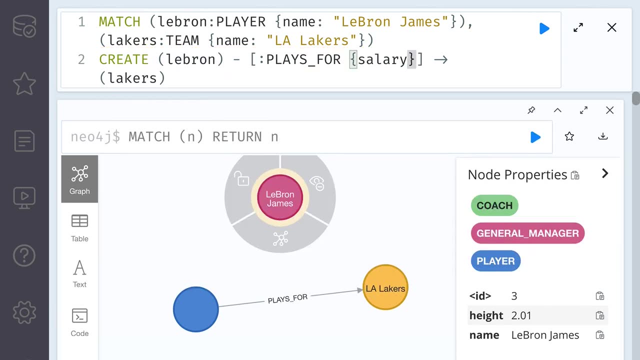 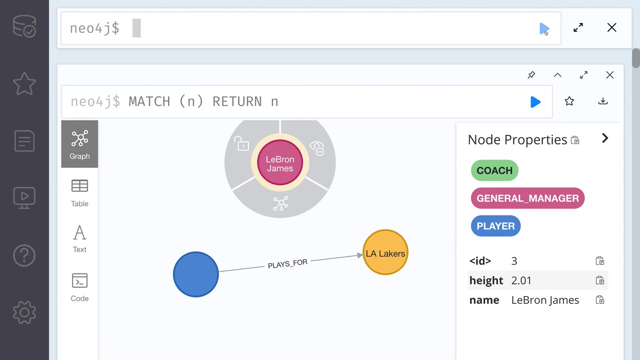 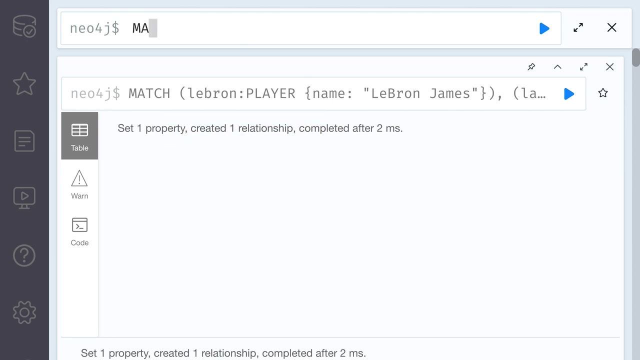 Between the already existing LeBron node and the already existing Lakers node, and we want a place for relationship and we want to give this a salary of 40 million. think that's 40 million. Yes, and now, if you were to execute this, It has worked. so we didn't create any new nodes. all we did was create a relationship. 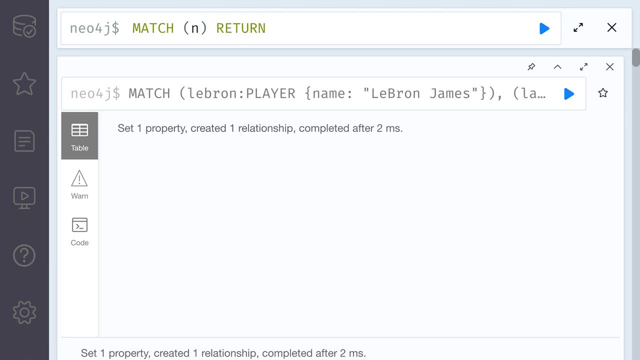 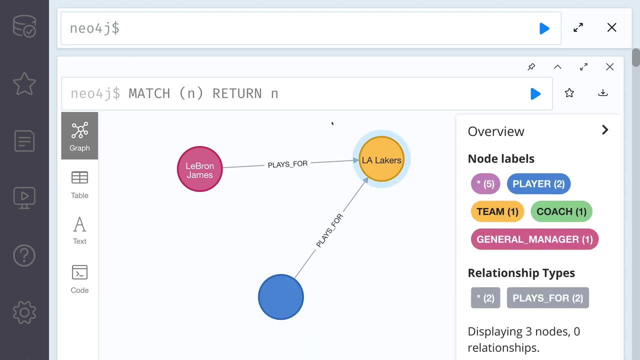 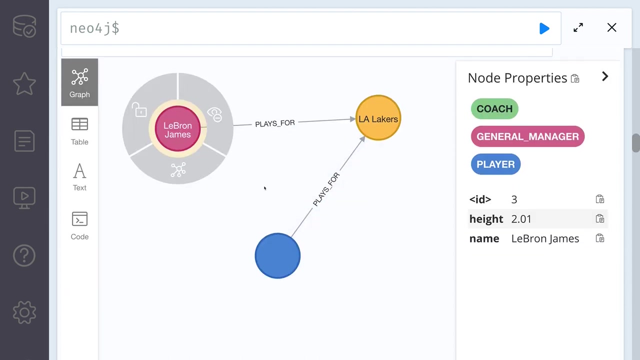 So now, if we did match and return and And execute this, You can see that we have that relationship and that's really all we need to know about. well, Creating date. the last thing that we are going to learn about is how we can update our nodes. 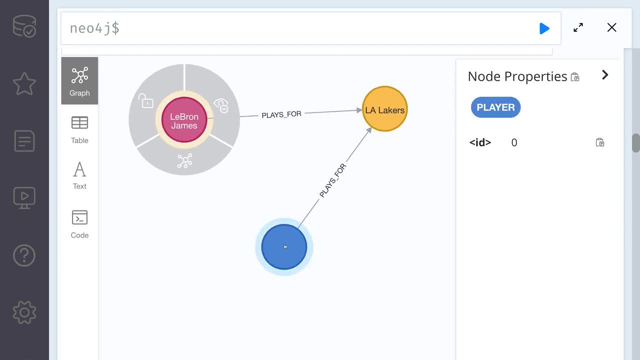 And relationship. Now this right here, we want to add the name of Anthony Davis, because we missed us. now, of course, we don't want to completely delete the node and then re add it. We just want to update it. So, in order to update it, the first thing that we need to do is find that specific node. 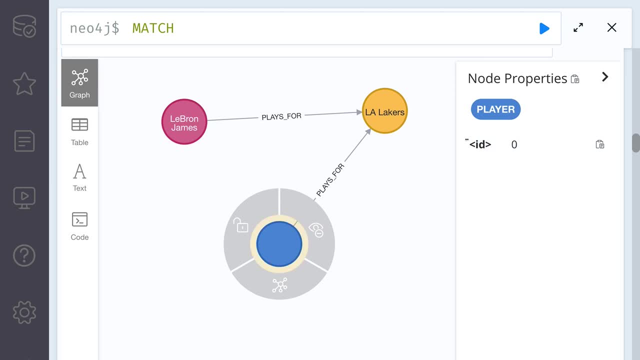 Now this node right here has no specific attributes but the ID. So we're going to have to query for this node by the ID. Now you might be thinking, OK, well, that's relatively easy. what we can say here is Anthony, or we can call this whatever. 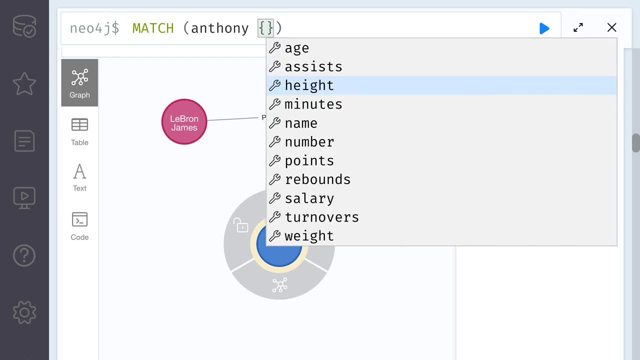 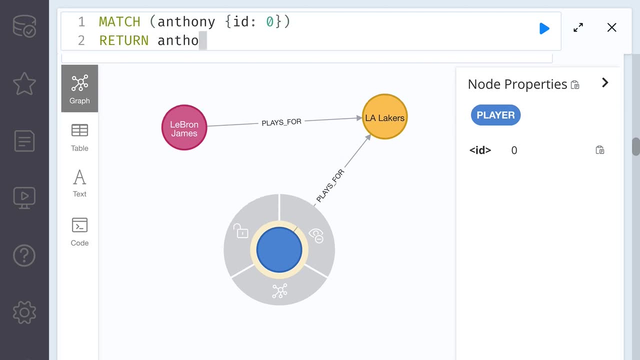 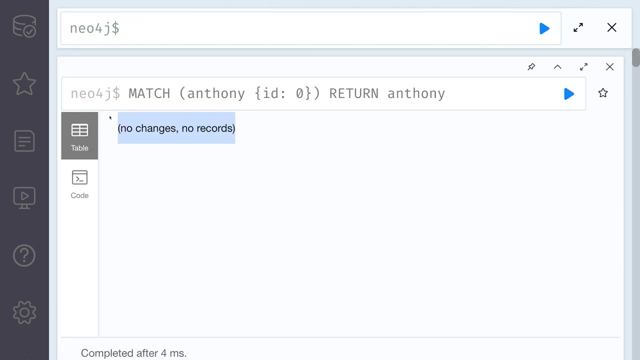 node it is that we want, and then we can say that we want the ID of zero in this case, So zero in this case. However, if I went ahead and I returned Anthony, what's going to happen is I scroll all the way up. There's nothing there. 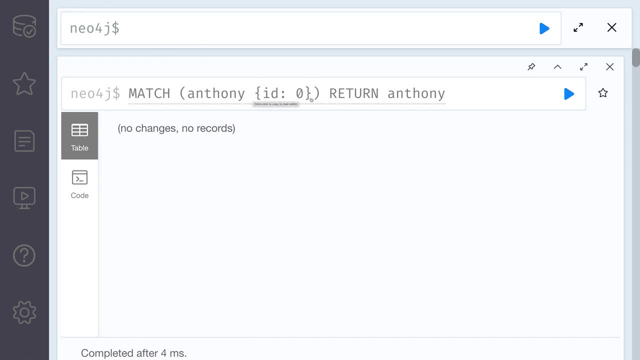 So the way that we actually query using an ID is going to be a little bit different than the way That we would Query using other properties. So, in order to query using an ID, and this is only using an ID, This is just the only difference. we're going to say Anthony. we're going to say Anthony. 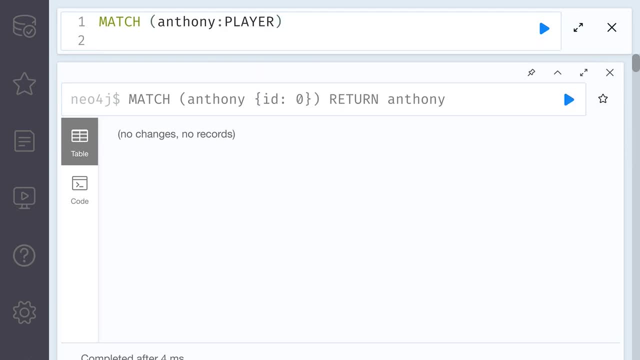 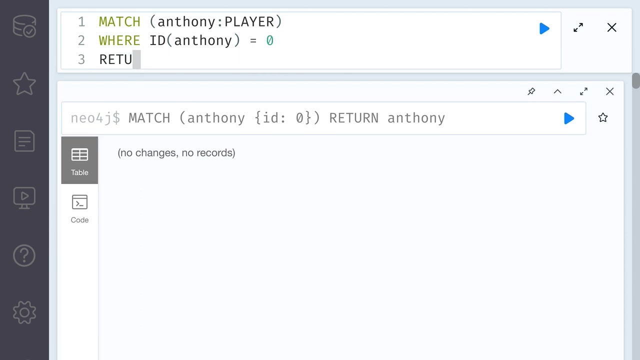 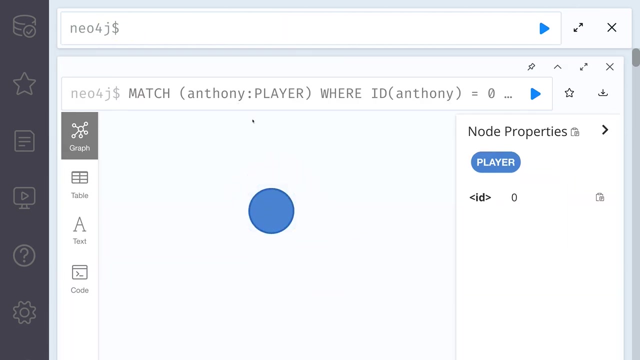 is also a player, and then what we're going to say is: where the ID of Anthony, So the ID of the Anthony node, is equal to- and I think it was zero, and then we can very simply just return Anthony, So Anthony, So let's go ahead and return that, and now we get Anthony. 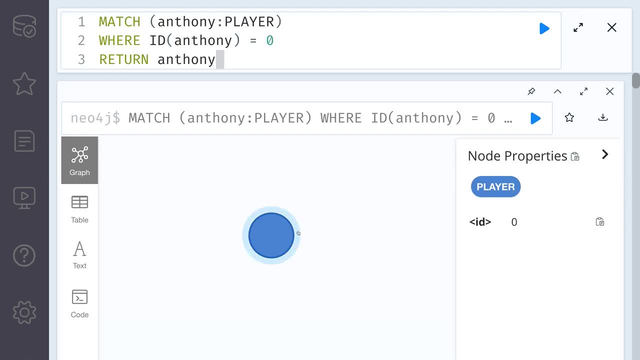 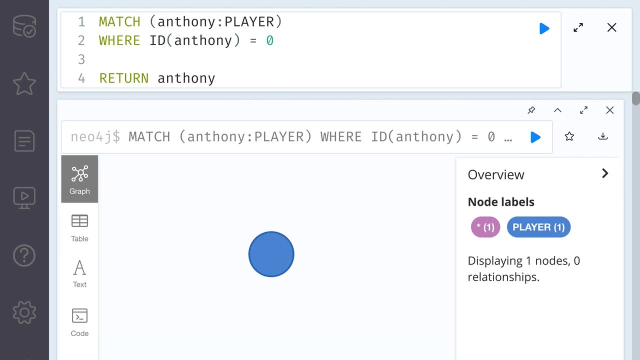 So what I want to do is I want to set a property in here called name Anthony Davis. So, in order to do this, what we're going to do is, right after the where clause, we're going to use another keyword called sect, and then in here we're going to get our node, and then 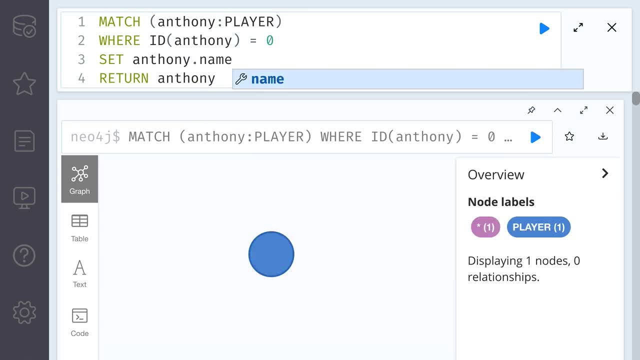 we're going to do dots and then whatever we want to say, So Anthony thought name And that's going to be equal to Anthony Davis, and then we're going to return Anthony. So if you were to actually execute this, you can see that now we actually created an updated 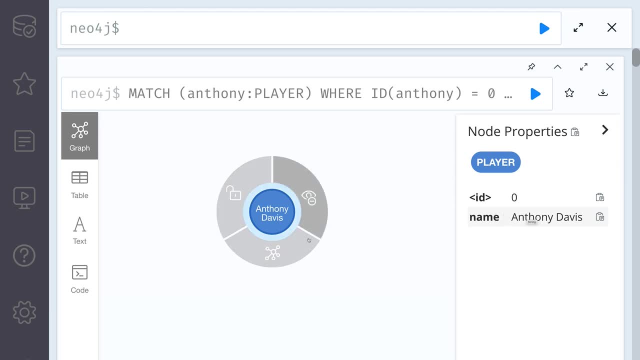 our node by adding this particular property. So of course we can add properties, we can also update properties. So let's actually kind of do things on the LeBron- LeBron node. So let's say: here LeBron, we're going to say LeBron is a player, and then we're going to 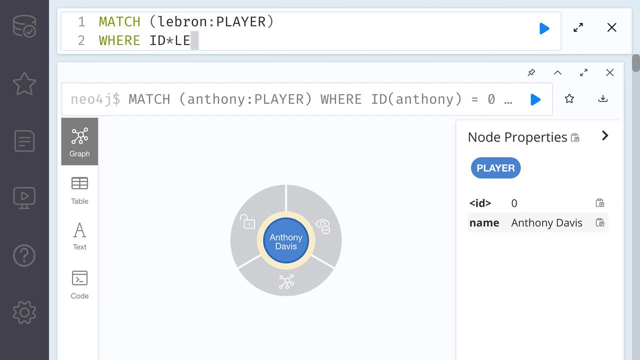 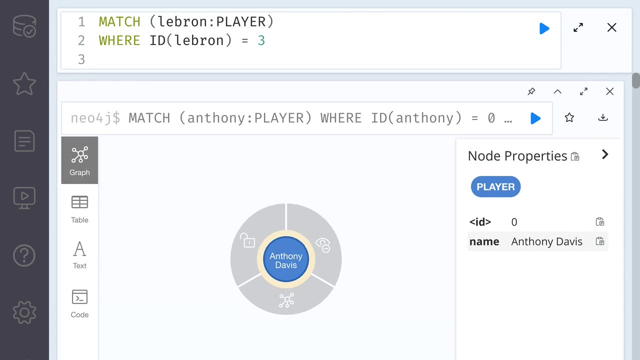 say, let's just use the where as well. So we're going to say where the LeBron node has An ID. LeBron node has an ID that's equal to three. That's what it was. And then in here, what we're going to do is we are going to update LeBron's height. 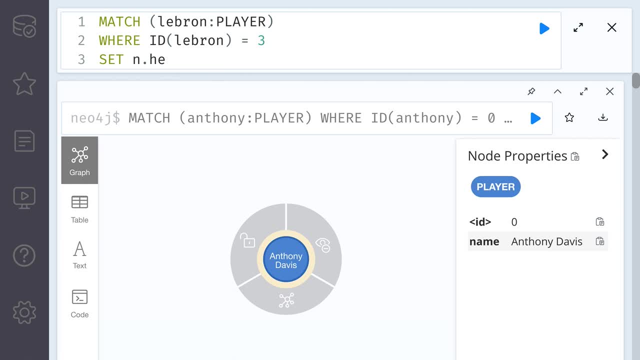 So we're going to update LeBron's height to be just a little bit taller. Maybe we we miscalculated LeBron's height. We're going to update it to 0.0 or 2.0, to it will- before it was 0.01- and what we can also do. 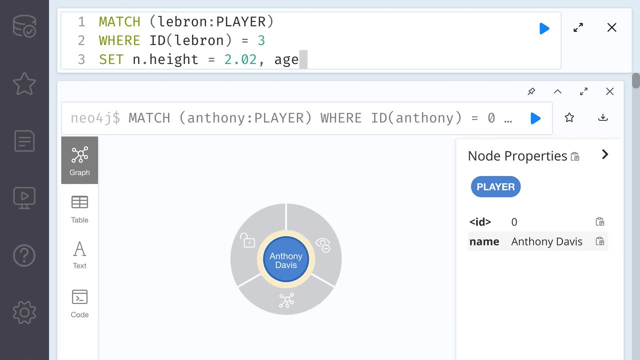 Is, we can also add another property if you want to. So we can update a property and add another property at the same time by simply doing- and we should call this LeBron, not an LeBron- and we can do that by having a comma and then have LeBron dot age, and I think LeBron is 36 and we can return LeBron the LeBron node. 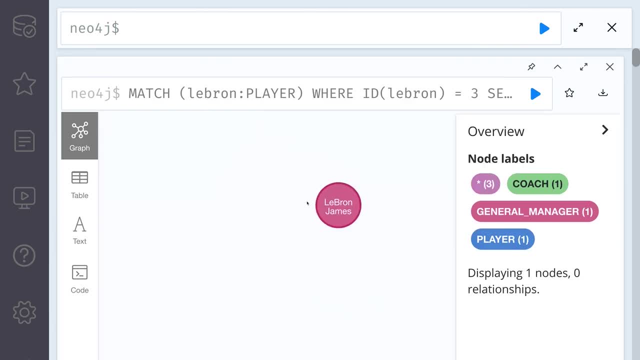 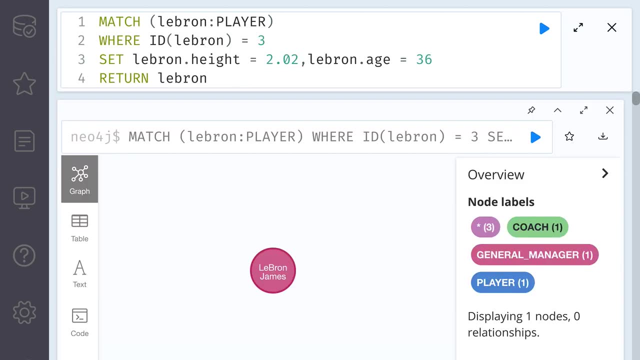 So if we were to execute this, there we go. Everything seems all fine and dandy. Now, of course, we can also Update the labels, So let's actually go ahead and we're going to re-execute this query, But instead, this time, I'm going to add another label right now. 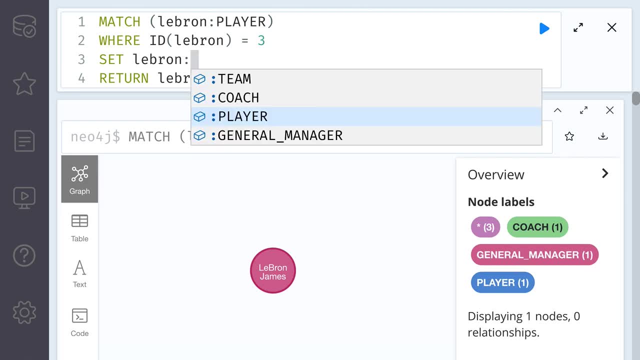 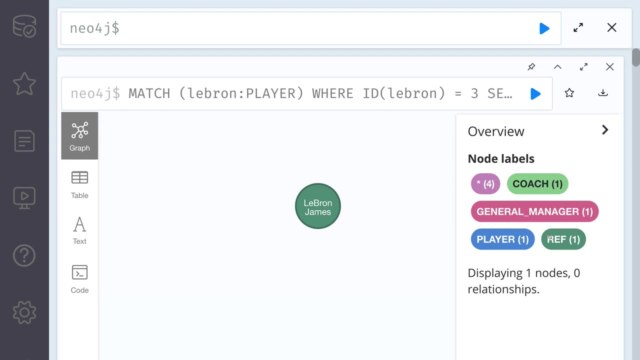 LeBron has the coach, general manager and player label. Let's also give him a ref label, And so all we have to do is say set, and then LeBron, and then whatever that label is, So call in that label. So now, if you were to execute this, you can see and how he has three different labels. 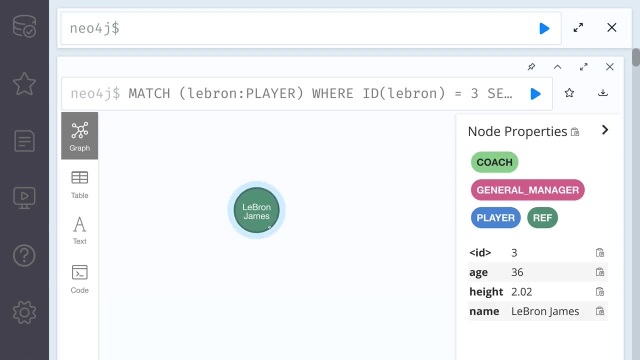 All right, isn't that terrific? So we can, of course, do the exact same thing with the relationships. So what if we have remember that play for relationship has a salary and we want to update that salary to be, you know, a little bit larger than what it was before? 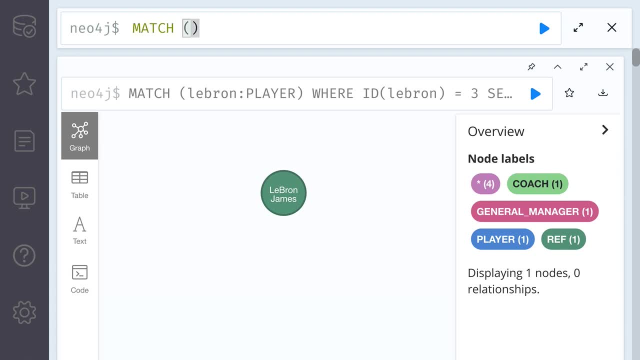 So just to quickly show you, we're going to have a match and let's say we want to update LeBron salaries. We're going to say LeBron where the name is LeBron James, and then what we want to do is we want to Get the salary. 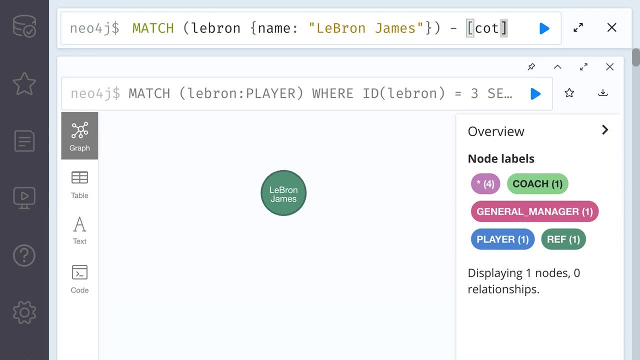 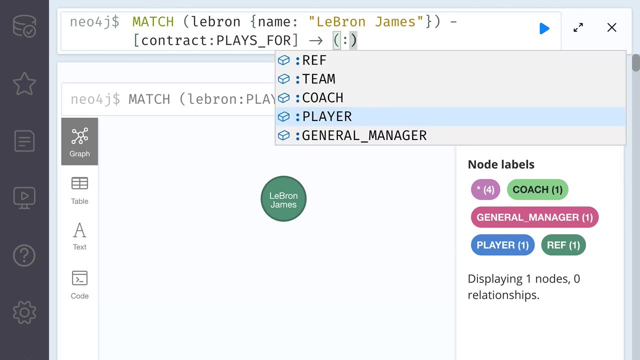 So we want to get the salary, so we can say contract here And this is going to be placed for, and then over here we can specify that this is a team. We don't really need to get the team, but we want it, We will. we will just say that it is a team. so we need- we don't need- a variable here. 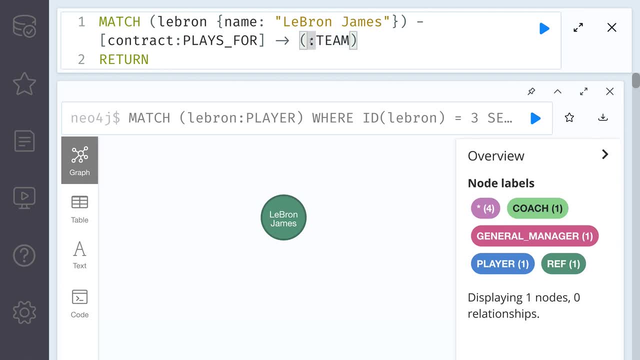 And then here we can simply just say: actually, you know what, Let's just return the team itself so we can also see the relationship between LeBron and the team. So we're going to say LeBron And then team. So if we were to do this, 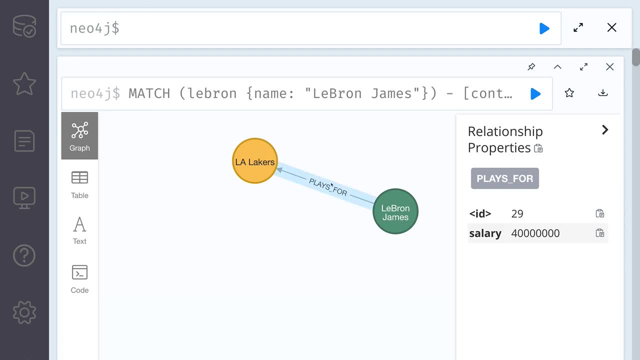 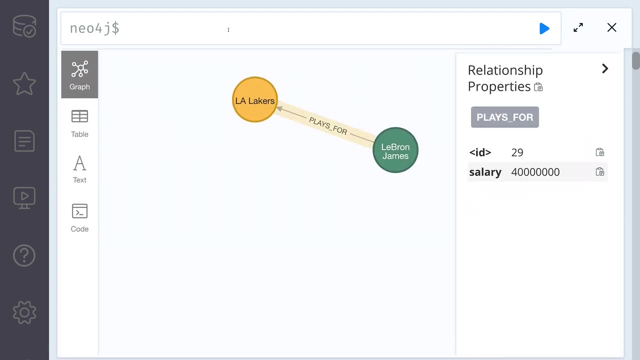 we were to get this and let's say, what I wanted to do is I wanted to update this. So I want to update this label so that the salary is maybe 60 million a year, And this is actually very easy. It's very similar to what we've done before.